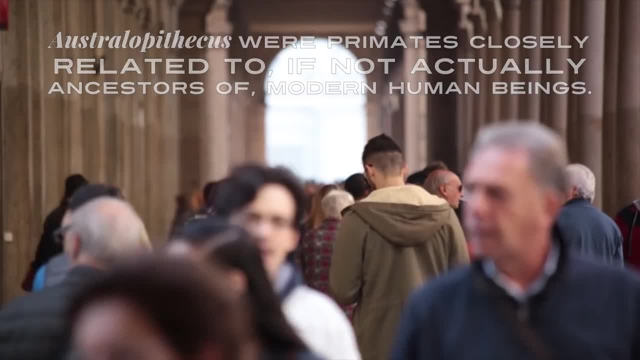 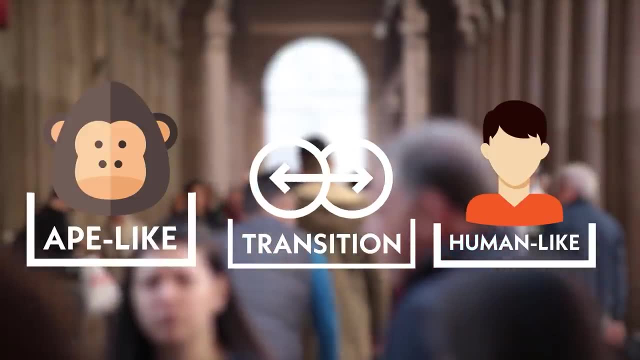 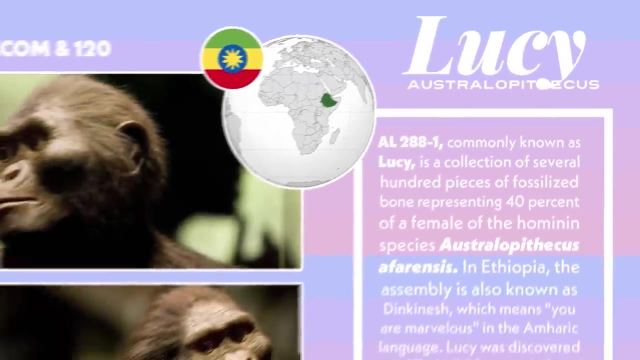 of modern human beings. For this reason, it is a crucial evolutionary link between non-human ape-like creatures and early human species. It is perhaps one of the richest paleoanthropological finds, with fossils like Lucy yielding significant insights into our evolutionary past. Species are numerous and include Australopithecus'. 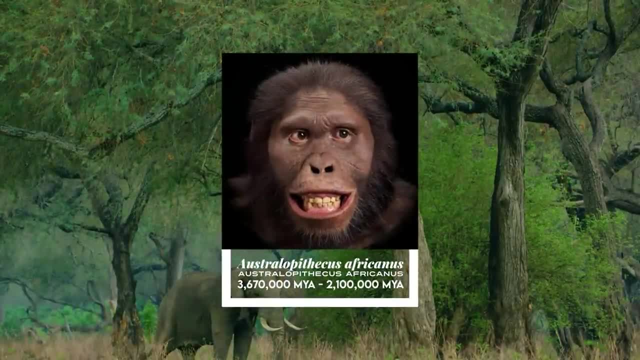 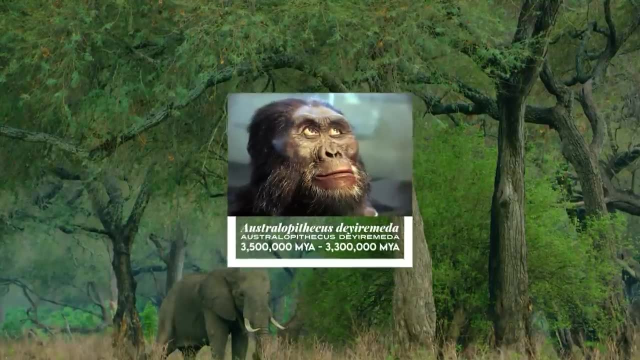 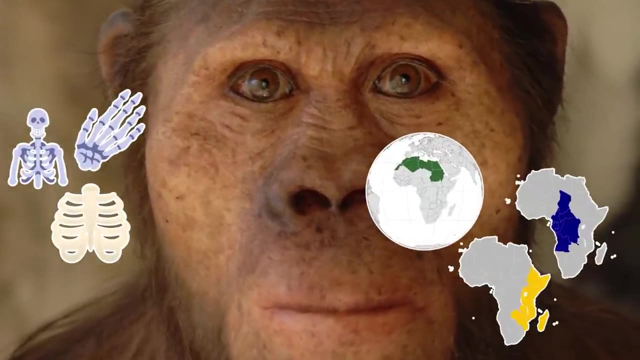 gari Africanus, Sediba Afarensis, Anamensis Barrel-Ghazali and Digeramida. Australopithecus is known from a series of fossils found in numerous sites in eastern, north-central and southern Africa, also known as the Cradle of Humankind For the longest. 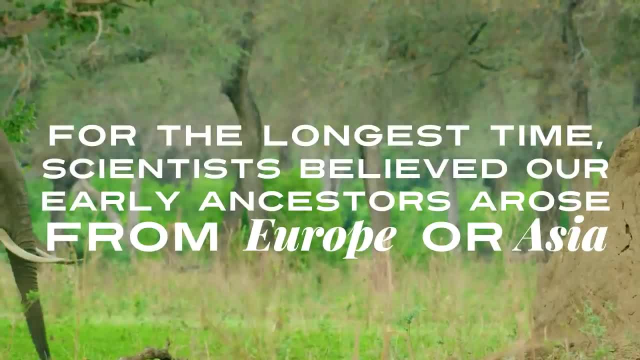 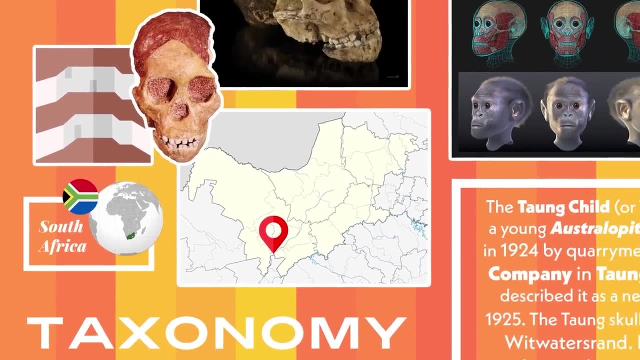 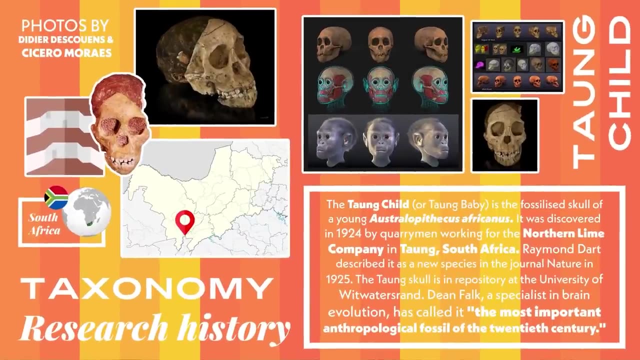 time, scientists believed our early ancestors arose from Europe or Asia. Yet in 1924, a fossil discovery in South Africa revolutionized the perception of early human evolution, known as the Tongue Child, which we will get to later in the video. 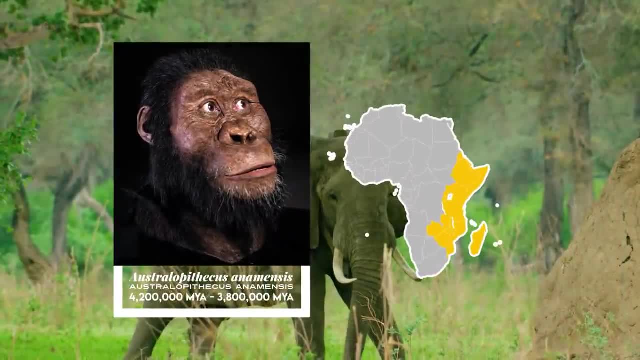 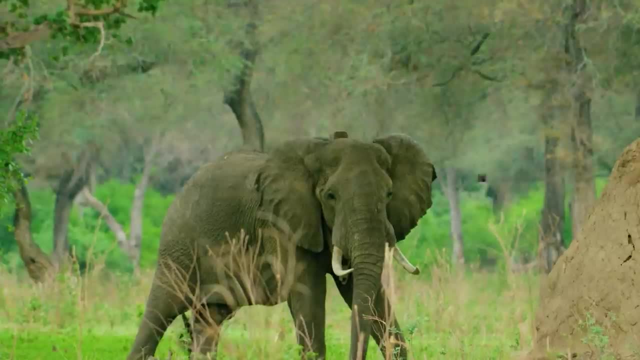 Australopithecus anamensis existed in eastern Africa around 4.2 million years ago, possessing a smaller cranial capacity than other australopithecines. Australopithecus fossils became more widely dispersed throughout eastern and southern Africa. 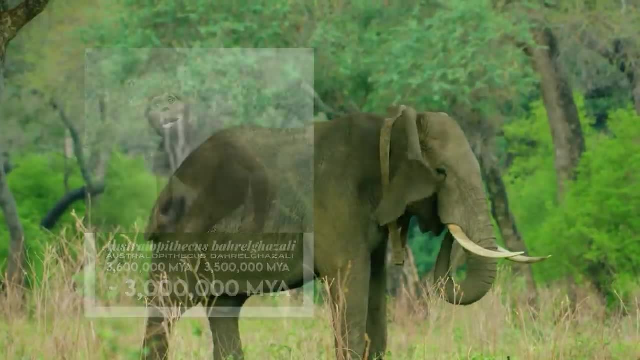 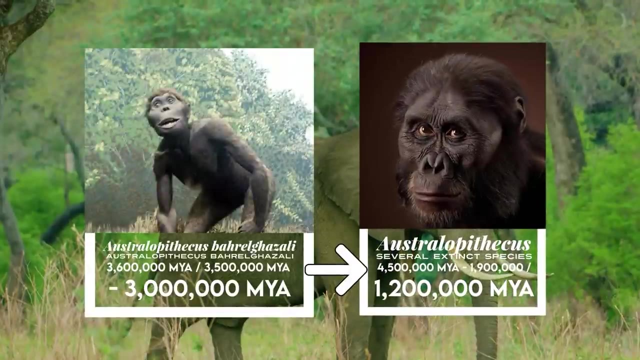 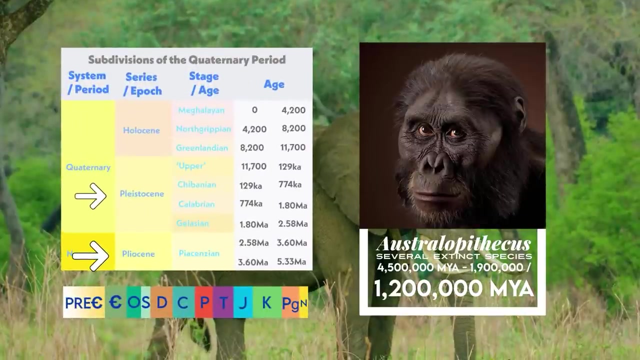 Australopithecus Fossil- Australopithecus Barrel-Ghazali, indicating the genus, was much more widespread than the fossil records suggest, before eventually becoming extinct 1.9 million years ago, or 1.2 million to 600,000 years ago, if Paranthropus is included, during the Pliocene and Pleistocene epochs. 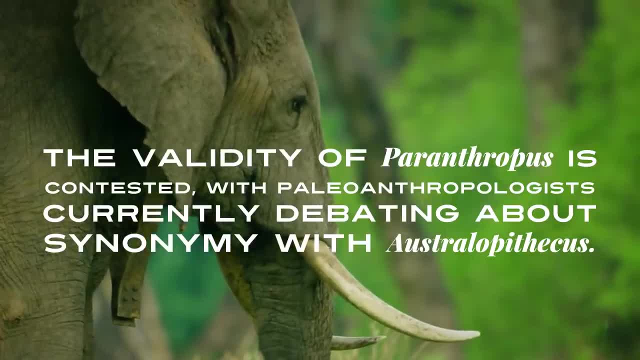 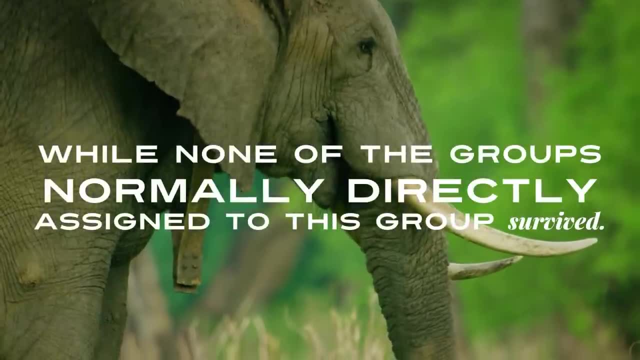 The validity of Paranthropus is contested, with paleoanthropologists currently debating about synonymy with Australopithecus. While none of the groups normally directly assigned to this group survived, including the subspecies, Australopithecus gave rise to living descendants. 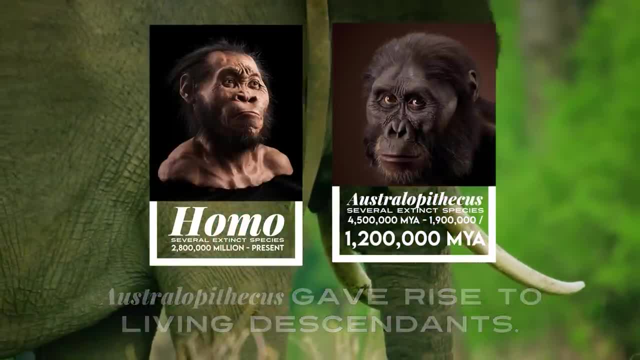 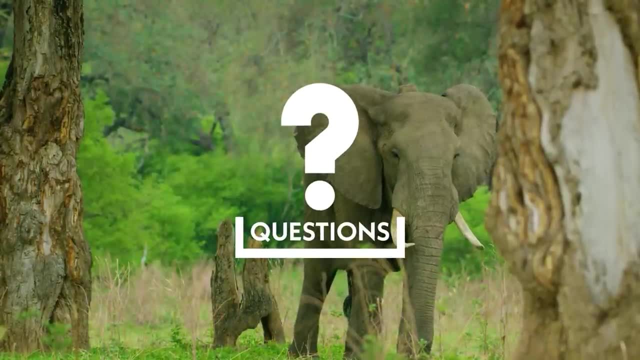 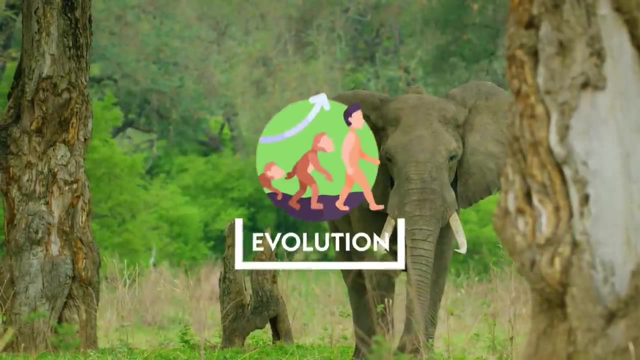 humans or Homo, which emerged from an Australopithecus species sometime between 3 and 2 million years ago. One of the greatest mysteries in paleoanthropology might be the exact species from which early Homo arose, whose discovery could notably change our view of early human evolution. 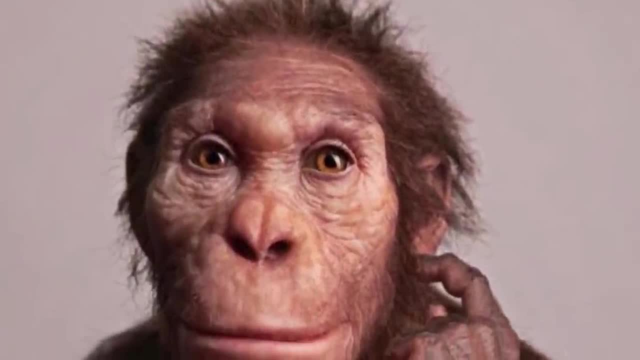 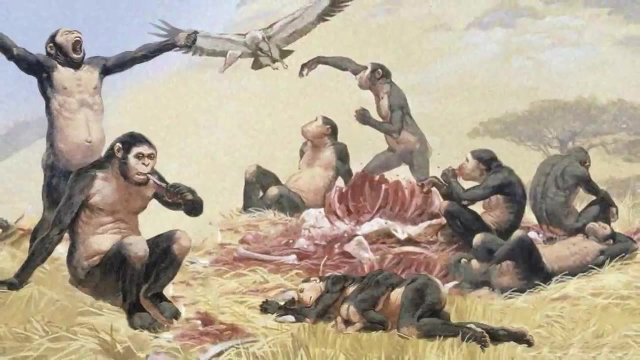 As evident in the fossils of Australopithecus, members of this group bore a huge amount of life, including a combination of human and ape-like traits. This is also present in later early hominids like Homo habilis, creating taxonomic inconsistency. 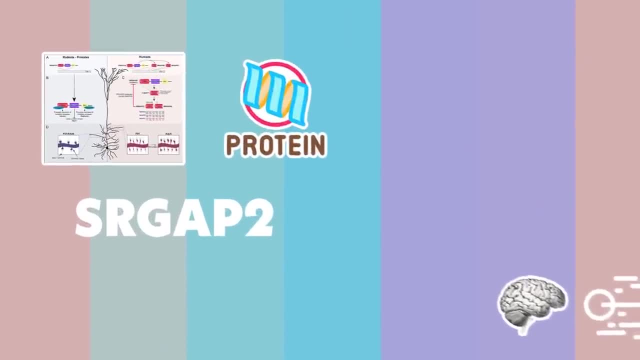 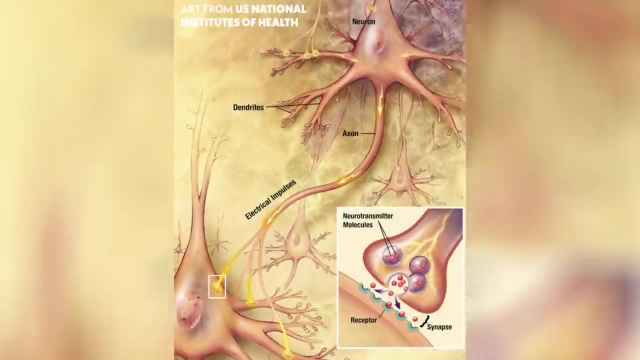 Australopithecus possessed two of three duplicate genes derived from S r Gap II, a mammalian protein that plays a critical role in synaptic development, brain mass and number of cortical neurons, roughly 3.4 and 2.4 million years ago, including S r Gap IIb and S r GapB. 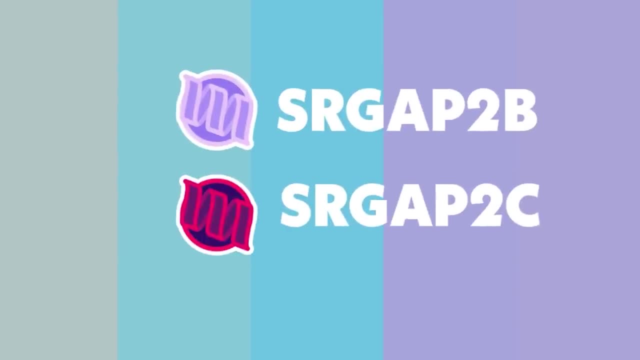 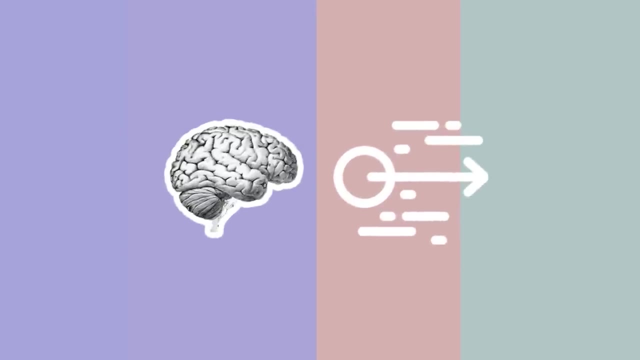 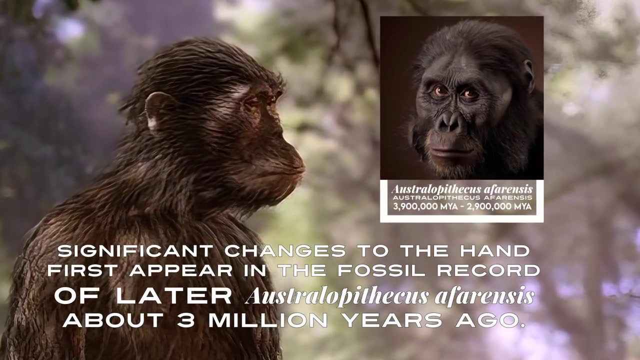 including sRGaP2b and sRGaP2c, the second of which contributed to the increase in number and migration of neurons in the human brain. Significant changes to the hand first appear in the fossil record of later Australopithecus afarensis about 3 million years ago, with the 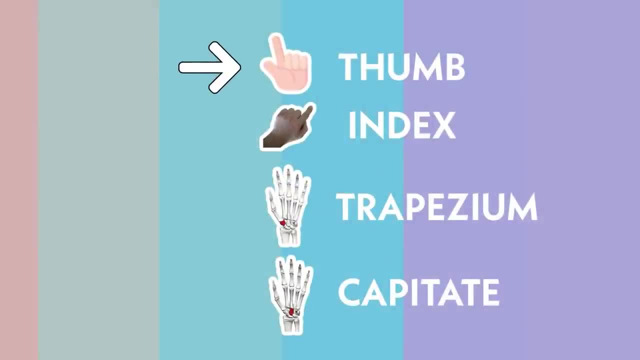 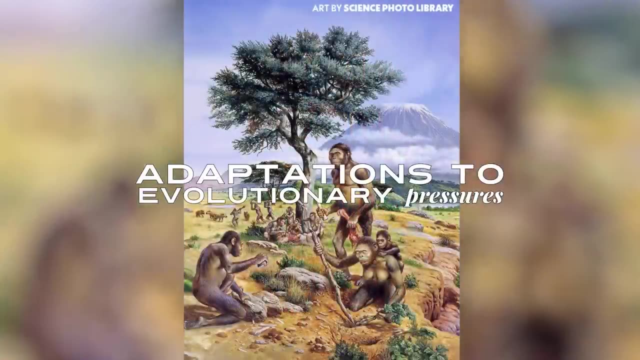 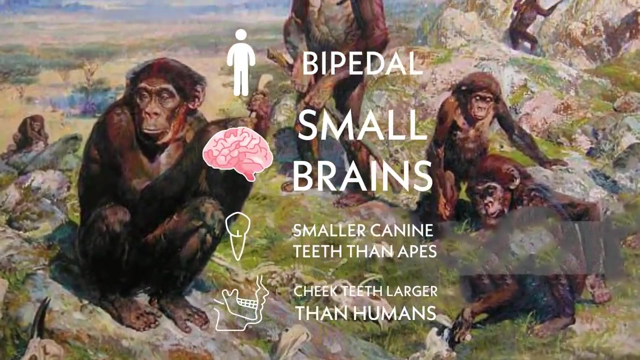 fingers, shortened relative to the thumb, and changes to the joints between hand bones like the index finger, the trapezium and capetid. These changes highlight adaptations to evolutionary pressures. They were similar to modern humans in that they were bipedal or walking on two legs. 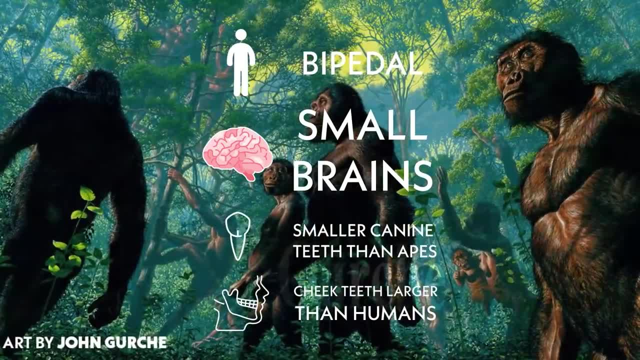 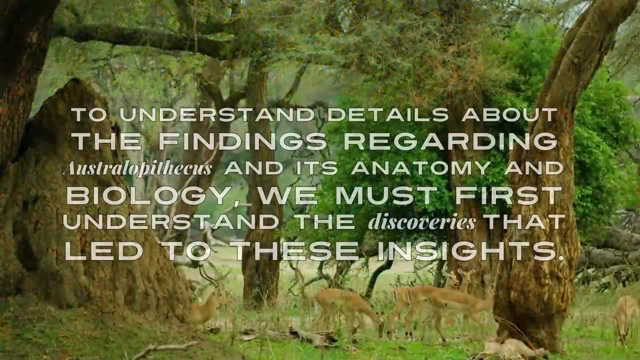 but like apes, they had small brains, with their canine teeth being smaller than those found in apes and their cheek teeth larger than those of modern humans. To understand details about the findings regarding Australopithecus and its anatomy and biology, please refer to the 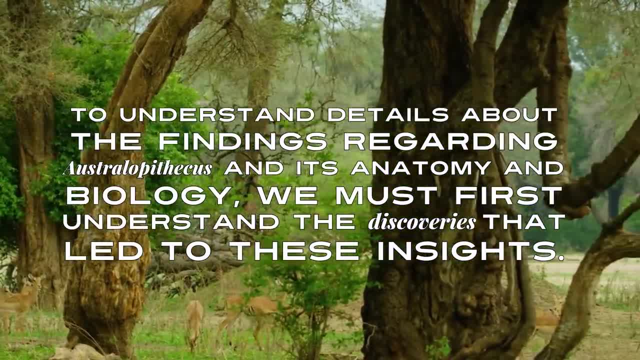 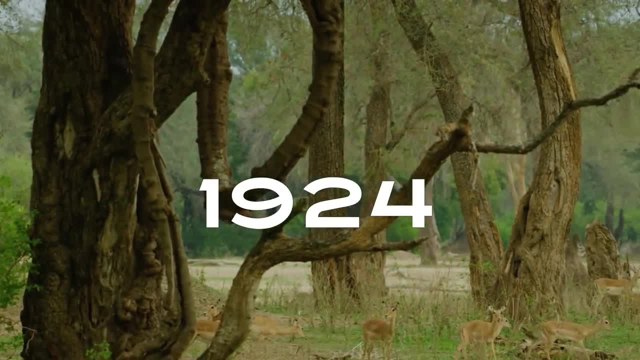 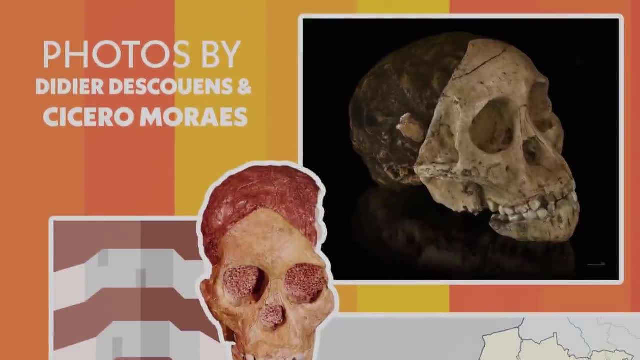 link in the description. We must first understand the discoveries that led to these insights. The year was 1924.. Workers at Taung, South Africa, were working at a lime quarry when they stumbled on a remarkable discovery: the first Australopithecus specimen. the type specimen. 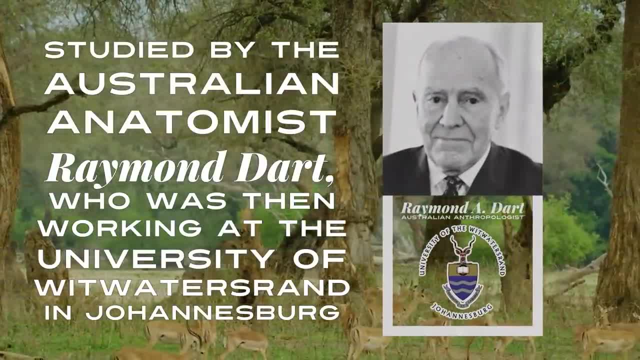 which was studied by Australian anatomist Raymond Dart, who was then working at the University of Woodwatersrand in Johannesburg. The first Australopithecus specimen was studied by Australian anatomist Raymond Dart, who was then working at the University of Woodwatersrand in Johannesburg. The fossil skull was from a 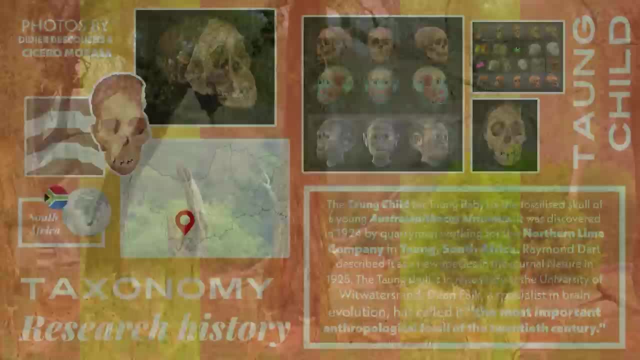 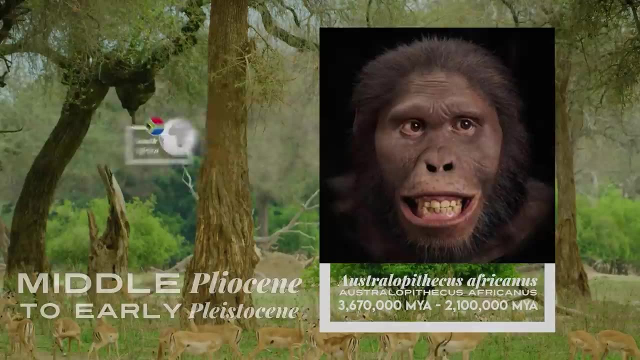 three-year-old bipedal primate that he named Australopithecus africanus, an Australopithecine that lived from 3.67 to 2 million years ago in the Middle Pliocene to Early Pleistocene of South Africa, and the first early hominin found. 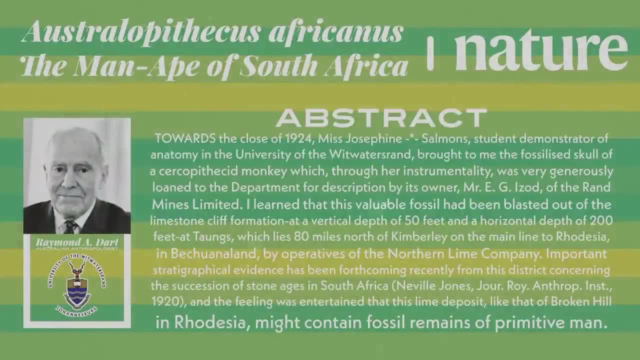 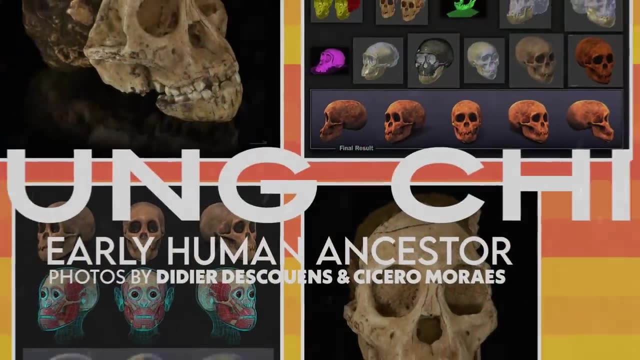 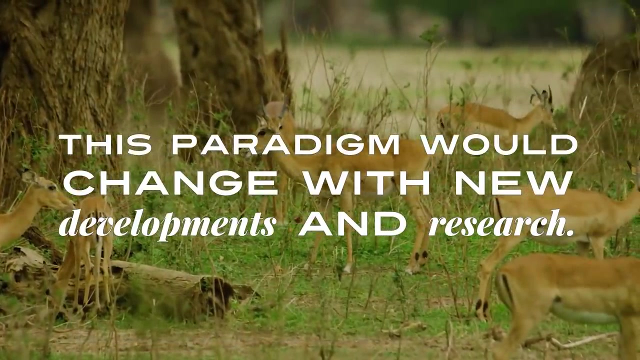 The first report was published in the journal Nature in February 1925.. Dart realized that the fossil had a number of humanoid features and consequently he came to the conclusion that it was an early human ancestor. This paradigm would change with new developments in research. Later, Scottish paleontologists Robert Broome and Dart set out to search for. 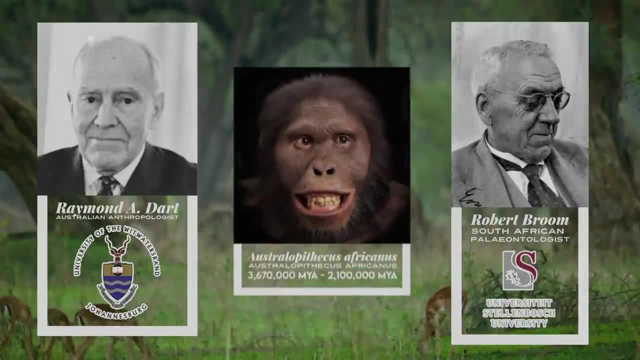 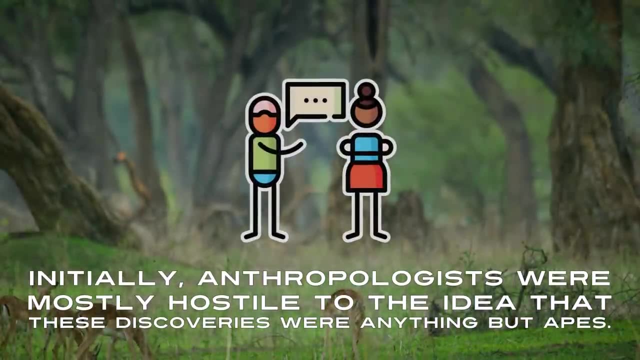 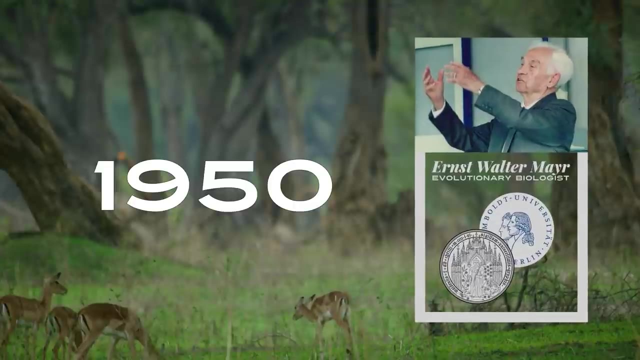 more early hominin specimens and several more Australopithecus africanus remains from numerous sites. Initially, anthropologists were mostly hostile to the idea that these discoveries were anything but apes, though this changed during the late 1940s. In 1950,, evolutionary 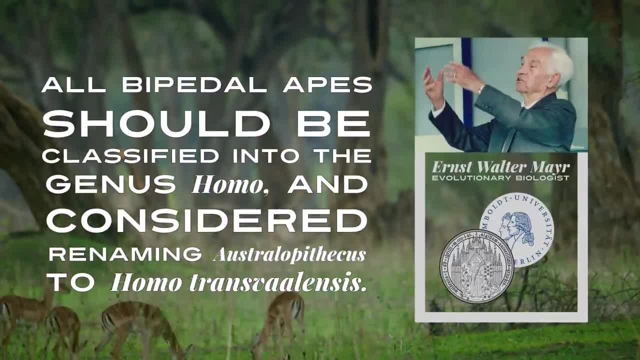 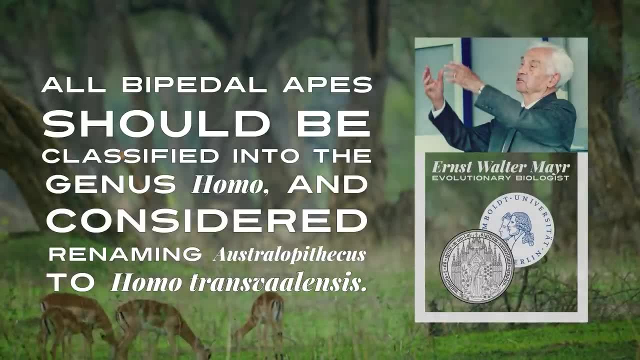 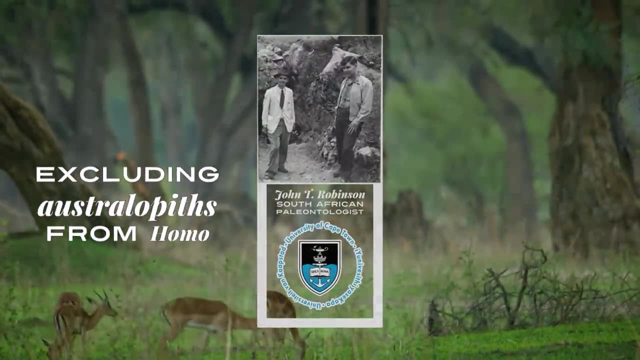 biologist Ernst Walter Mayer stated that all bipedal apes should be classified into the genus Homo and considered renaming Australopithecus to Homo transvalensis. Nonetheless, the contrary view taken by Robinson in 1954, excluding Australopiths from Homo, became the more popular and prevalent. 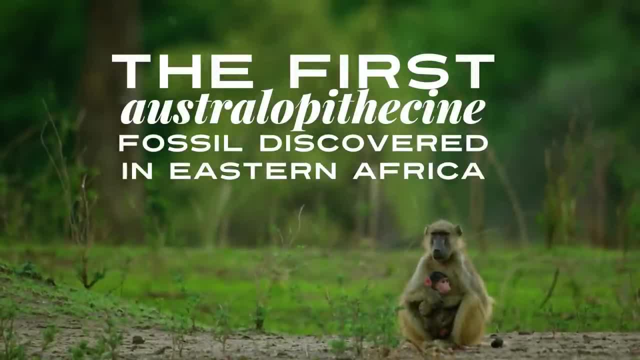 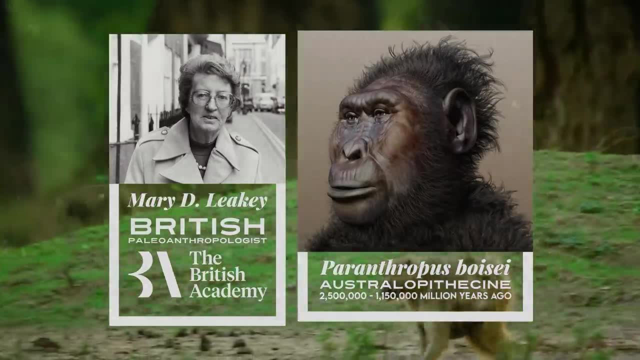 view. The first Australopithecine fossil discovered in Eastern Africa was an Australopithecus boisei skull excavated by renowned paleoanthropologist Mary Lee. The first Australopithecine excavated Leakey in 1959 in Olduvai Gorge, Tanzania. Since then the Leakey family has 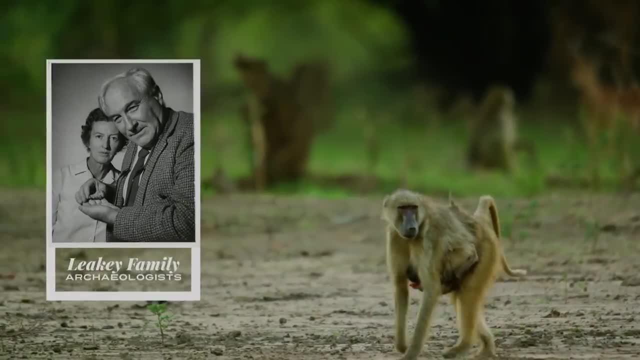 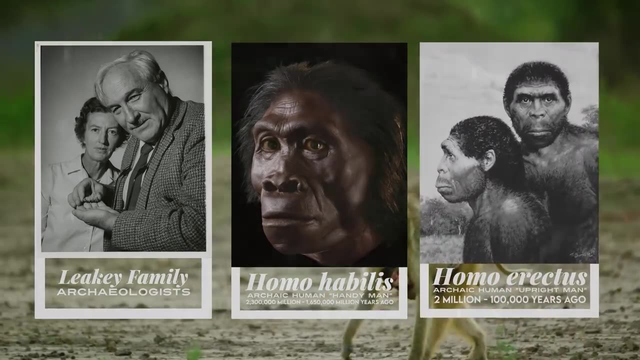 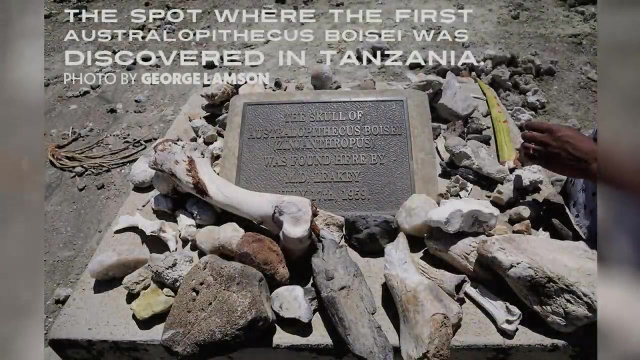 continued to excavate the gorge, uncovering further evidence for Australopithecines, as well as for Homo habilis, or the handyman, and Homo erectus, or the upright man. The scientific community took 20 more years to widely accept Australopithecus as a member of the human family tree. 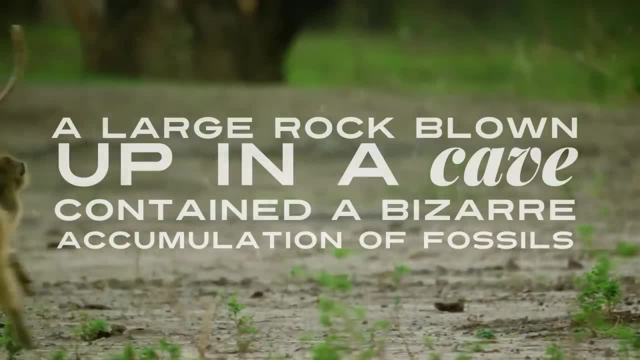 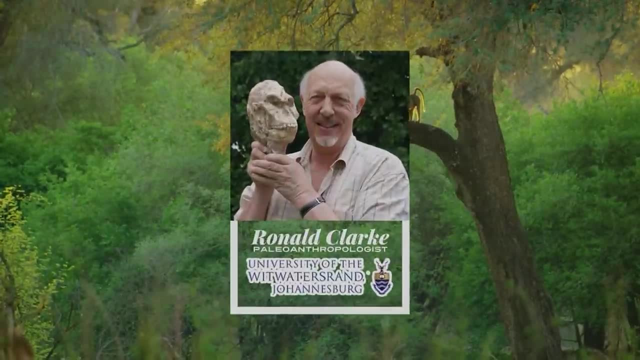 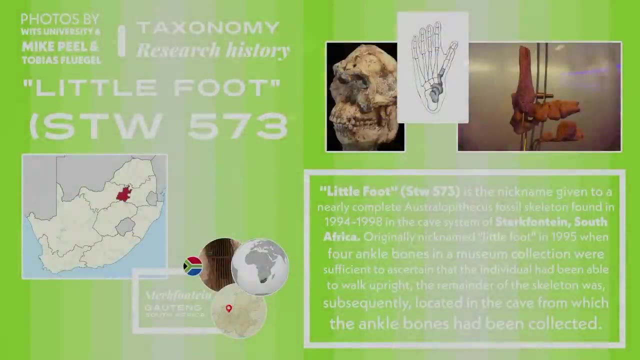 1997, A large rock blown up in a cave contained a bizarre accumulation of fossils. Paleoanthropologist Ronald J Clark, while searching through museum boxes, identified hominin fossils likely from the same individual which came from the Silberberg Grotto, a large cavern within the Circfantine caves. 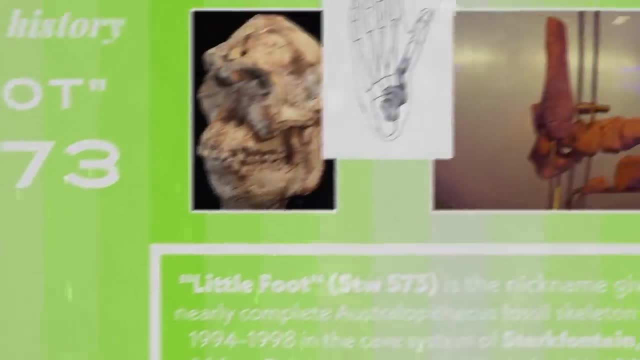 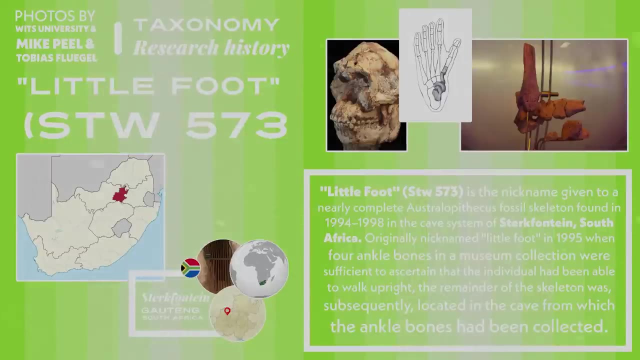 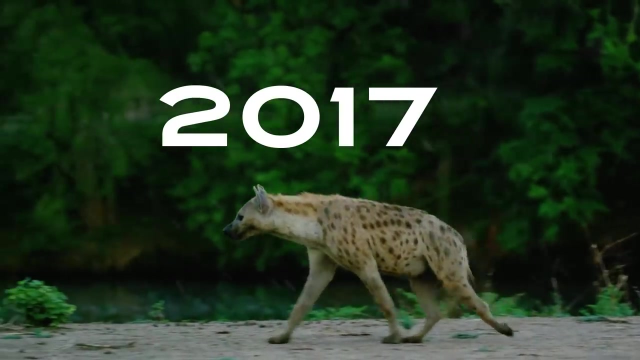 They recovered the rest of the fossil at the cave at a later date, and it took Clark and his team two full decades to fully extricate, clean and analyze the specimen, Work that was finally completed recently, in 2017.. This find would represent an almost complete 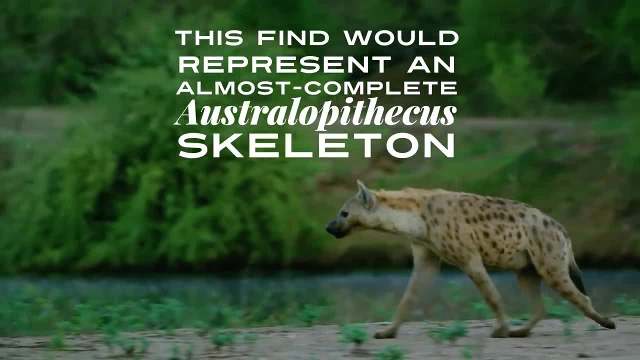 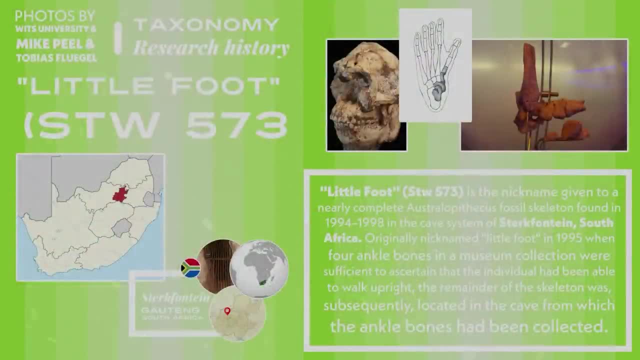 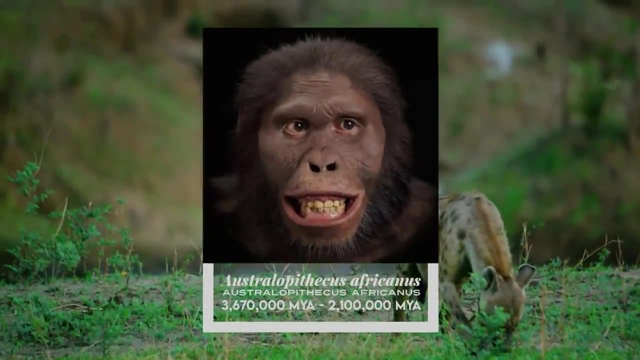 Australopithecus skeleton with a skull that was found in Gotang, South Africa. Dubbed Littlefoot, it was around 3.7 million years old. It was named Australopithecus prometheus and has since been placed with Australopithecus africanus. Other fossil remains found in the same cave in 2008 were named: 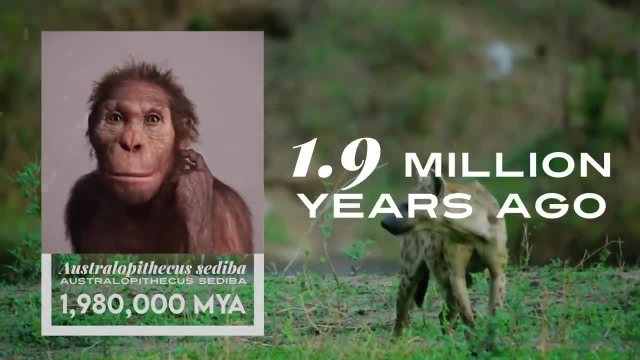 Australopithecus sediba. Other fossil remains found in the same cave in 2008 were named Australopithecus sediba, which lived 1.9 million years ago. Australopithecus africanus probably evolved into Australopithecus. 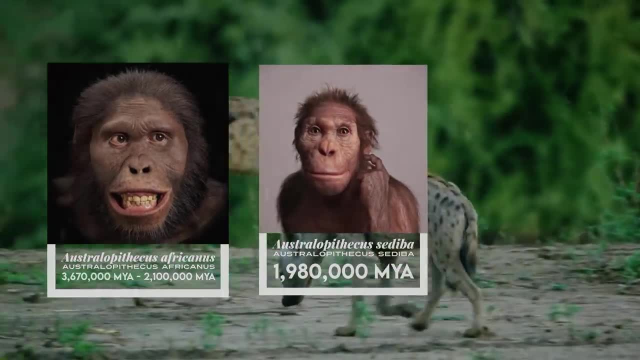 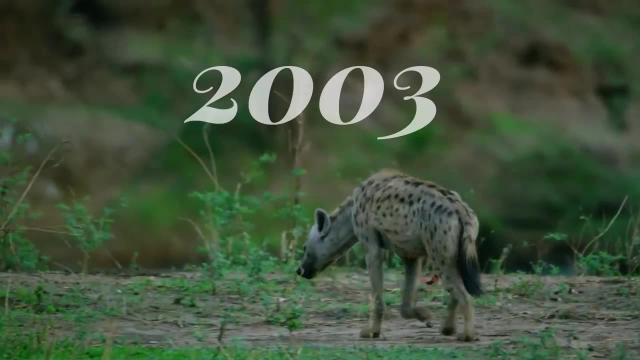 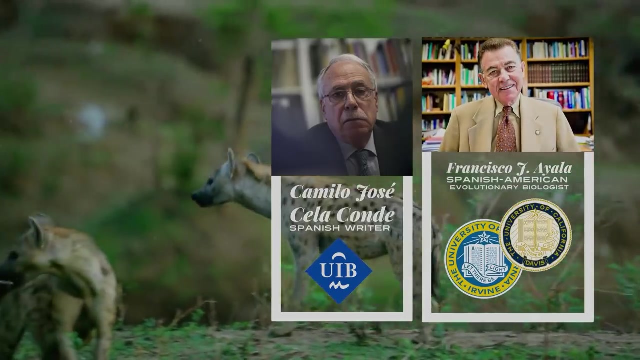 sediba, which some scientists believe may have evolved into Homo erectus, though this view is controversial and disputed by many. In 2003,, Spanish writer Camilo José Celaconde and the evolutionary biologist Francisco J Ayala proposed resurrecting the genus Praanthropus to house Ororin. 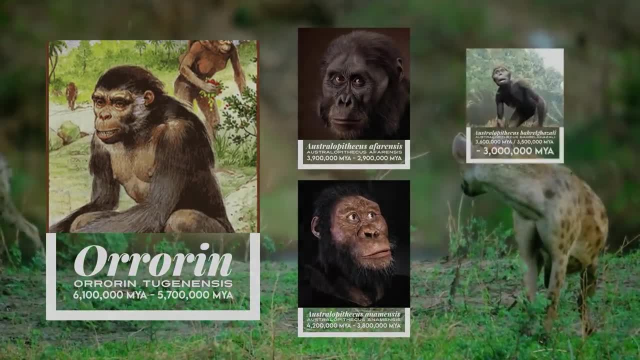 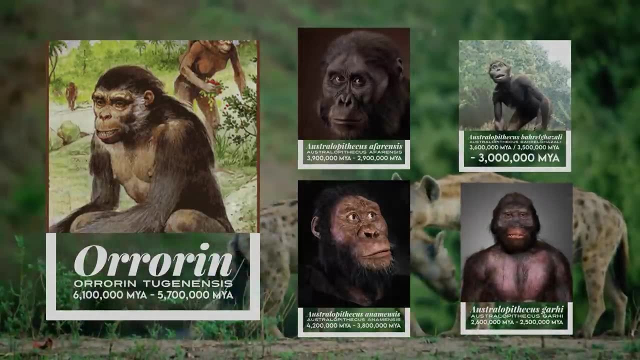 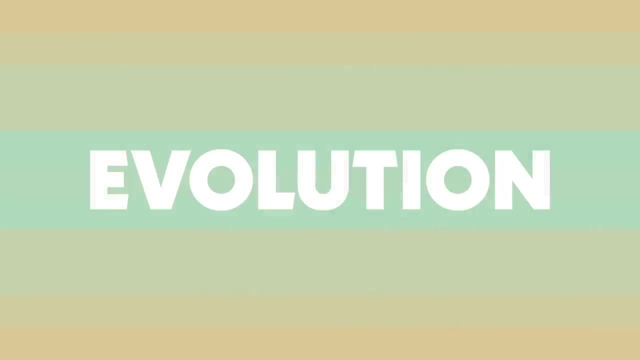 Australopithecus anamensis, Paralchazali and Gari. yet this genus has largely been dismissed and the credibility of the authors has been questioned. So what about its evolution? Which species arose from which, Well, Australopithecus anamensis may have descended from or was closely related to? 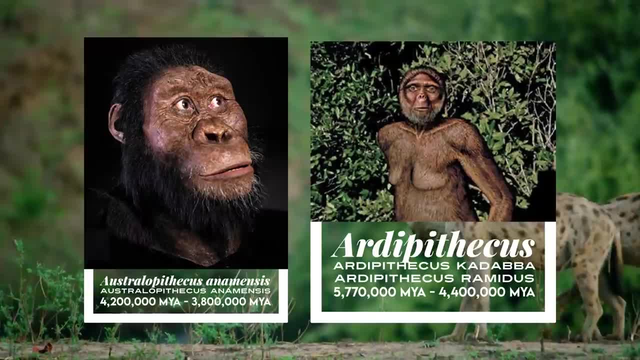 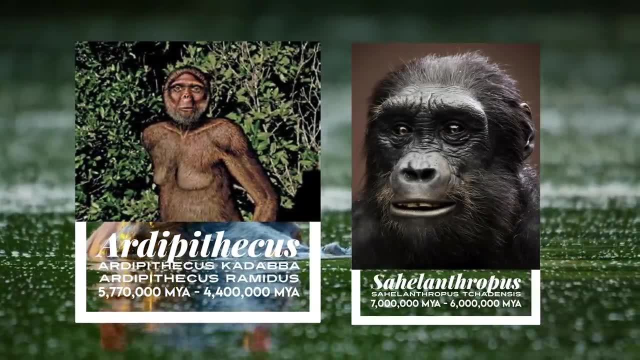 Ardipithecus remidus. Australopithecus anamensis shows some similarities to Australopithecus, similarities to both Ardipithecus ramidus and Coelanthropus, meaning they might have been connected in terms of their evolutionary pathways. 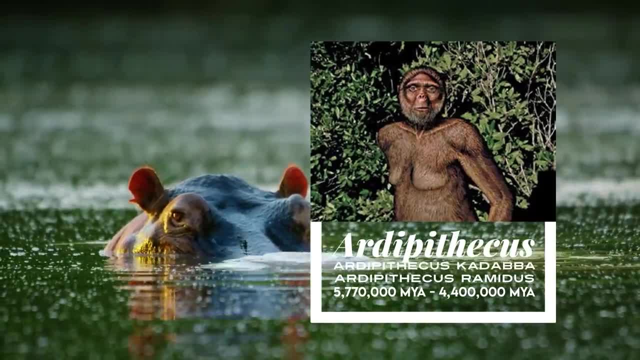 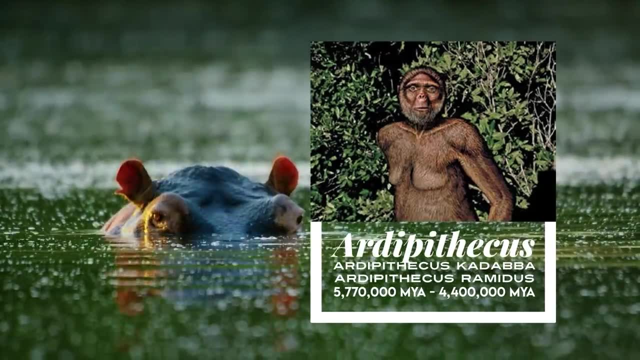 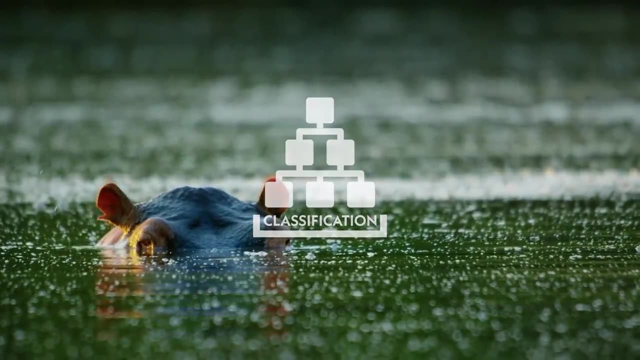 Ardipithecus is traditionally depicted as very similar to chimpanzees. It turns out that they more closely resemble bonobos, based on recent analysis about canine size and lack of canine sexual dimorphism. Its exact classification is a matter of ongoing debate. 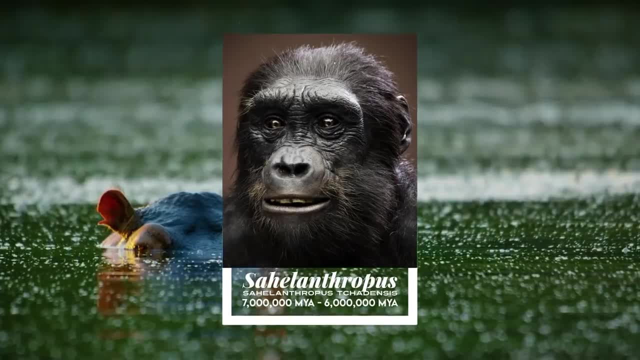 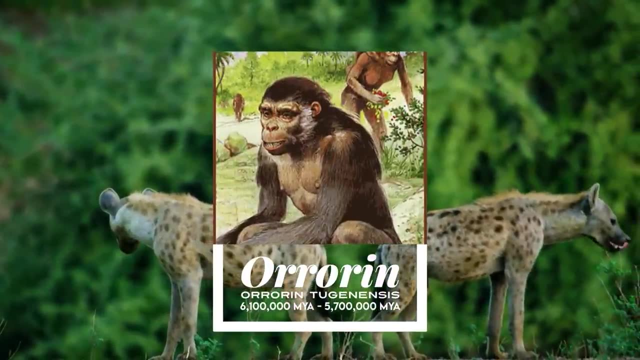 On the other hand, Coelanthropus chidensis lived close to the time of the chimpanzee-human divergence, possibly related to Ororik, a later hominin species. It may have been ancestral to both humans and chimpanzees, leading to placement in homininity. 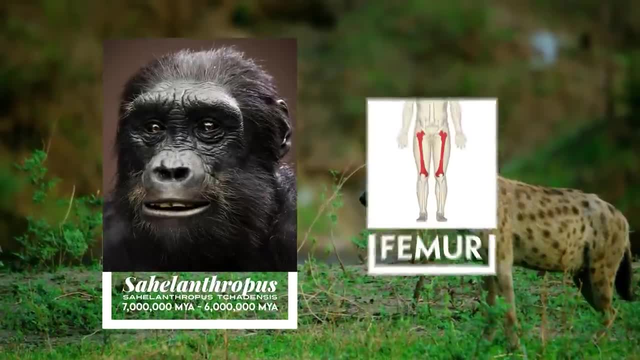 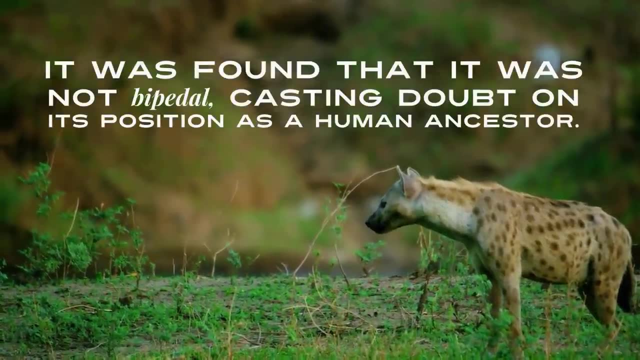 yet in 2020, a Coelanthropus, femur, was analyzed and it was found that it was not bipedal, casting doubt on its position as a human ancestor. Australopithes shared several traits with Mothra. Australopithes are known as modern apes and humans and were widespread throughout eastern 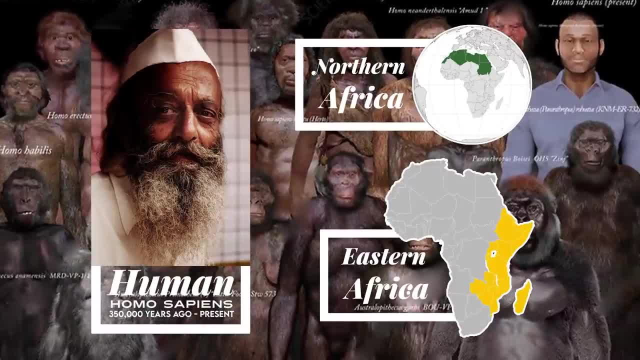 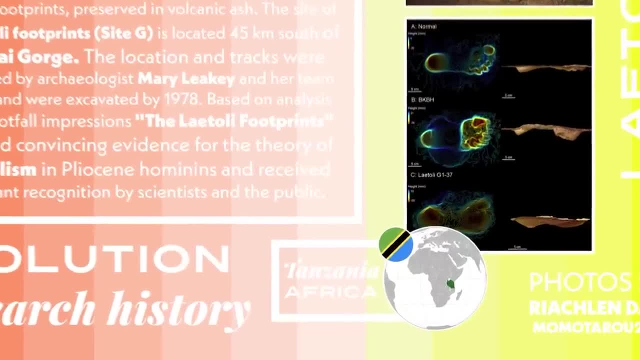 and northern Africa by 3.5 million years ago. The earliest evidence of fundamentally bipedal hominins is a 3.6 million year old fossil trackway in Laetoli, Tanzania, which bears a remarkable similarity to those of modern. 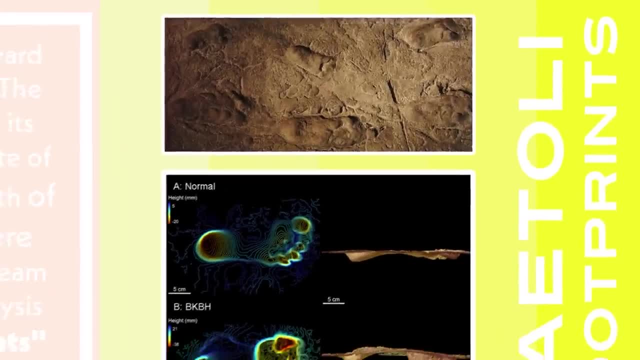 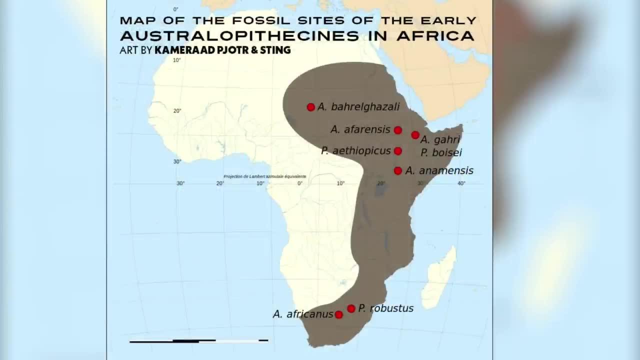 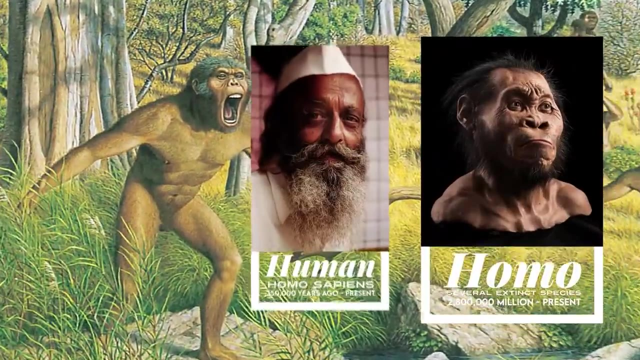 humans. These are known as the Laetoli footprints. The footprints have generally been classified as australopithes, as they are the only form of pre-human hominins known to have existed in that region, The first undisputed evidence of the genus Homo, the genus that includes modern human. 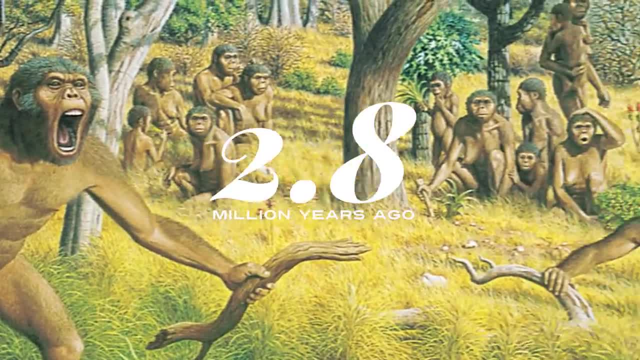 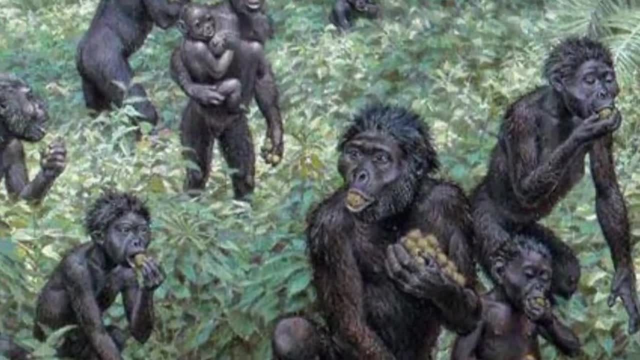 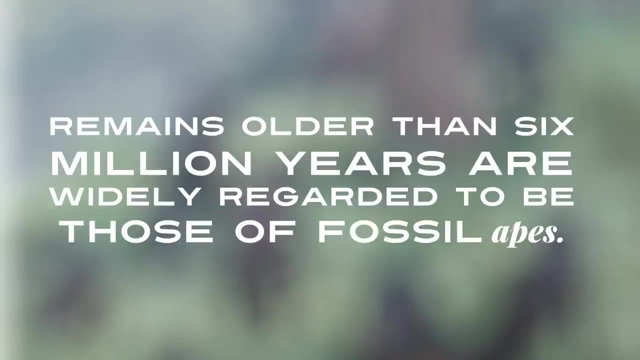 beings appears as early as 2.8 million years ago, and some traits of Homo resembled those of earlier species of Australopithecus. however, there is controversy surrounding the identity of the earliest species of Homo. In contrast, remains older than 6 million years are widely regarded to be those of fossil. apes- Australopithecanus Australopithecus. Australopithecus, The 43nd genus of Australopithecus and Homo overlapped in time with one another for nearly 1 million years, According to the Chimpanzee Genome Project. the human chimpanzee last common ancestor. 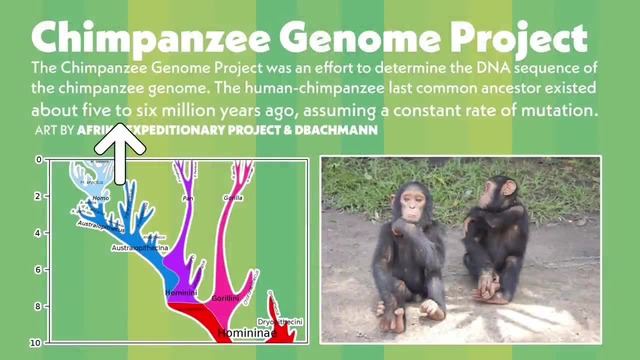 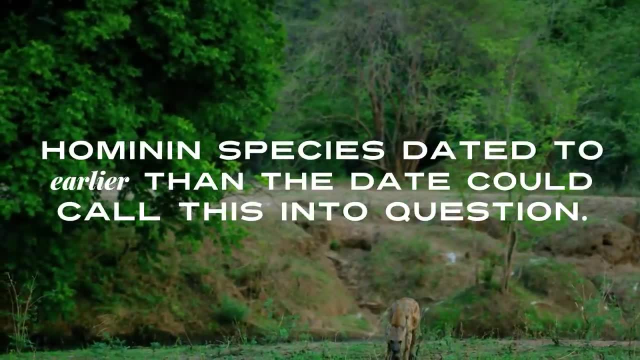 existed about 5-6 million years ago, assuming a constant rate of mutation. Nonetheless, hominin species dated to earlier than the date could call this into question. Cezanthropus Schadensis, commonly called Tumot, is about 7 million years old and 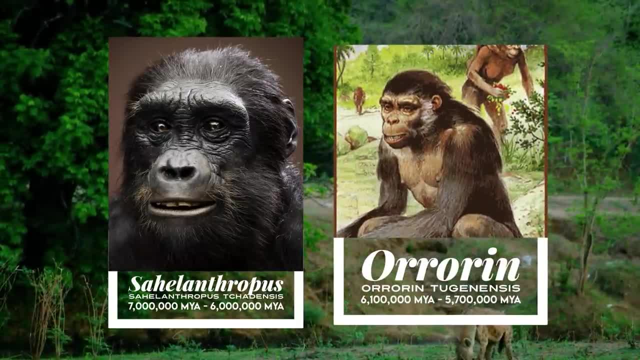 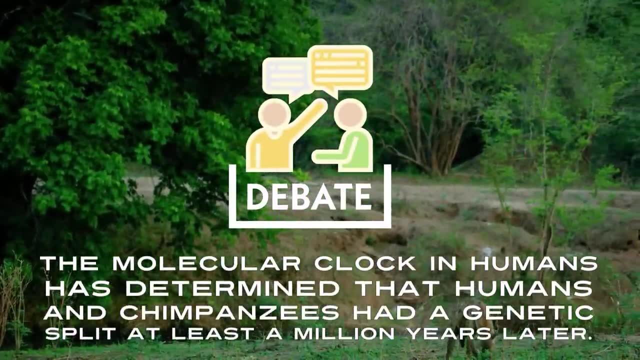 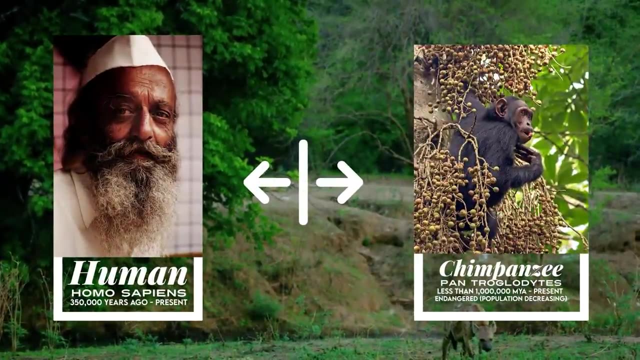 and Orenthogenensis lived at least 6 million years ago. Since little is known of them, they remain controversial among scientists, since the molecular clock in humans has determined that humans and chimpanzees had a genetic split at least a million years later. 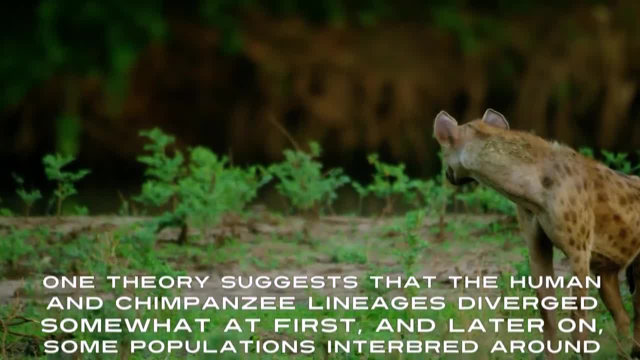 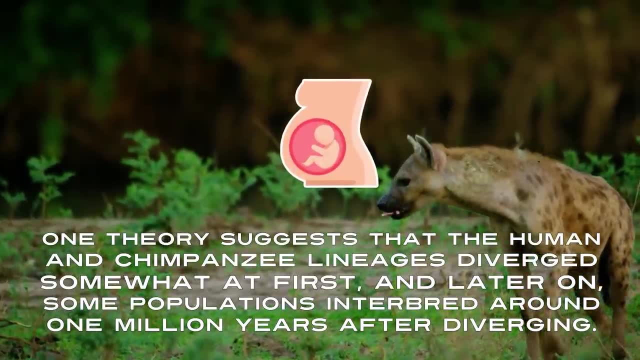 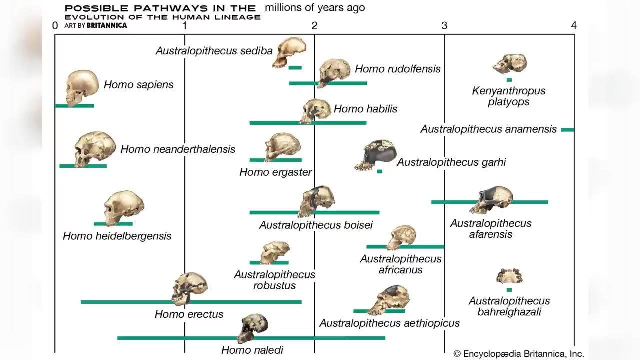 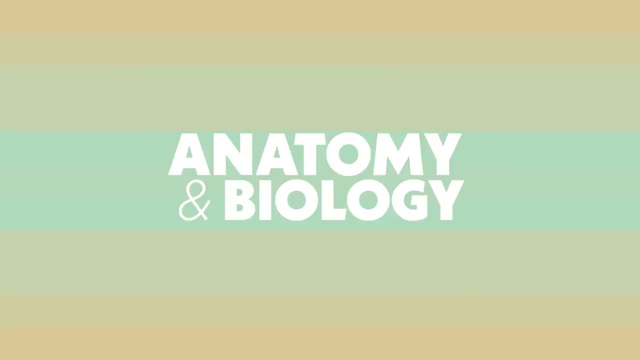 One theory suggests that the human and chimpanzee lineages diverged somewhat at first and later on. some populations interbred around 1 million years after diverging. Here are some proposed pathways in the evolution of the human lineage. Let us now delve into the anatomy and biology of Australopithecus. 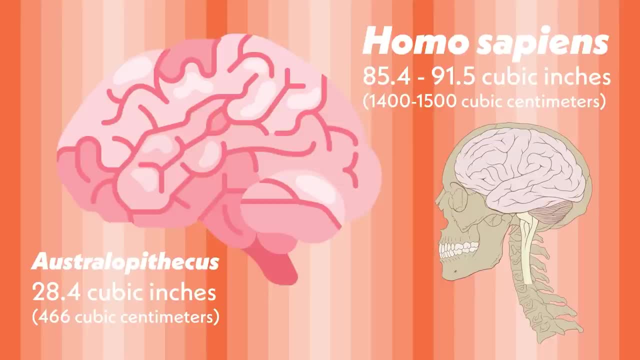 The brains of most species of Australopithecus were roughly 35% of the size of a modern human brain, with an endocranial volume average of 28.4 cubic inches or 466 cubic centimeters. Despite the fact that this is more than 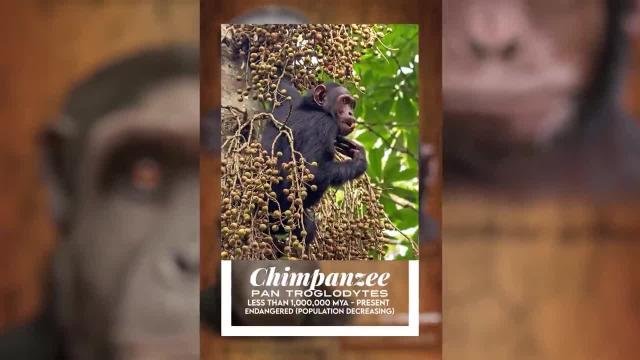 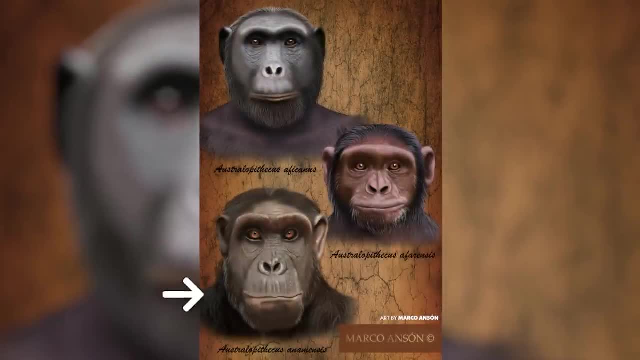 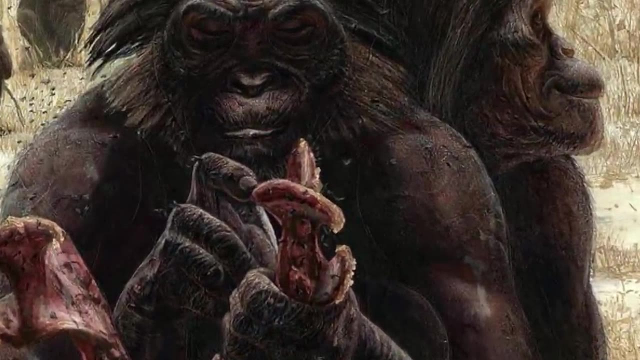 the average endocranial volume of chimpanzee brains at 22 cubic inches or 360 cubic centimeters. the earliest australopiths, like Australopithecus anamensis, appear to have been within the chimpanzee range, whereas some later australopith specimens have a larger endocranial volume. 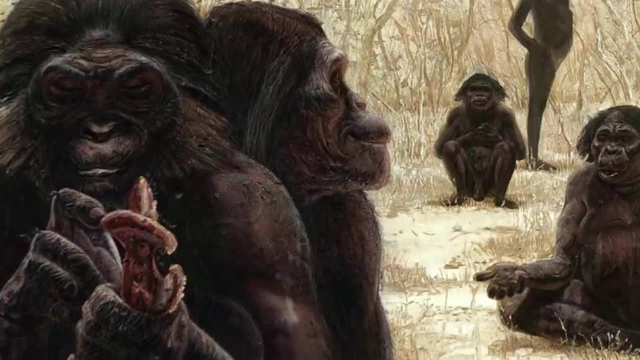 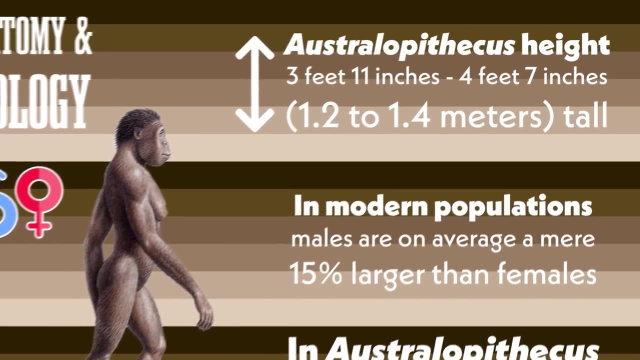 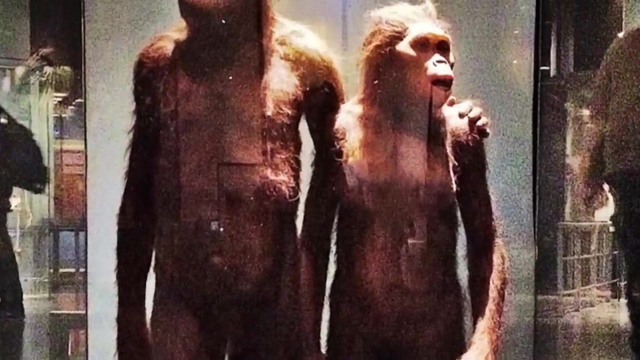 than that of some early Homo fossils. Most species of Australopithecus were diminutive and gracile, typically standing 3 feet 11 inches to 4 feet 7 inches. It seems possible that they exhibited a considerable degree of sexual dimorphism. 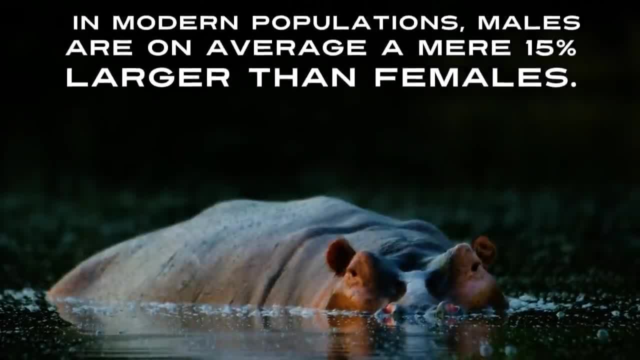 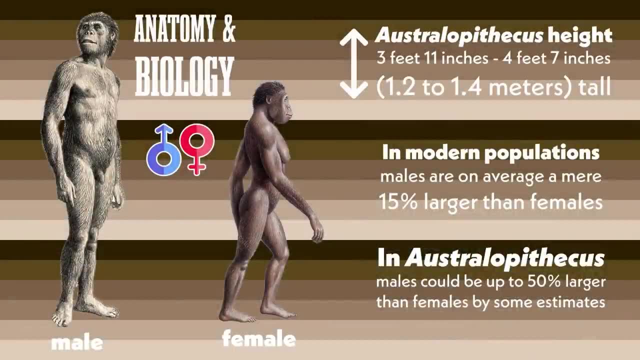 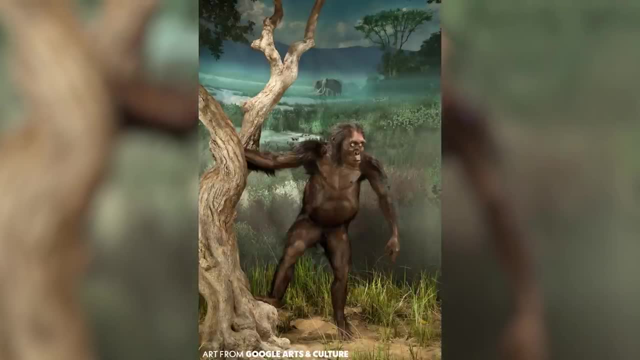 with males being larger than females. In modern populations, males are, on average, a meter 15% larger than females, while in Australopithecus, males could be up to 50% larger than females by some estimates. However, the degree of sexual dimorphism is debated due to the fragmentary nature of Australopithecus'. 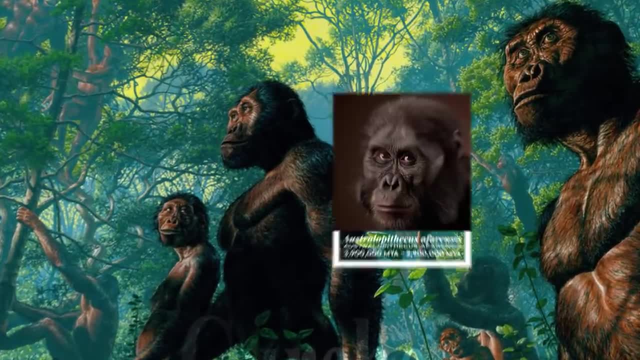 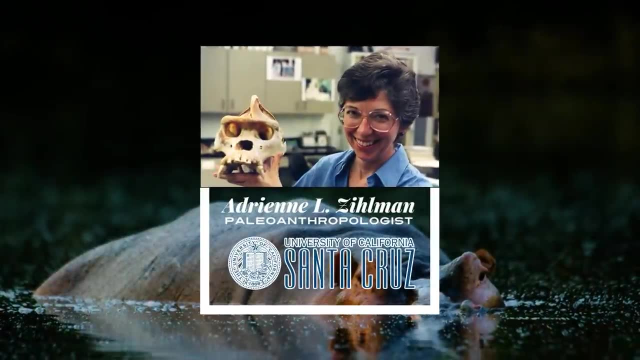 remains. One paper finds that Australopithecus afarensis had a level of dimorphism close to modern humans. According to Adrian Zillman, one of the key figures of paleoanthropology, Australopithecus'. 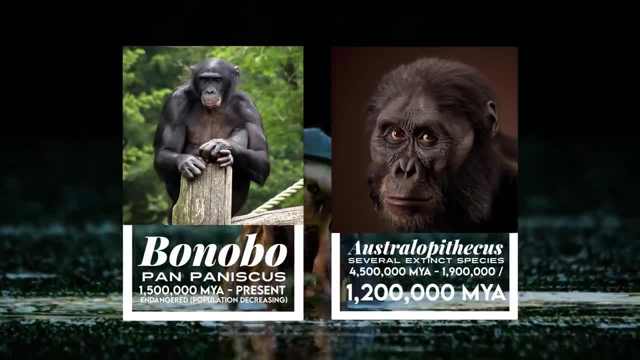 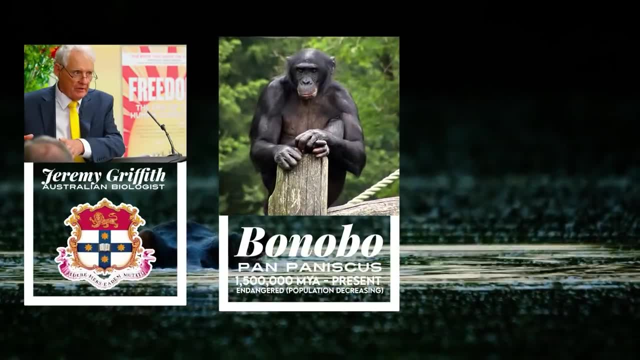 body proportions closely resemble those of bonobos, also known as pan-boniscus, leading evolutionary biologist, Jeremy Griffith to suggest that bonobos may be phenotypically similar to Australopithecus. Furthermore, thermoregulatory models suggest that Australopithecus' body proportions are: 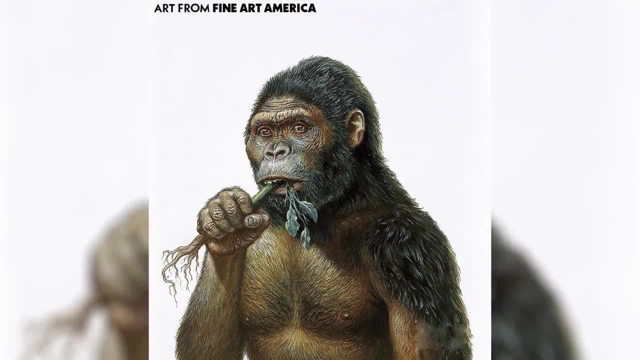 similar to those of the male Bonobos. The body proportions of the male Bonobos are similar to those of the female Bonobos and, in fact, the size of an actual human is not completely different from that of a male Bonobo. 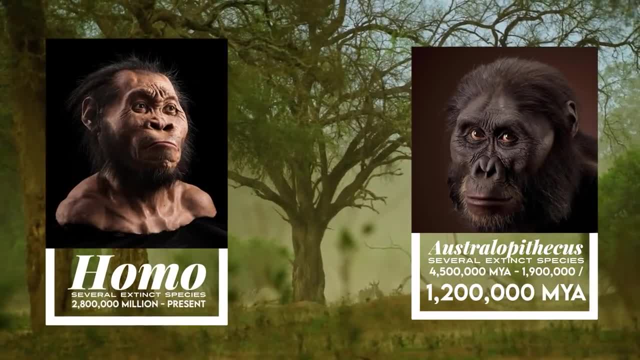 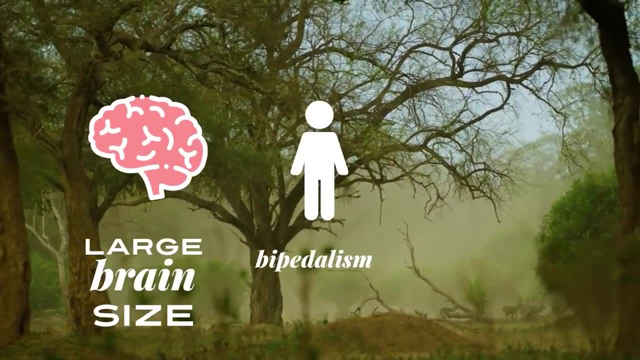 The fossil record seems to indicate that Australopithecus is ancestral to Homo and modern humans. It was once assumed that large brain size had been a precursor to bipedalism. yet the discovery of Australopithecus with a small brain but developed bipedality upset this. 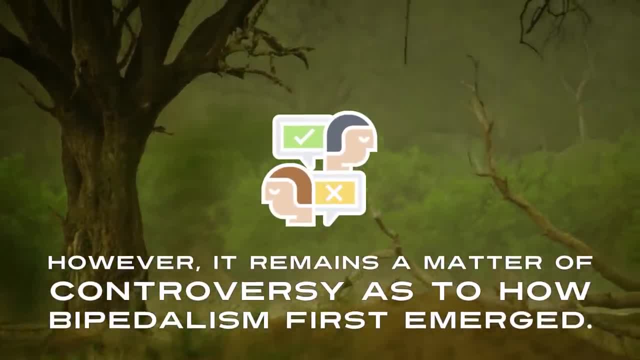 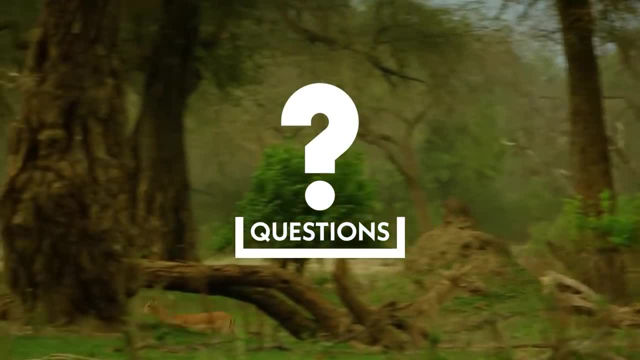 theory. However, it remains a matter of controversy as to how bipedalism first emerged. The discovery of Australopithecus with a small brain, but developed bipedality, upset this theory. This is amongst the greatest mysteries in paleoanthropology, crucial to our understanding. 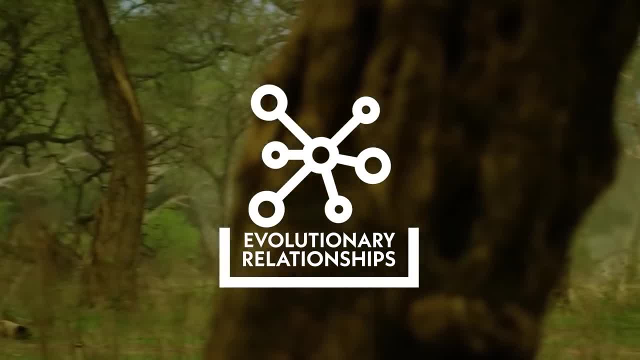 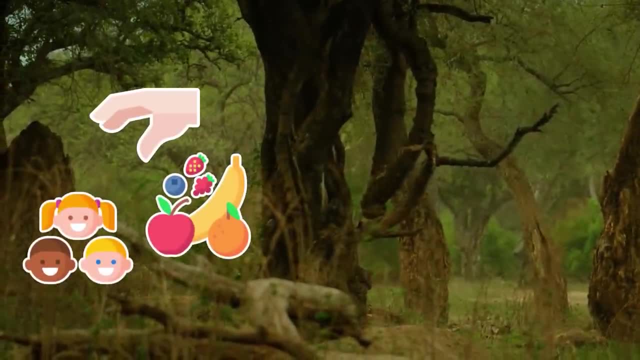 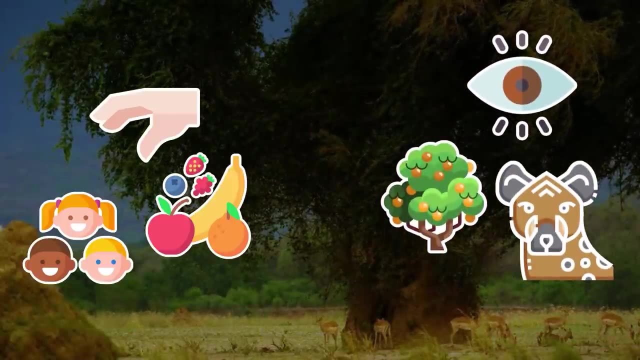 of evolutionary pathways of early hominids. The advantages of bipedalism were that it left the hands free to grasp objects like caring, food and young, and allowed the eyes to look over tall grasses for possible food sources or predators. But it is also argued that these advantages were 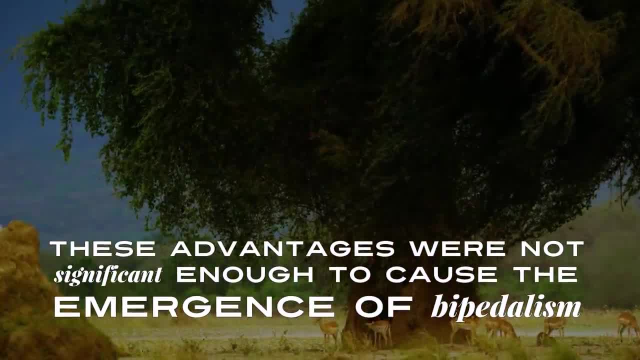 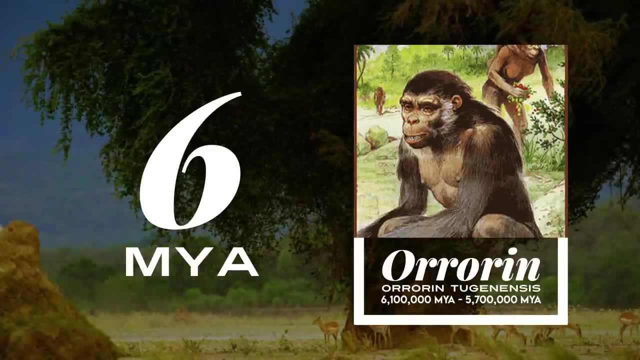 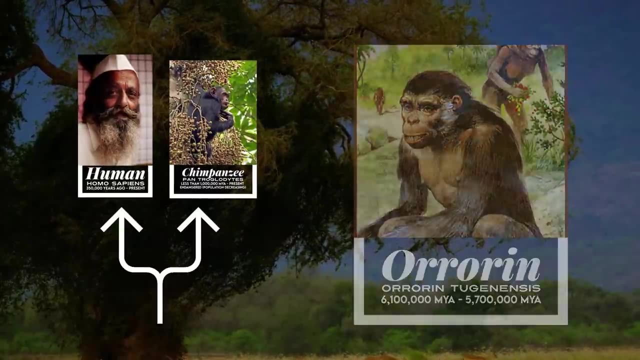 not significant enough to cause the emergence of bipedalism. Earlier fossils, including Aurorantigenensis, indicate bipedalism around 6 million years ago, around the time of the split between humans and chimpanzees indicated by genetic studies. This suggests that erect 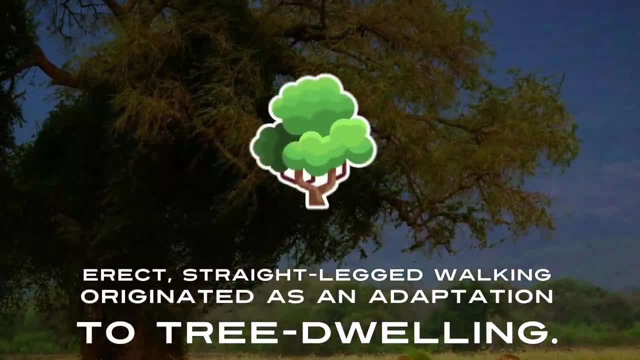 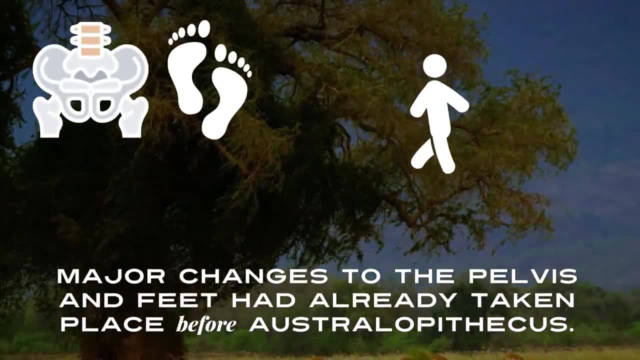 straight-legged walking originated as an adaptation to tree-dwelling. Major changes to the pelvis and feet had already taken place before Australopithecus. It was the first time that a bipedalist could be identified as a bipedalist. 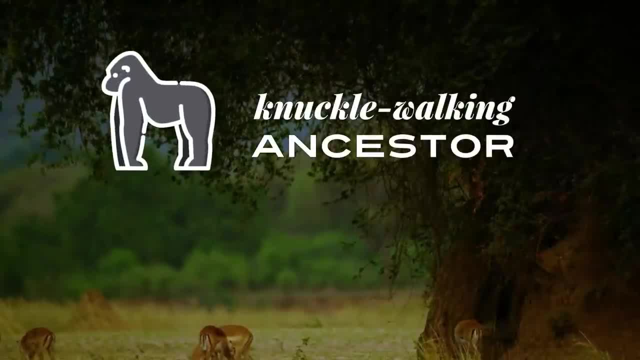 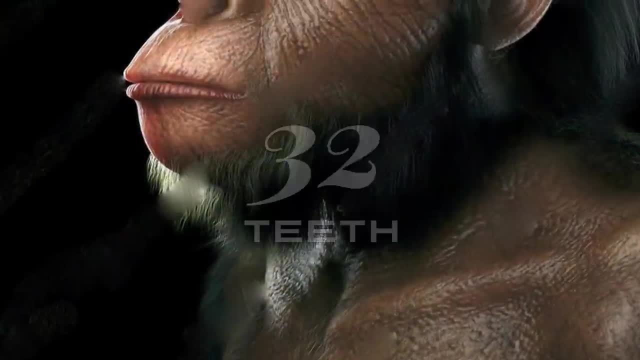 It was the first time that a bipedalist could be identified as a bipedalist. It was once thought that humans descended from a knuckle-walking ancestor, but this is not well substantiated. outdated and stereotypical Australopithecines have 32 teeth as modern. 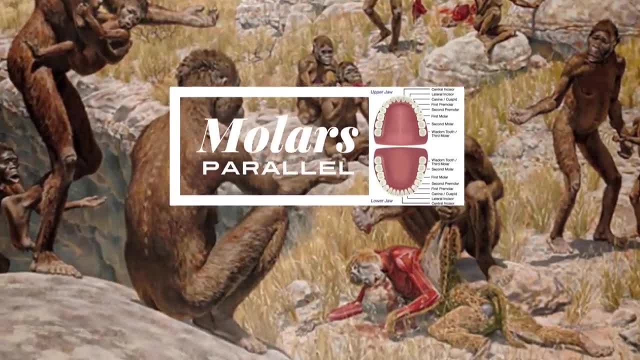 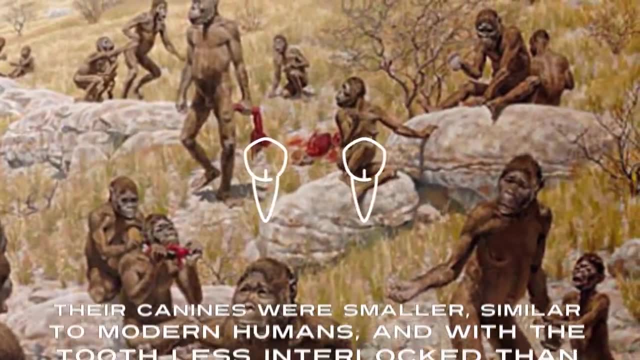 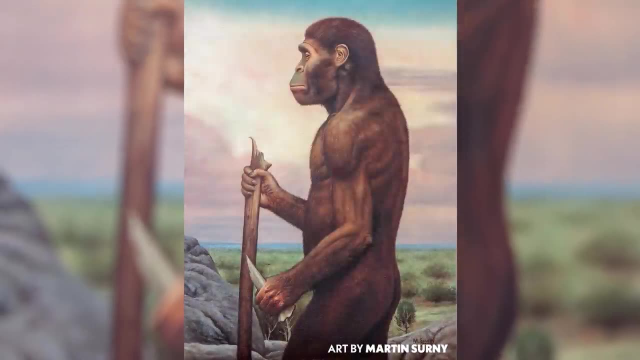 humans do. Their molars were parallel, similar to those of great apes, and they had a slight pre-canine gap or diastema. Their canines were smaller, similar to modern humans and with the tooth less interlocked than in previous hominids. In fact, in some Australopithecines. 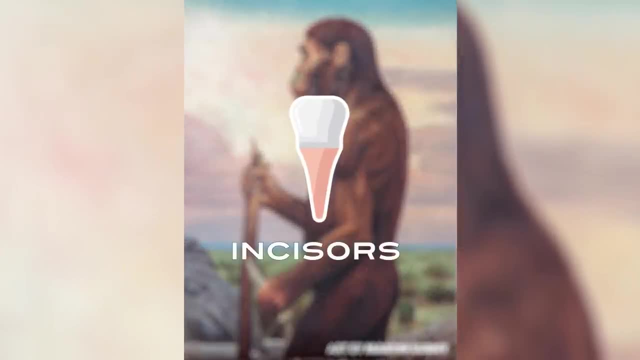 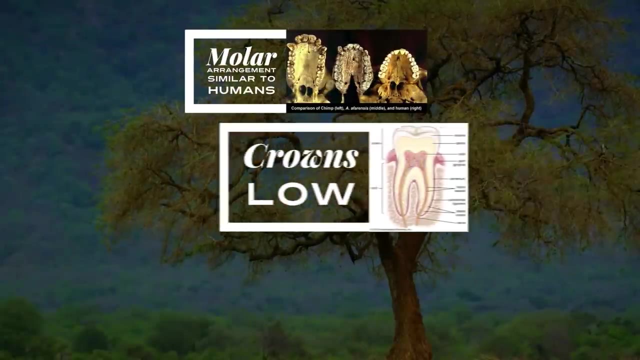 the canines are shaped more like incisors. The molars of Australopithecus fit together in much the same way those of humans do, with low crowns and four low rounded cusps used for crushing. They have cutting edges on the crests. 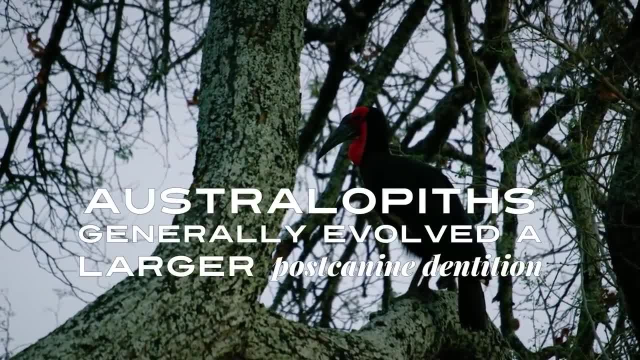 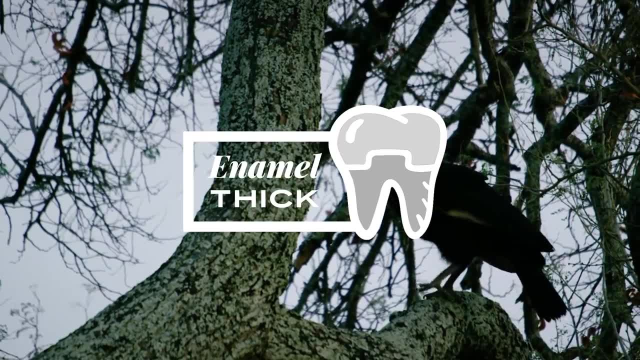 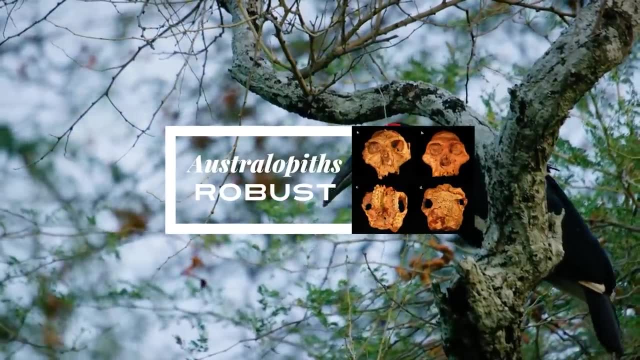 However, Australopiths generally evolved a larger post-canine dentition with thicker enamel. Australopiths in general had thick enamel, like Homo, while other great apes have markedly thinner, thinner enamel. Robust Australopiths wore their molar surfaces down flat. 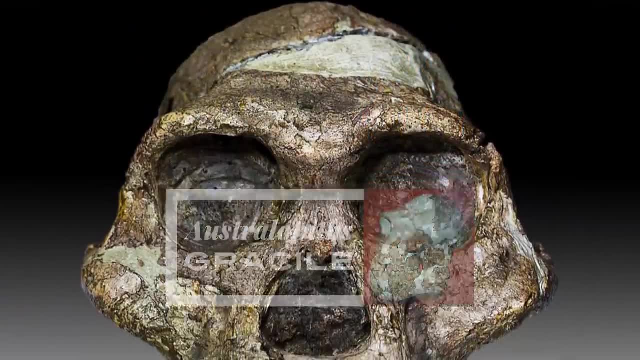 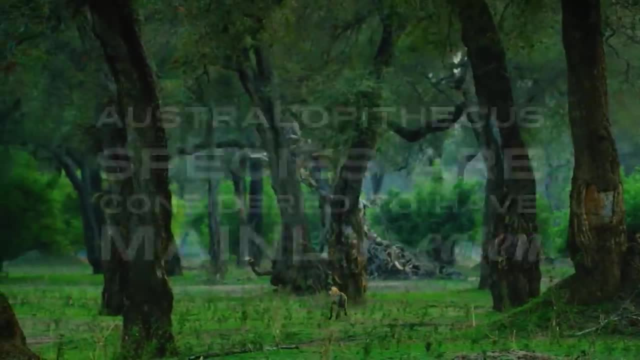 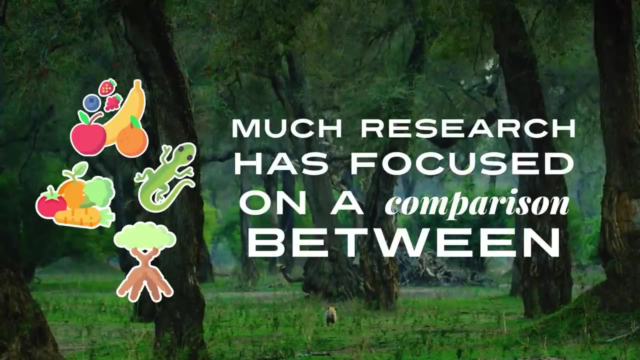 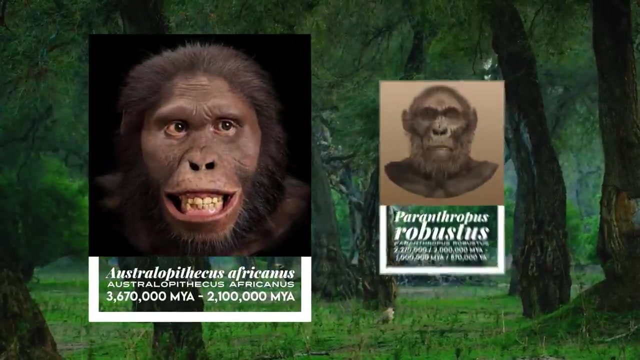 unlike the more grasshopped species who kept their crests, Australopithecus species are considered to have mainly eaten fruit, vegetables and tubers, and perhaps easy to catch animals like small lizards. Much research is focused on a comparison between the South African species Australopithecus africanus and Paranthropus. 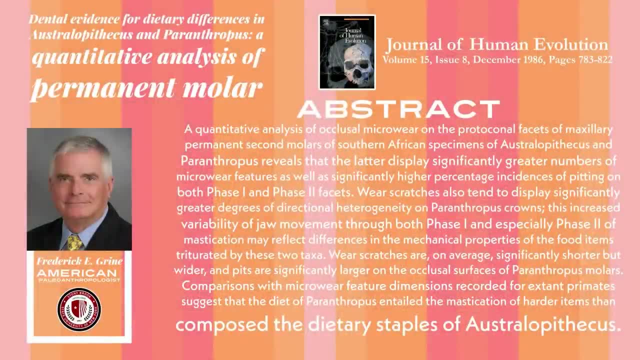 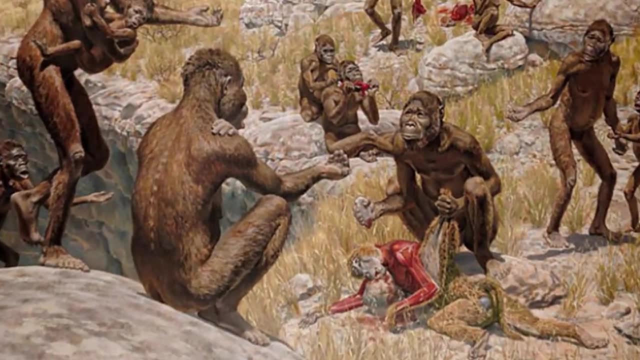 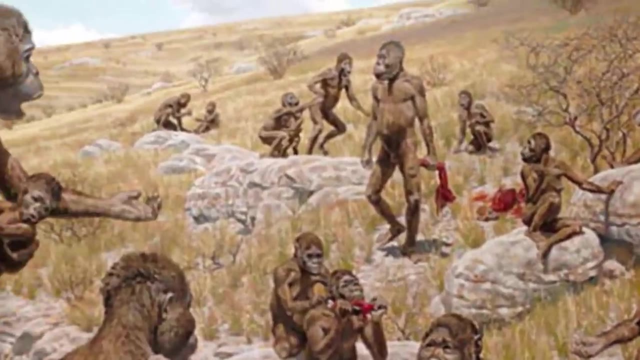 robustus. Early analysis of dental micro-wear in these two species demonstrated. compared to Paranthropus robustus, Australopithecus africanus had fewer micro-wear features and more scratches, as opposed to pits on its molar-wear facets, Micro-wear patterns on the cheek teeth. 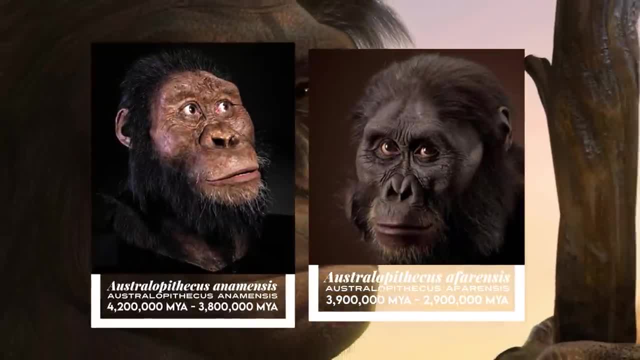 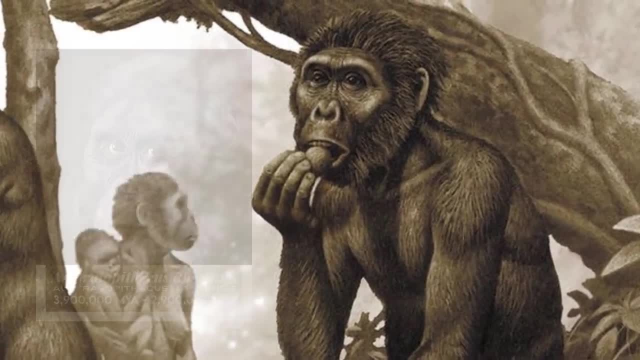 of Australopithecus afarensis and Australopithecus anamensis indicate that Australopithecus afarensis predominantly ate fruits and leaves, whereas Australopithecus anamensis feasted on grass. The differences between Australopithecus africanus and Paranthropus. 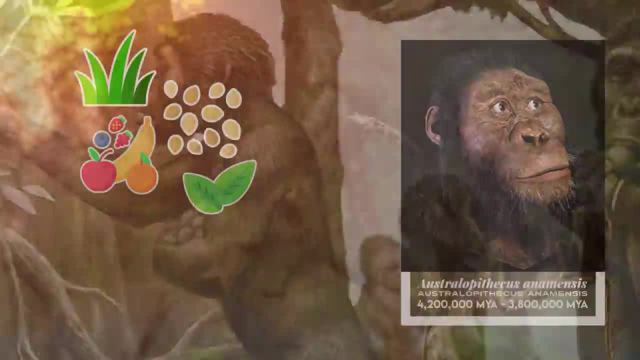 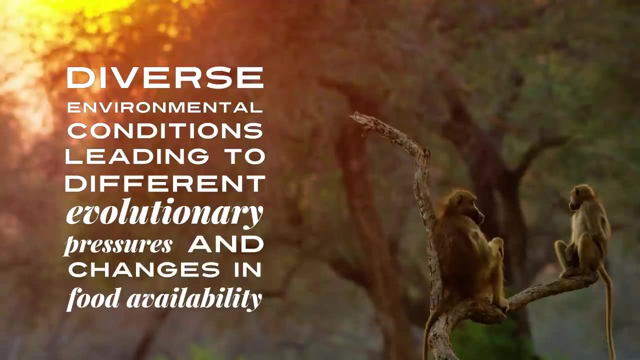 are that Australopithecus anamensis ate only grasses and seeds, in addition to fruits and leaves. There is variation between the diet of numerous species of Australopithecus, and this is largely due to diverse environmental conditions, leading to different evolutionary. 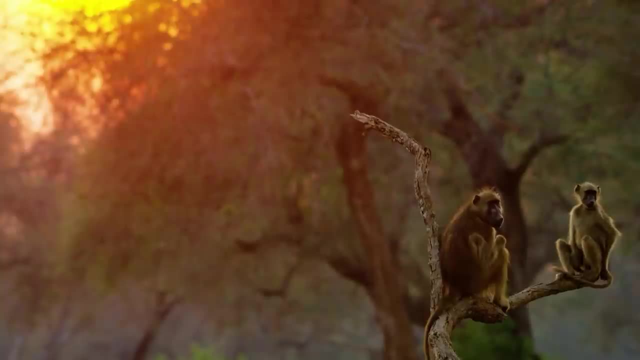 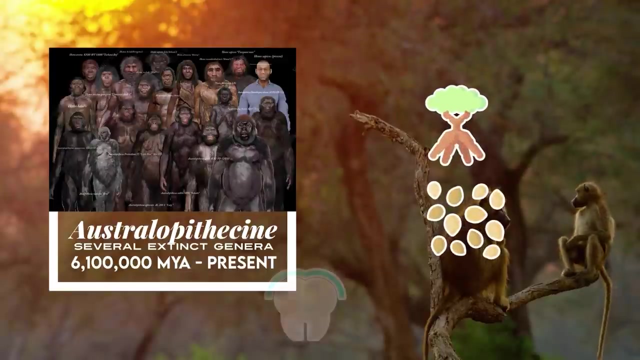 pressures and changes in food availability. The thickening of enamel in Australopithes may have been a response to eating more ground-bound foods like tubers, nuts and cereal grains with gritty dirt and other small particulates which would wear away enamel. 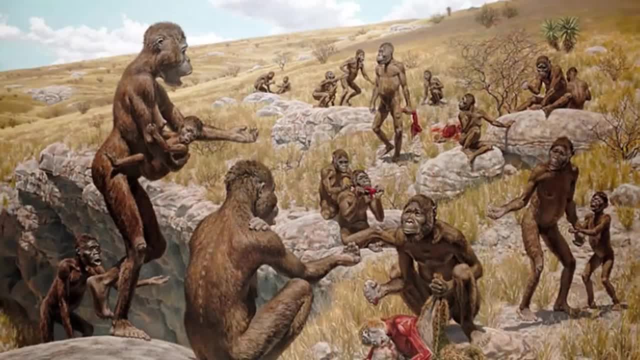 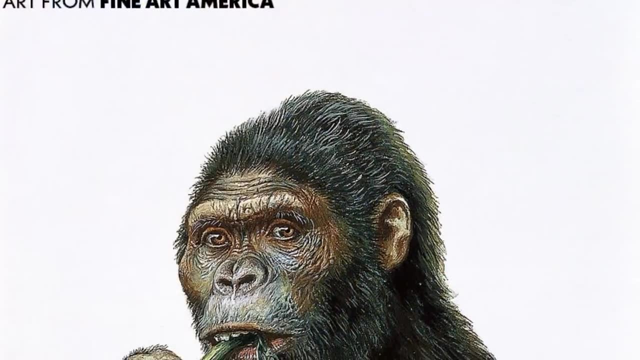 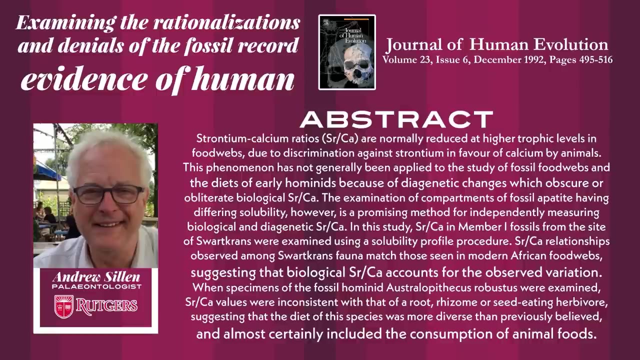 Grass-style Australopithes had larger incisors, which indicates tearing food was important, perhaps eating scavenged meat. Nonetheless, the wearing patterns on the teeth support a largely herbivorous diet. In 1992, trace element studies of the strontium-calcium ratios in robust 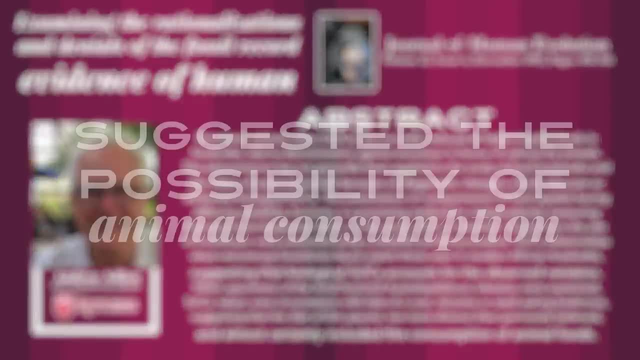 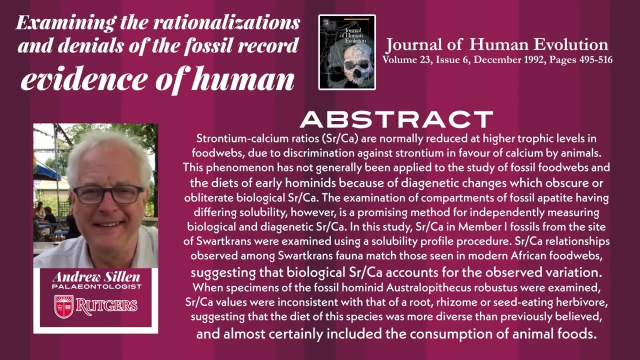 australopithe fossils suggested the possibility of animal consumption, as was brought to light in 1994 using stable carbon isotopic analysis. In 2005, fossil animal bones with butchery marks dating to 2.6 million years ago were. 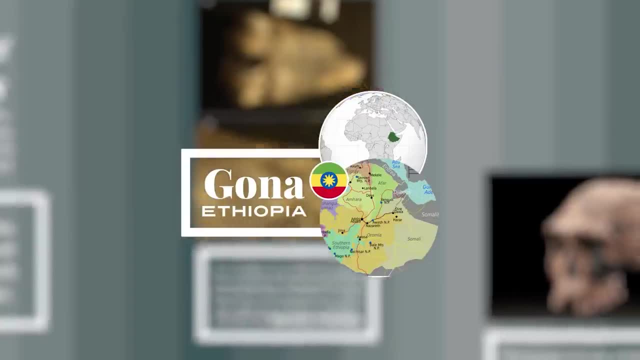 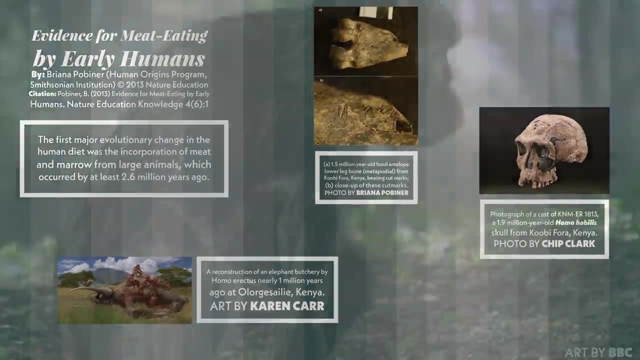 found at the site of Gona, Ethiopia. This implies meat consumption by at least one of three species of hominids occurring around that time: Australopithecus africanus gari and or Paranthropus aethiopicus. 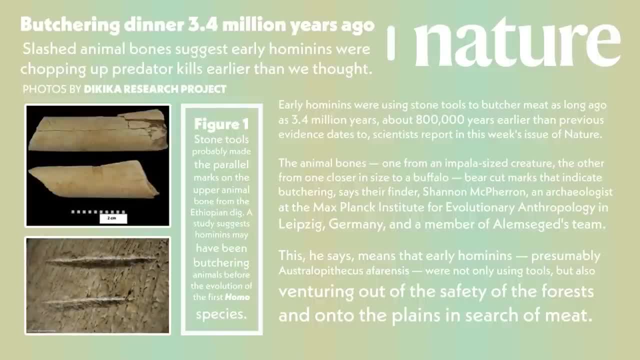 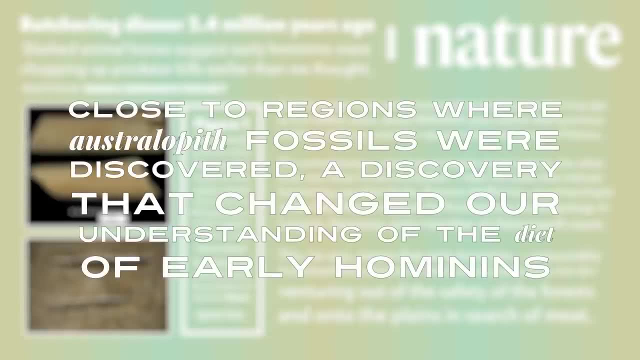 In 2010,. fossils of butchered animal bones dated to 3.4 million years old were found in Ethiopia, close to a region where australopith fossils were discovered, a discovery that changed our understanding of the diet of early hominids. 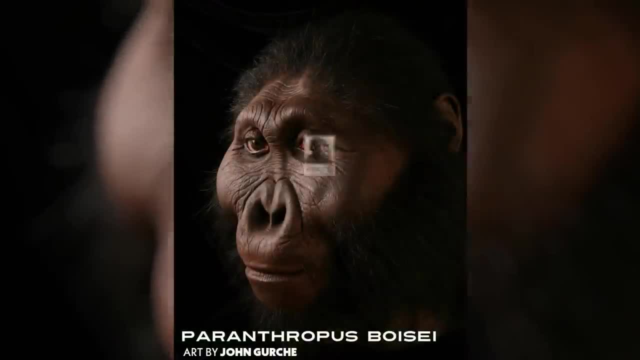 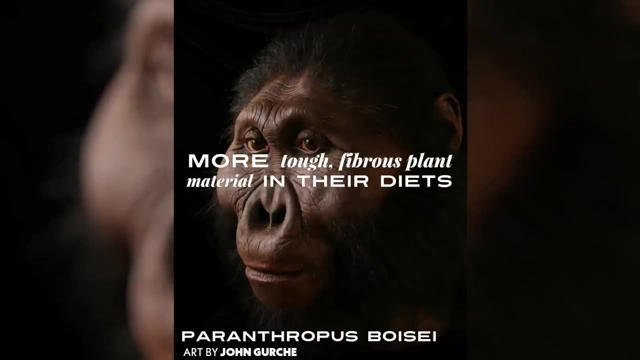 Robust australopithecines, including Paranthropus, had larger cheek teeth than gracile australopiths, possibly because robust australopithecines had more tough fibrous plant material in their diets, Whereas gracile australopithecines had more fiberous plant material in their diets. 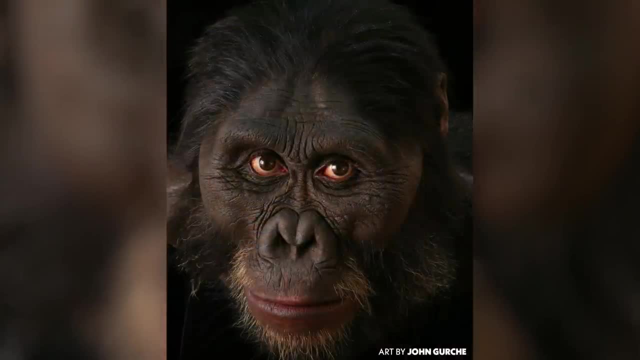 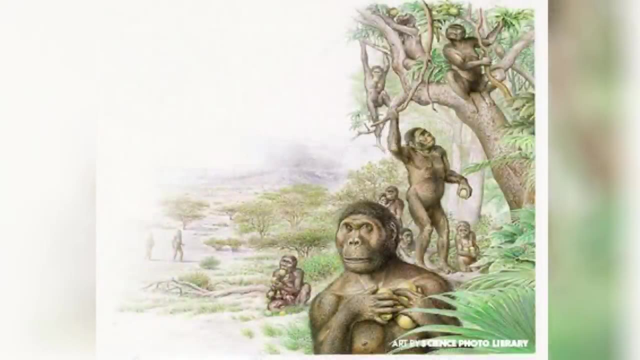 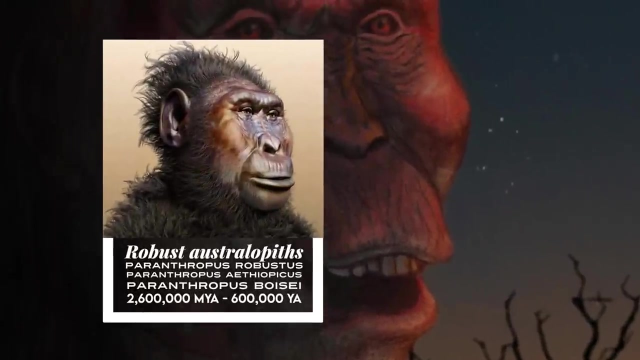 However, such a divergence in chewing adaptations may instead have been a response to fallback food availability. In leaner times, robust and gracile australopithecines may have turned to different, low-quality foods, with fibrous plants for robust australopithecines and hard food for the gracile australopithecine. 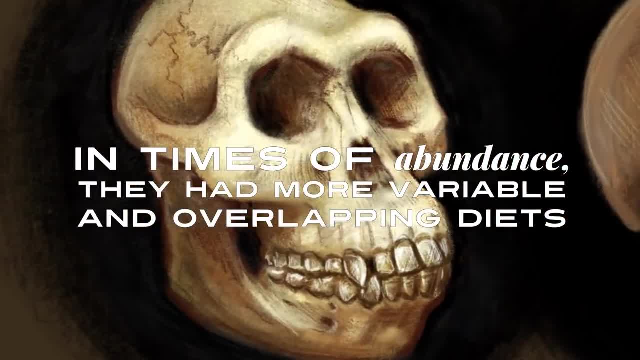 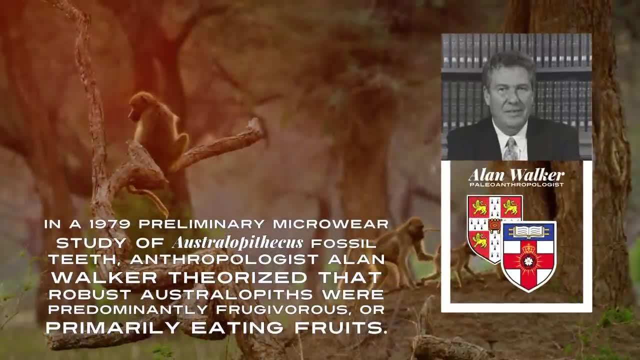 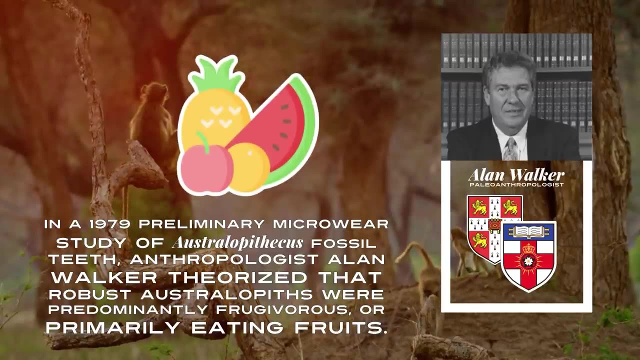 However, in times of abundance they had more variable and overlapping diets. In a 1979 preliminary study, a study was conducted in the United States of America. where a study was conducted in the United States of America, The study found that robust australopithecines were predominantly frugivorous or primarily 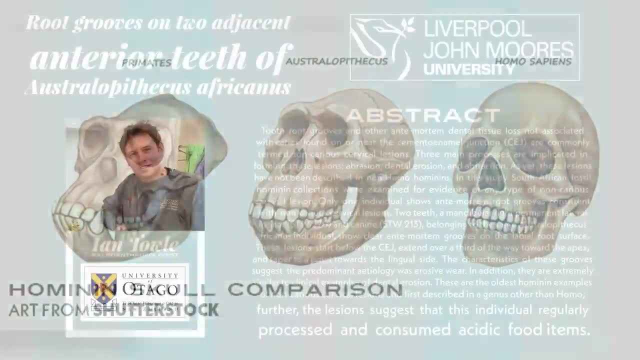 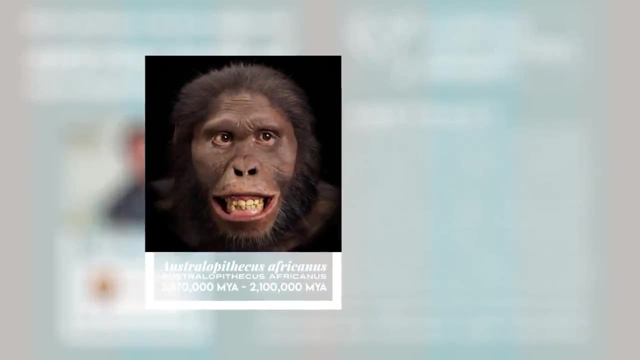 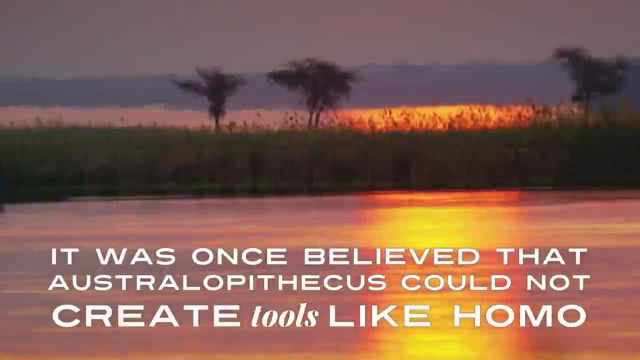 eating fruit. A recent 2018 study found non-carious cervical lesions caused by acid erosion on the teeth of australopithecines africanus, probably caused by consumption of acidic fruit. Conclusion: It was once believed that australopithecines 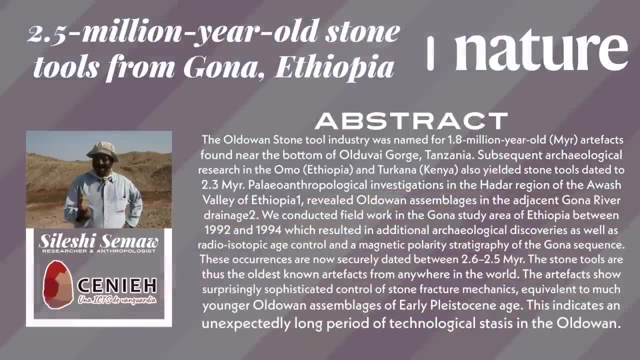 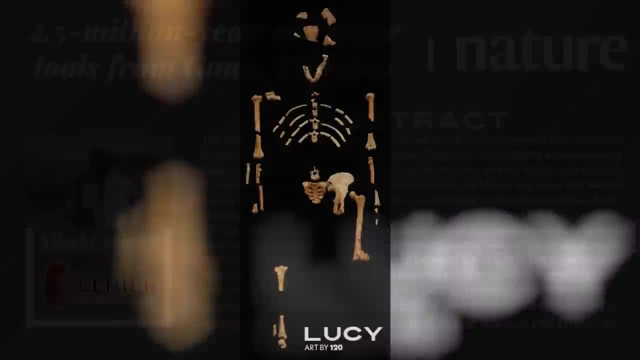 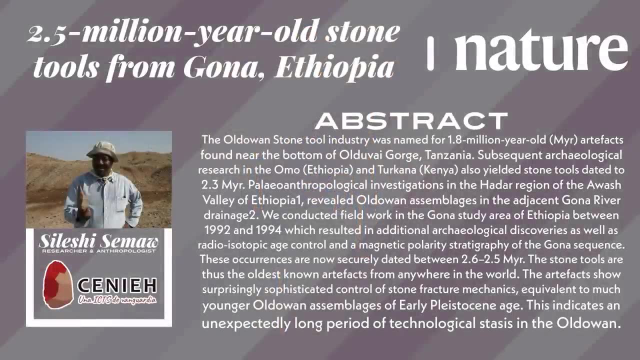 could not create tools like teeth. Yet the discovery of Australopithecus gari, associated with large mammal bones bearing evidence of processing by stone tools, demonstrated this not to have been the case. Discovered in 1994, this was the oldest evidence of manufacturing at the time. 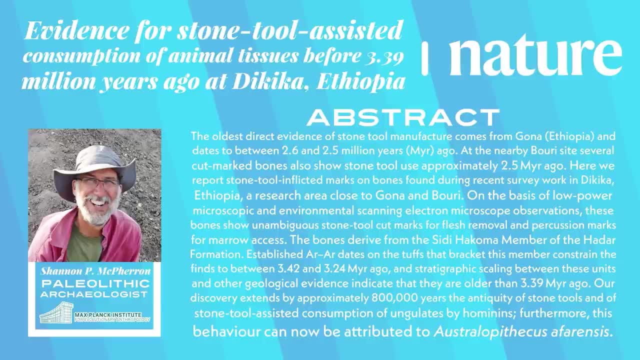 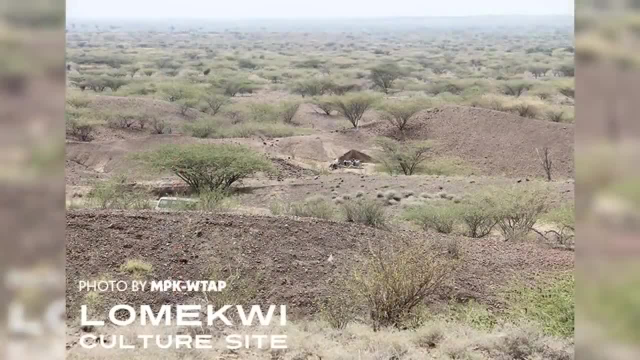 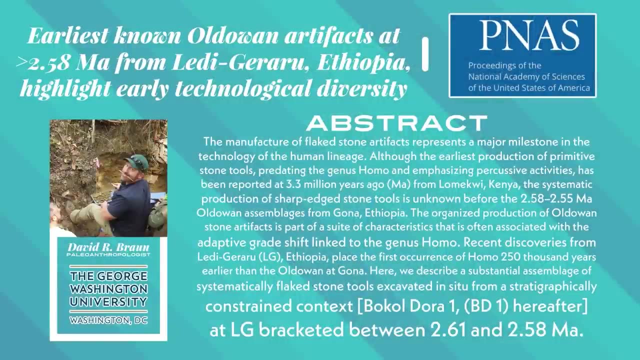 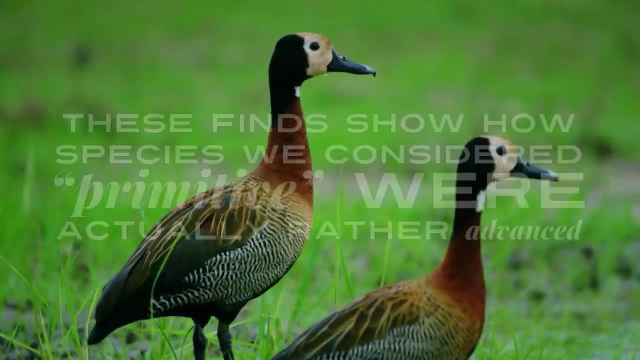 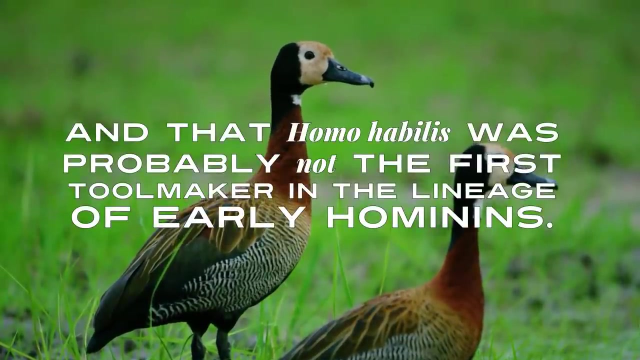 to the Lomekwi culture, from Lake Turkana to the Lomekwi culture, from the Lomekwi and Giza civet culture, from the Lomekwi culture, from the Lomekwi culture, from the Turkana into the Textile. 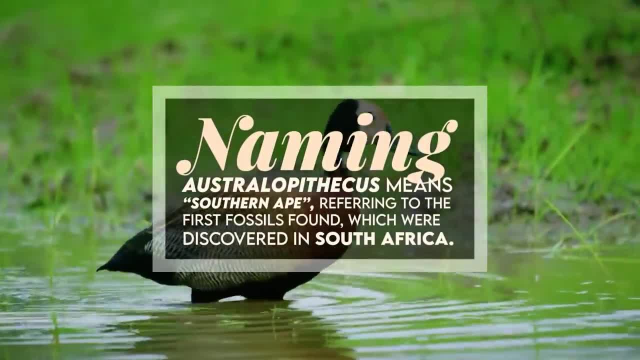 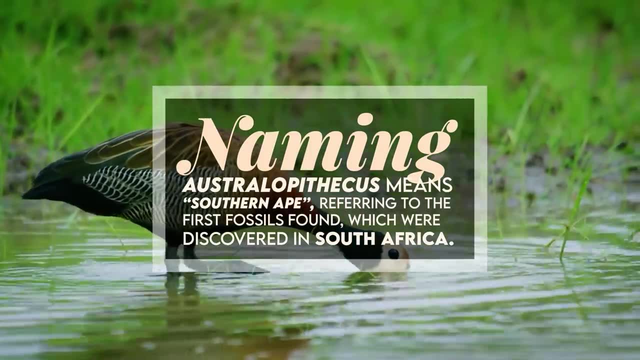 culture Addrup escaped Home accreditation. http//t авt apologiesch. Australopithecus. from Latin australis, meaning southern, and Greek pithecus, meaning ape. combined, meaning southern. ape refers to the first fossils found which were discovered. 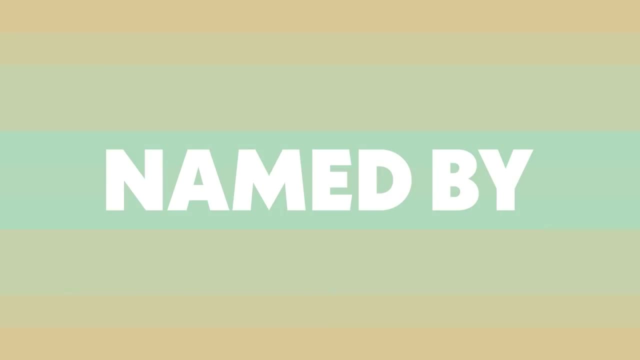 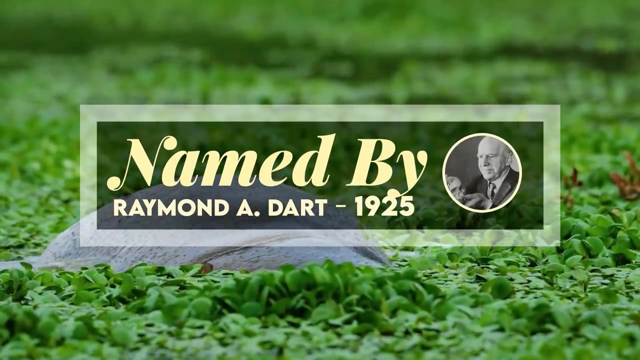 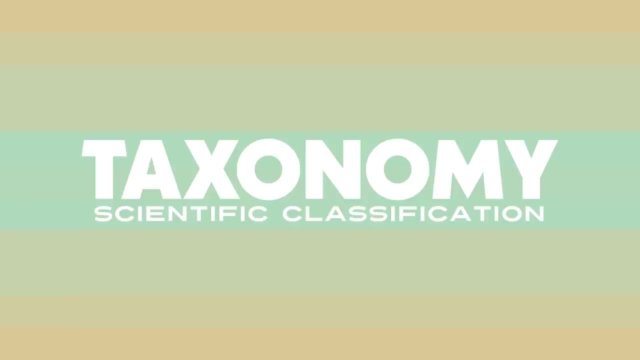 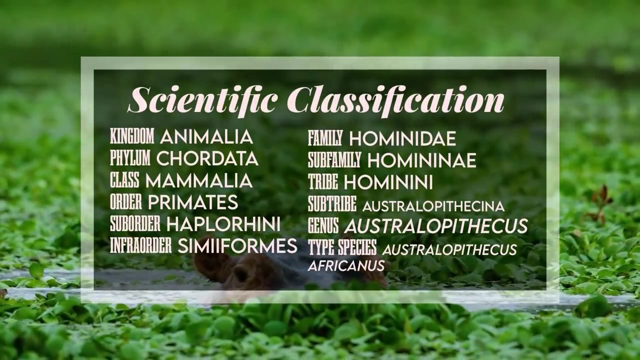 in South Africa. Australopithecus was named by Raymond Arthur Dart in 1925, with the type species Australopithecus africanus named by Dart as well in 1925.. Australopithecus belongs to the kingdom Animalia, the phylum Credata, the class Mammalia, the 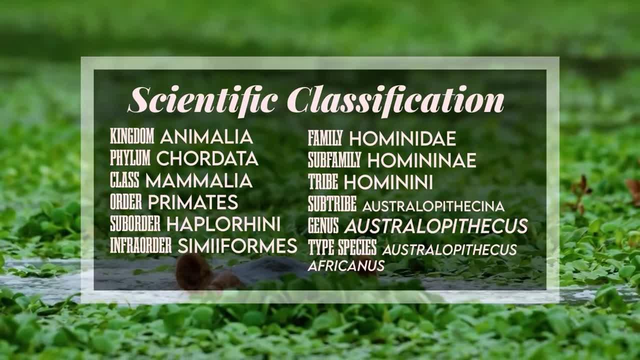 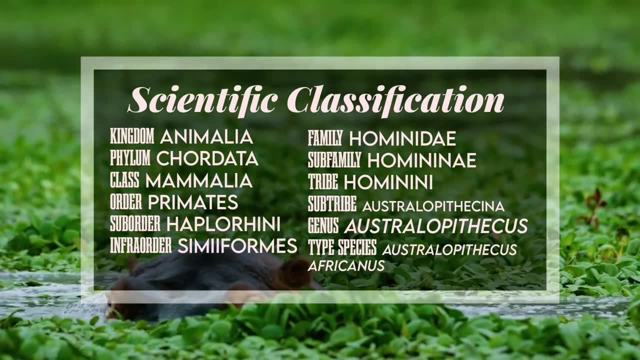 order: Primates, the suborder Haplorhini, the infraorder Semiformes, the family Hominidae, the subfamily Hominidae, the tribe Hominidae, the sub-tribe Australopithecina, the genus. 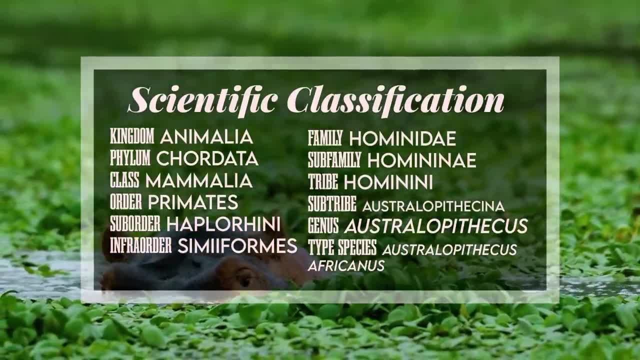 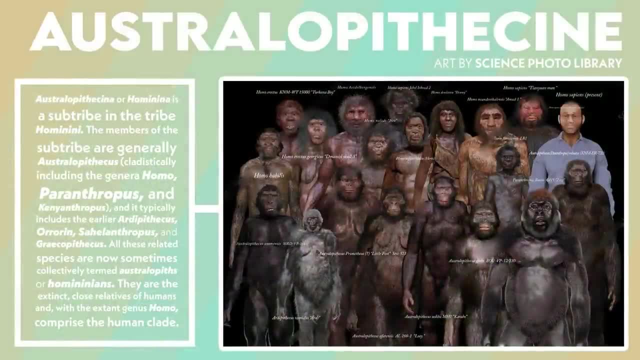 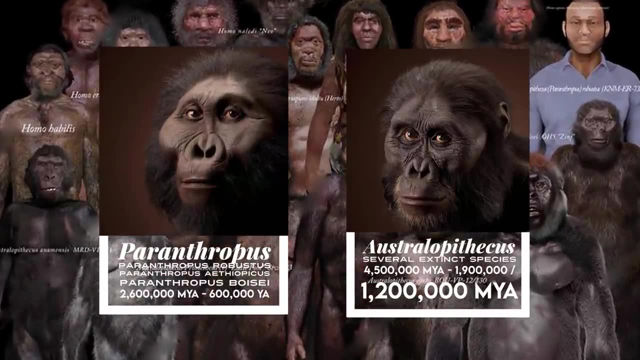 Australopithecus and the type species Australopithecus africanus. The general term Australopithecine refers to members of the genus Australopithecus, while also including the genus Paranthropus dated to 2.3 to 1.2 million years ago, which comprises: 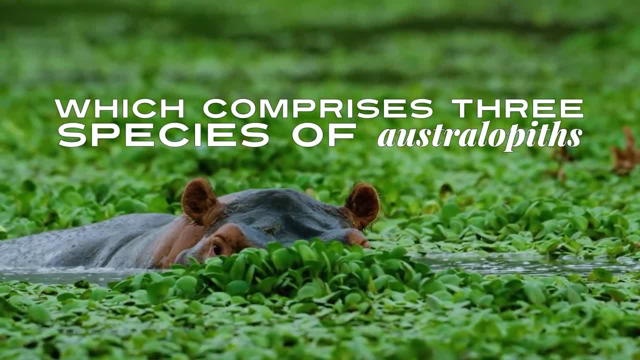 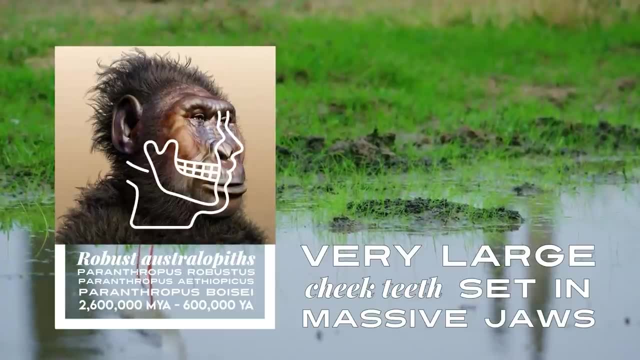 three species of australopiths, collectively known as the robust because of their very large cheek teeth set in massive jaws. Non-Australopithecine members of the human lineage, or hominids, include Salanthropus chidensis, dated to 7 to 6 million years ago. 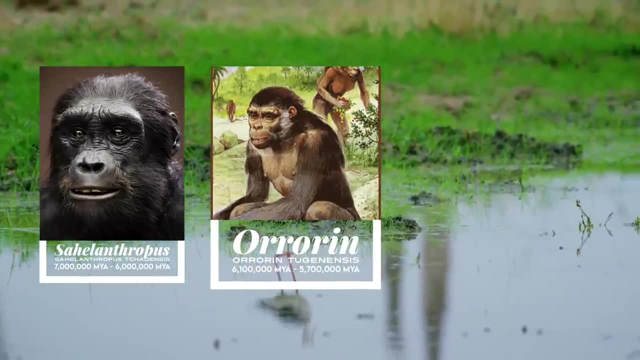 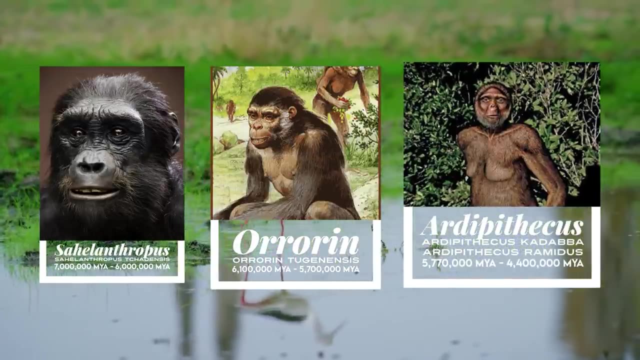 Ororhynchus genensis dated to 6 million years ago, Ardipithecus cadaver dated to 5.8 to 5.2 million years ago And Ardipithecus ramidus dated to 5.8 to 4.4 million years ago. That is, pre-Australopithecus species that are considered to be ancient humans, and one additional species of early human Canyanthropus, platyops, dated to 3.5 million years ago. Australopiths were bipedal apes that existed in the ancient world. 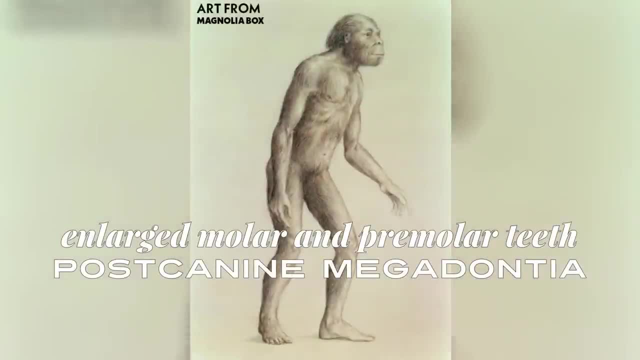 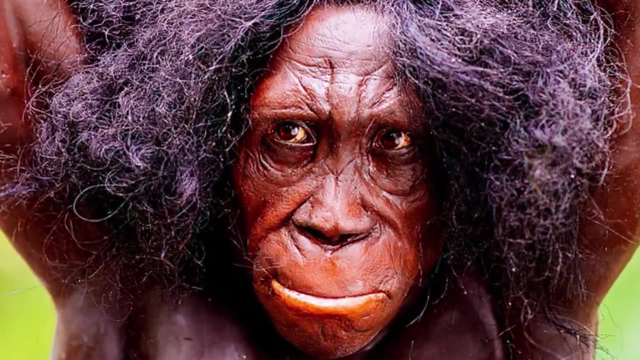 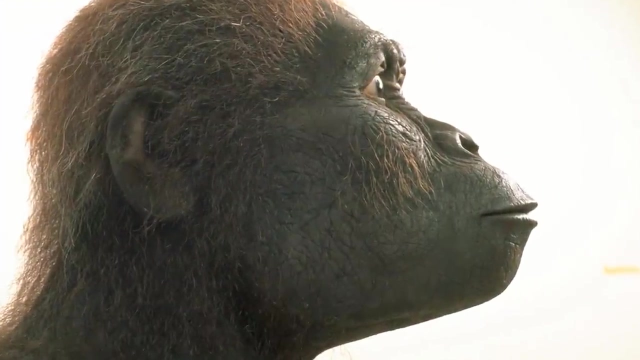 They were exhibited in large molar and premolar teeth or post-canine megadontia and other associated modifications to their feeding apparatuses. Dietary adaptations clearly played an important role in shaping their evolutionary history. They are also distinguished by their lack of derived features typically associated with. 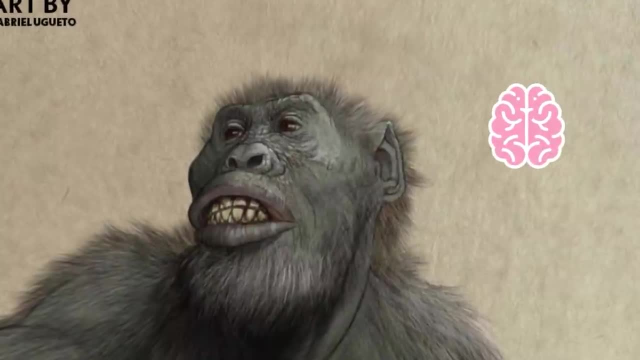 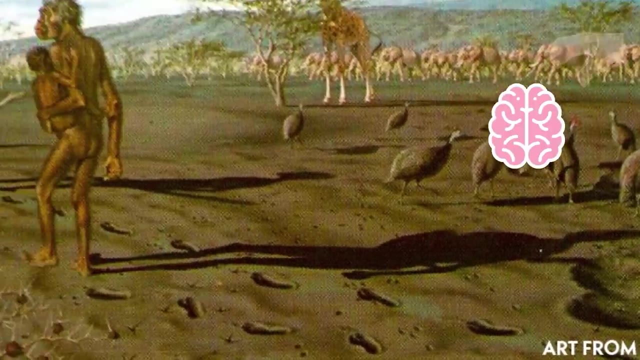 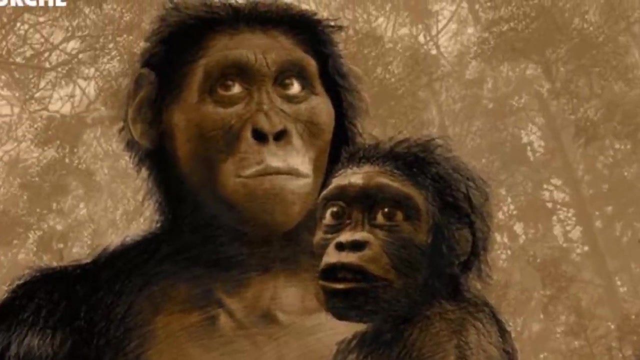 the genus Homo like a large brain, a broad complement of adaptations for manual dexterity and advanced tool use. Nonetheless, Homo is almost generally descended from an australopith ancestor, so at least one or some australopiths belong directly to the human lineage. 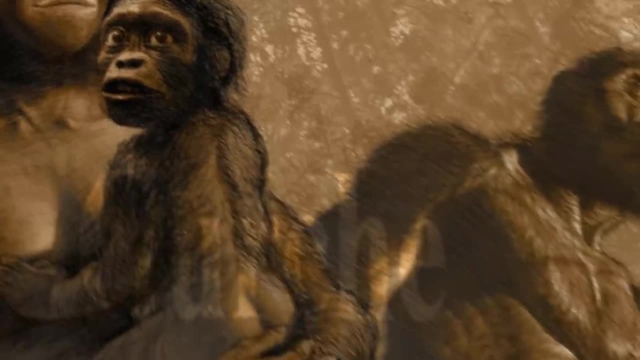 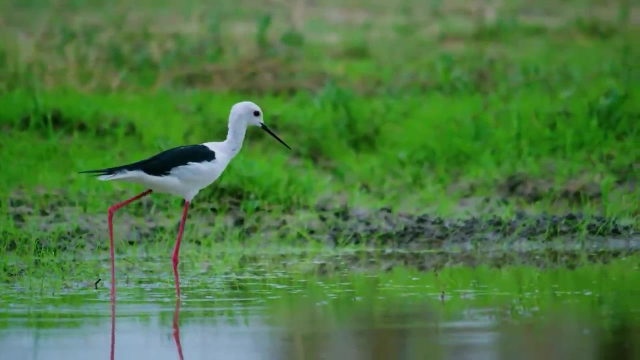 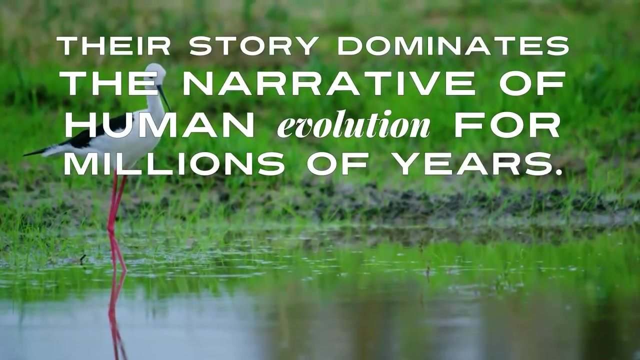 Regardless, australopiths had a rich evolutionary history deserving of study and dependent of questions about their direct ancestry. They were diverse, geographically widespread and anatomically derived. They lived through periods of pronounced climate change and their story dominates the narrative. 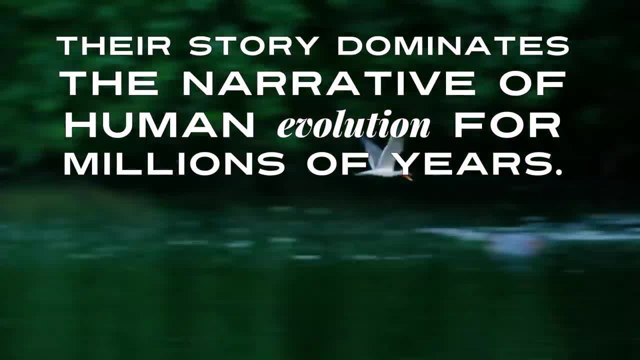 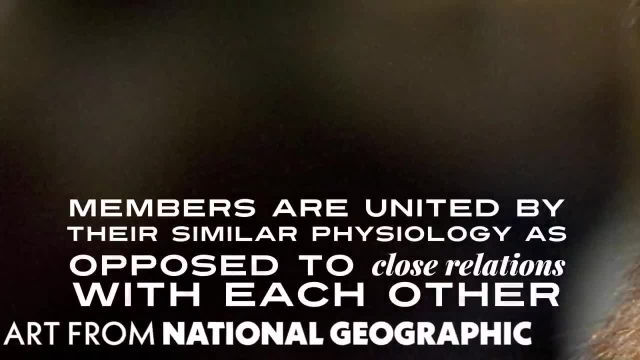 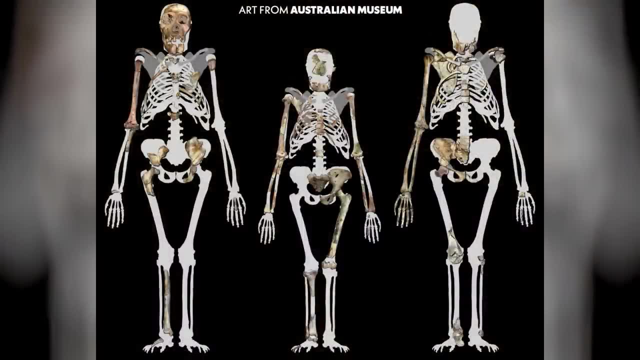 of human evolution for millions of years. The genus Australopithecus is considered to be a great taxon whose members are united by their similar physiology, as opposed to close relations with each other over all their hominid genera. It is considered the ancestor of Homo Kenyanthropus and Paranthropus and, as such, is paraphyletic. 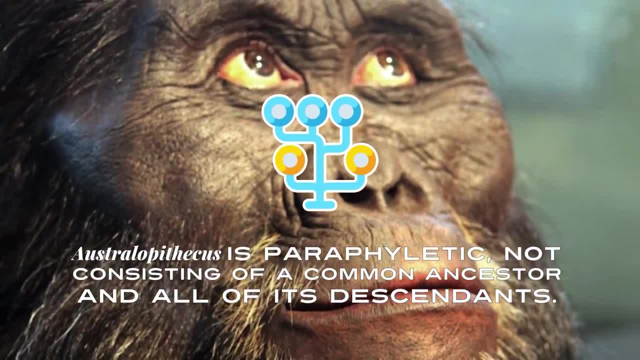 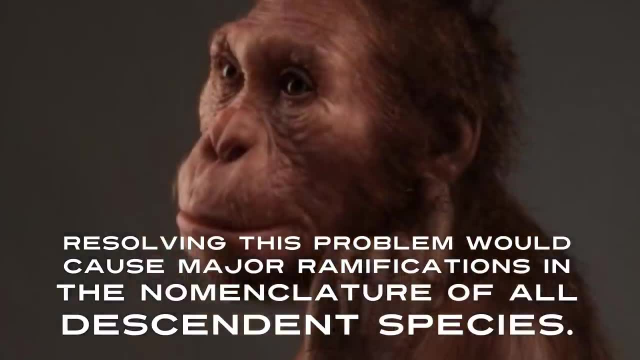 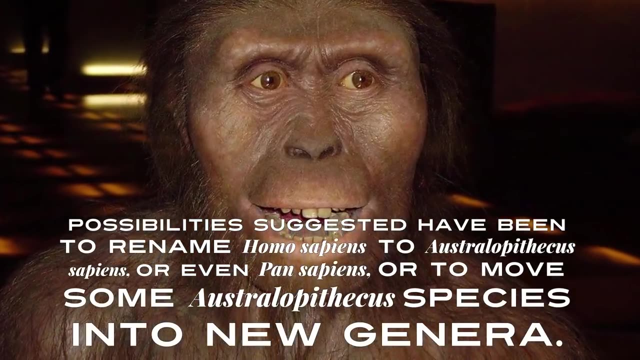 not consisting of a common ancestor and all of its descendants, For solving this problem would cause major ramifications in the nomenclature of all descendants' species. Possibilities suggested have been to rename Homo sapiens to Australopithecus sapiens or even Pan-sapiens, or to move some Australopithecus species into new genera. 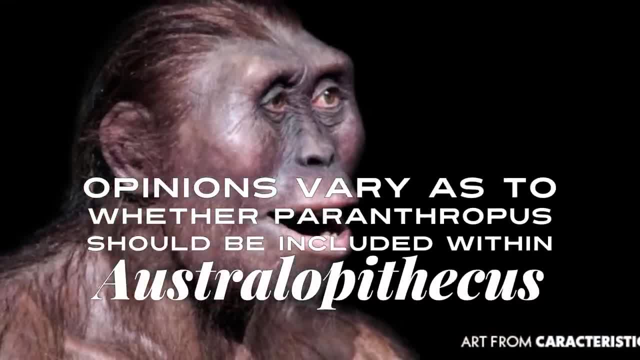 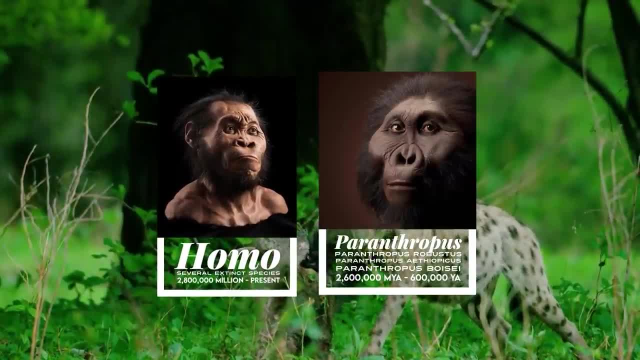 Opinions vary as to whether Paranthropus should be included within Australopithecus, and Paranthropus is suggested, along with Homo, to have developed this part of a clade within Australopithecus africanus as its basal root. 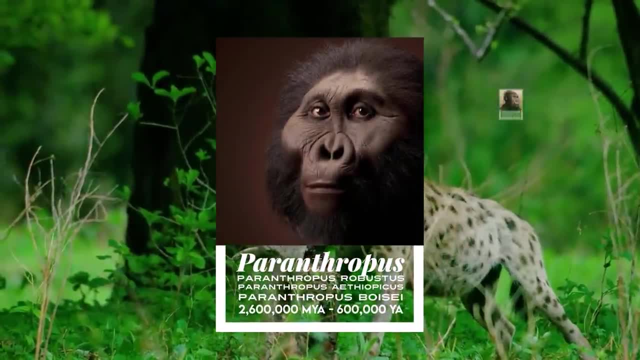 The members of Paranthropus appear to have a distinct genus. The genus Australopithecus is considered to be a great taxon as opposed to a common ancestor. It is unclear to have a distinct robustness compared to the Grassalostralopiths, but it 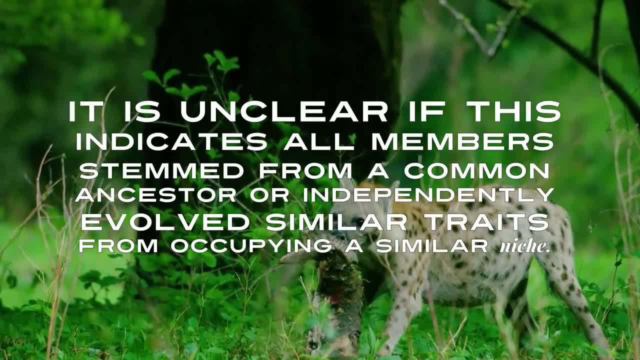 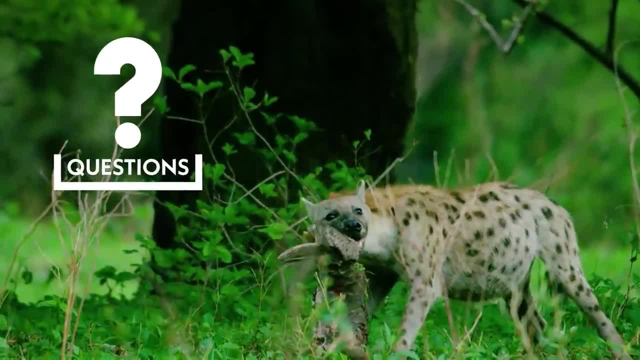 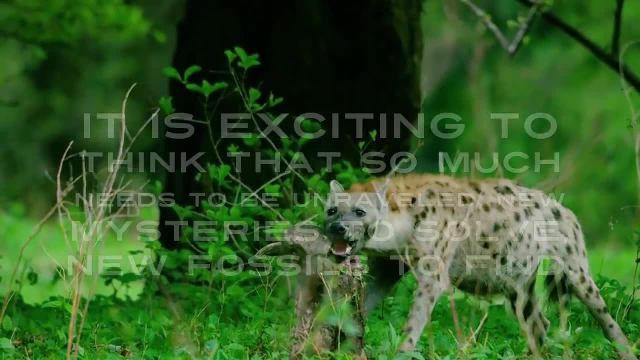 is unclear. this indicates all members stem from a common ancestor or independently evolved similar traits from occupying a similar niche. These questions are what paleoanthropologists continue to ponder and simply show how challenging it is to reconstruct their past. It is exciting to think that so much needs to be unraveled new mysteries to solve. 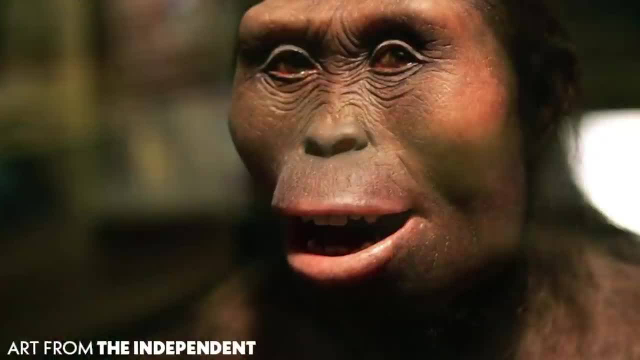 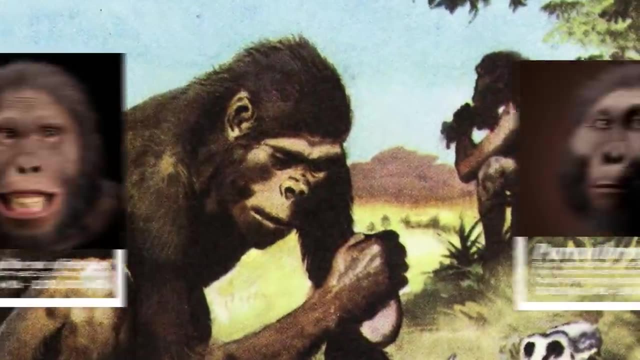 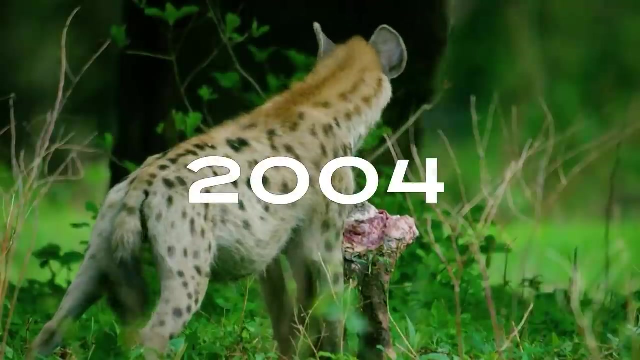 new fossils to find Conclusion. In 2002, and again in 2007,, Celia Gonde and colleagues suggested that Australopithecus africanus be moved to Paranthropus On the basis of craniodental evidence. Strait and Green in 2004 suggested that Australopithecus 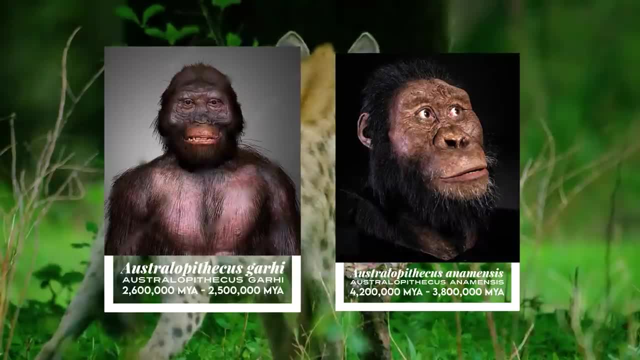 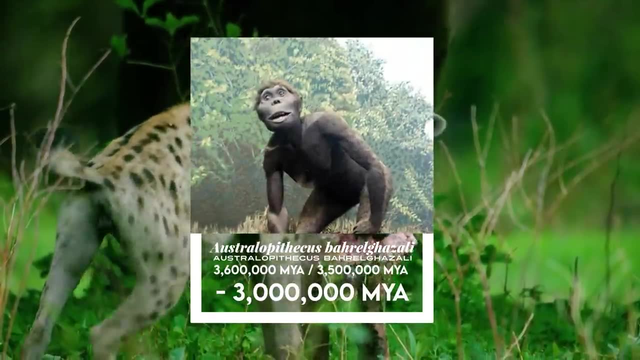 anamensis and Australopithecus gari should be assigned to new genera. It is debated whether or not Australopithecus barogazali should be considered simply a western variant of Australopithecus afarensis instead of a separate species. 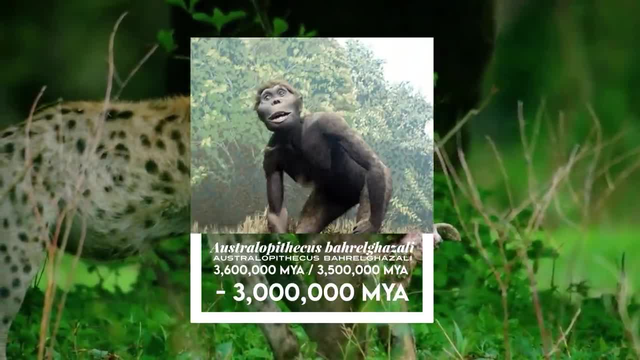 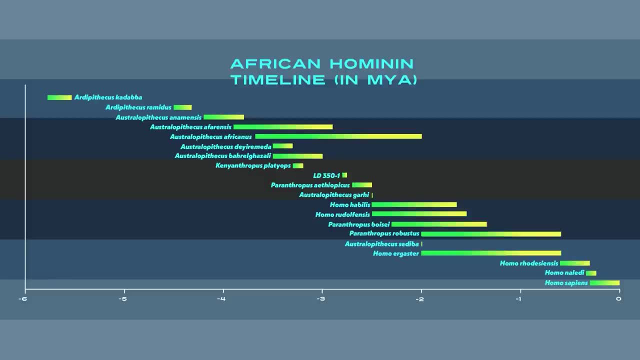 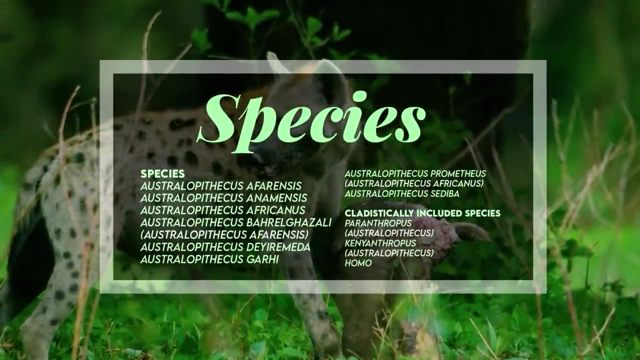 The results of this study show that Australopithecus anamensis and Australopithecus gari should be assigned to new genera. Here is an African hominin timeline in millions of years ago. Species include Australopithecus afarensis, Anamensis, africanus, Barogazali, possibly. 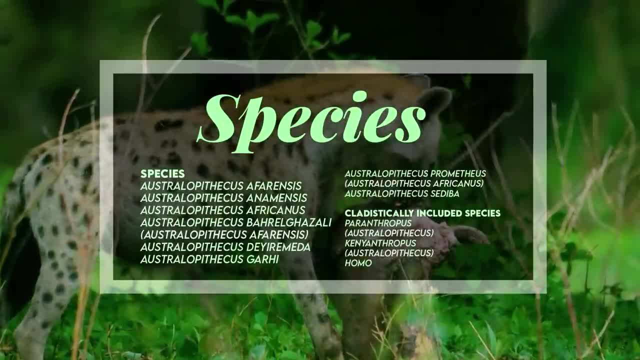 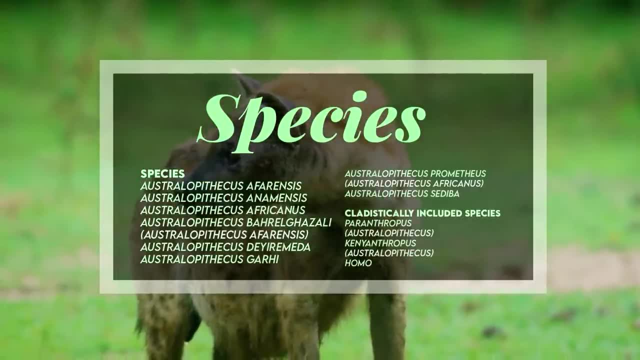 Australopithecus afarensis, Dejiramida, Gari, Prometheus, possibly Australopithecus africanus, Sediva, etc. 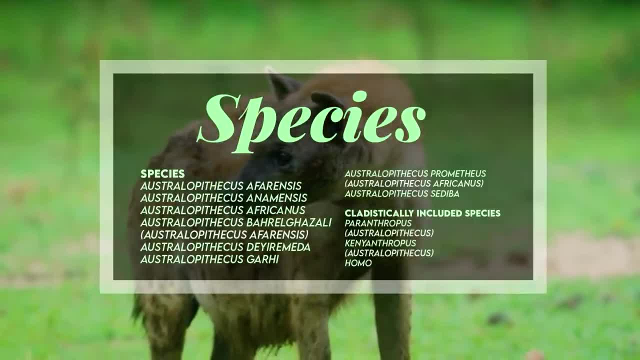 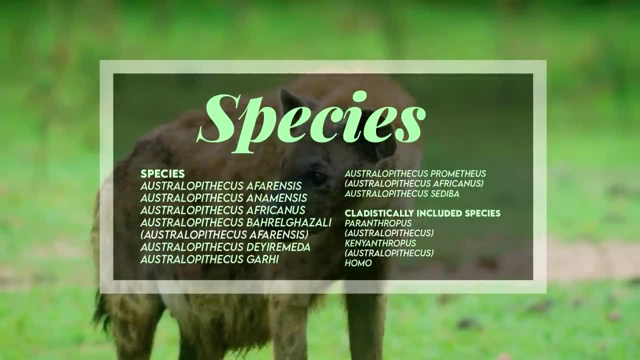 . . . . . . . . . . . Species classically excluded but cladistically included Pentherophis possibly Australopithecus, Kinyanthropus possibly Australopithecus as well, and Homo. �� Unscripted 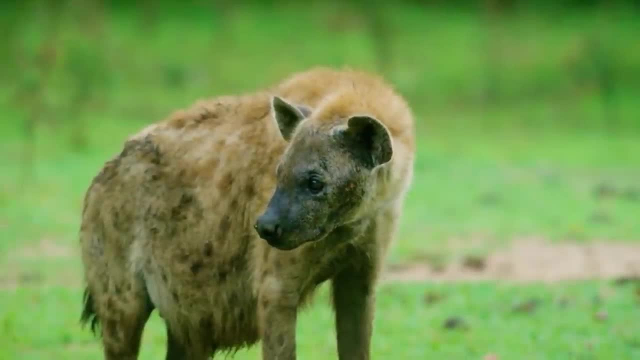 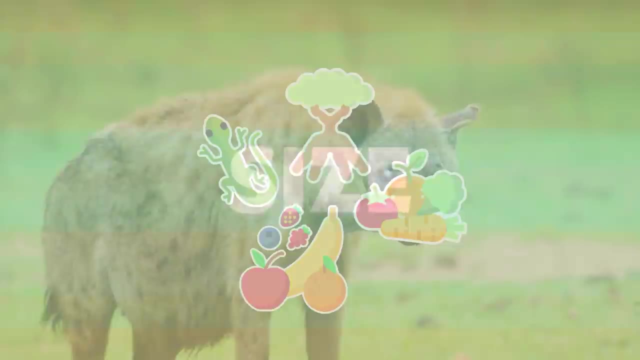 Australopithecus species are considered to have mainly eaten fruit, vegetables and tuber and perhaps easy to catch animals like small lizards. CHRISTTOPH toner boxing Menopause. Most species of Australopithecus were diminutive and grasa typically standing through feet. 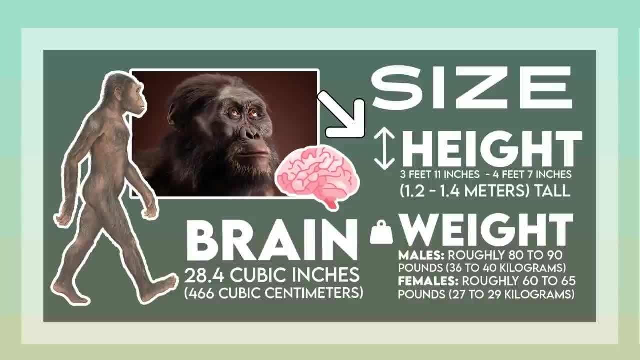 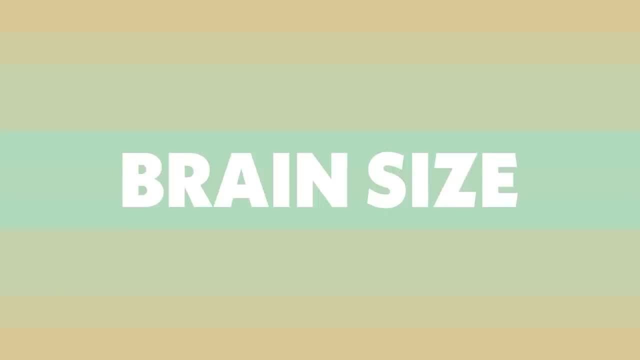 feet being rubbed off, orauen's beating sounds and☆ concerts, wood进掉. 3 feet 11 inches to 4 feet 7 inches, or 1.2 to 1.4 meters tall. The brains of most species of Australopithecus were roughly 35% the size of a modern human. 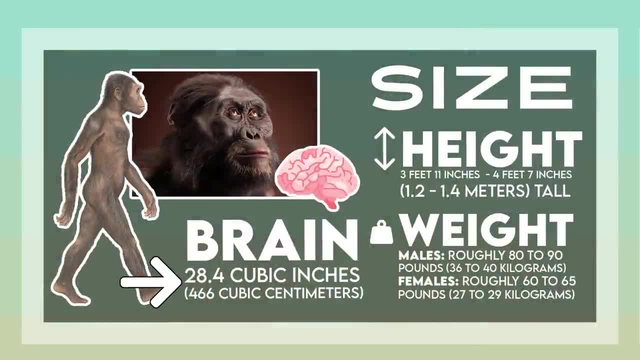 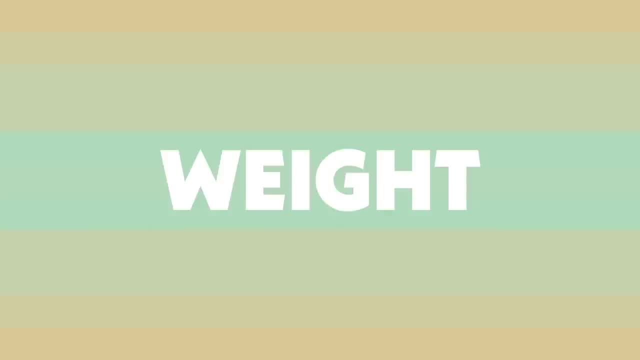 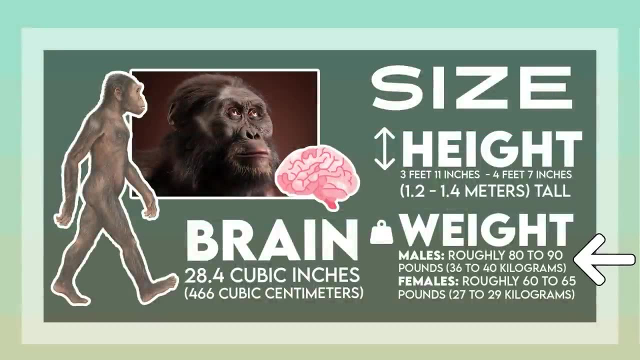 brain, with an endocranial volume average of 28.4 cubic inches or 466 cubic centimeters. Several Australopithecus species weighed roughly 80 to 90 pounds, or 36 to 40 kilograms as male, and roughly 60 to 65 pounds or 27 to 29 kilograms as females. 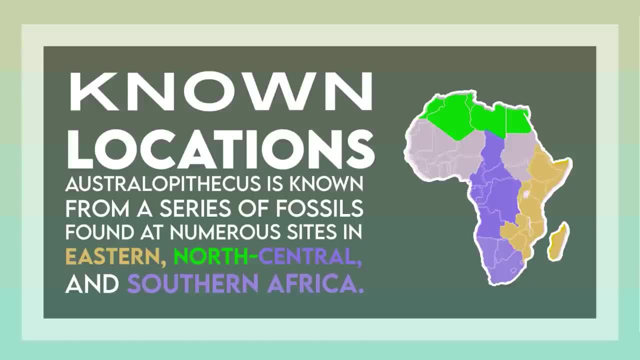 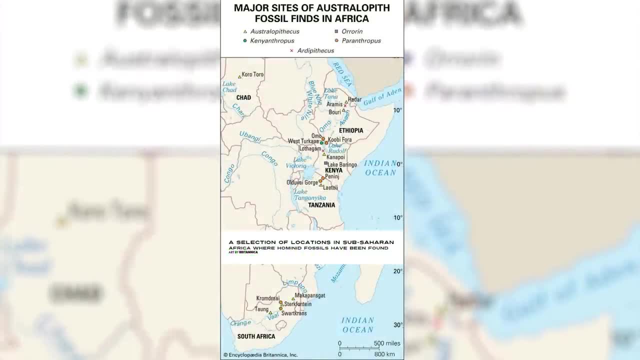 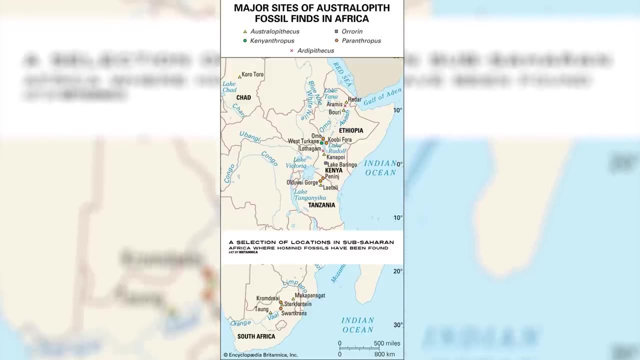 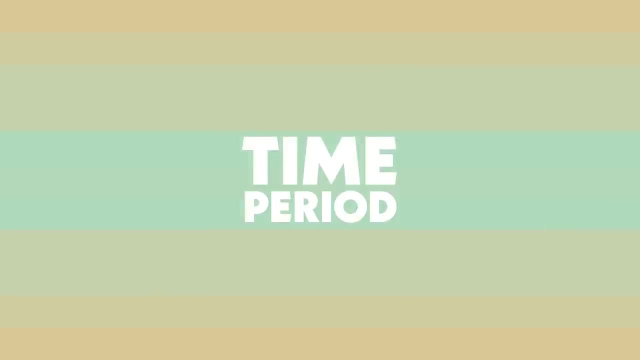 Australopithecus is known from a series of fossils found in numerous sites in eastern, north-central and southern Africa. Here are a selection of locations in sub-Saharan Africa where hominid fossils have been found. Here are approximate time ranges of sites yielding Australopithecus fossils: 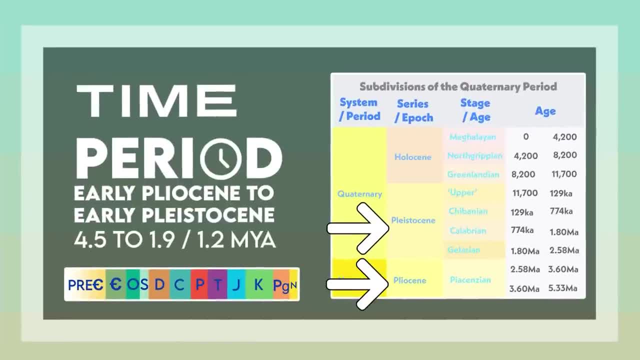 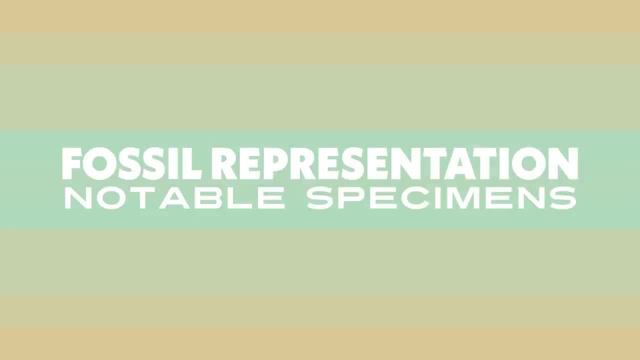 Australopithecus lived during the early Pliocene to early Pleistocene, 4.5 to 1.9 or 1.2 million years ago. The first species to be identified as Australopithecus received that name in 1925.. 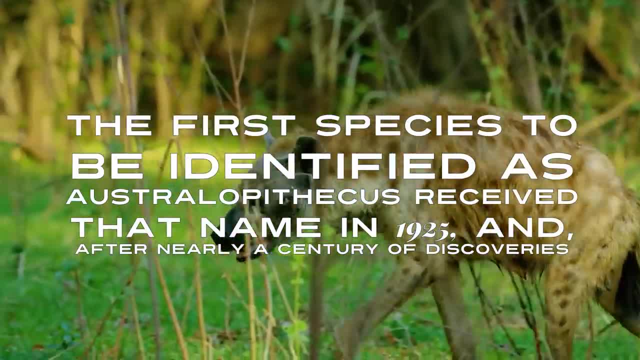 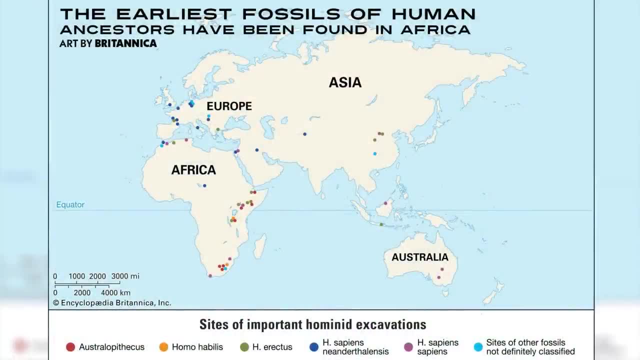 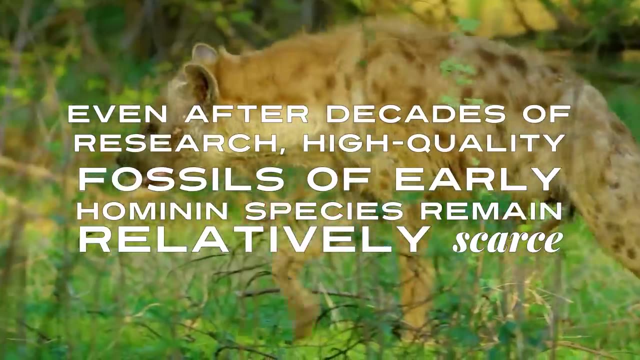 And After nearly a century of discoveries, paleoanthropologists are able to draw upon a fairly rich collection of fossil hominin specimens from Africa. However, even after decades of research, high quality fossils of early hominin species remain relatively scarce, and thus their continued discovery has become even more vital to the 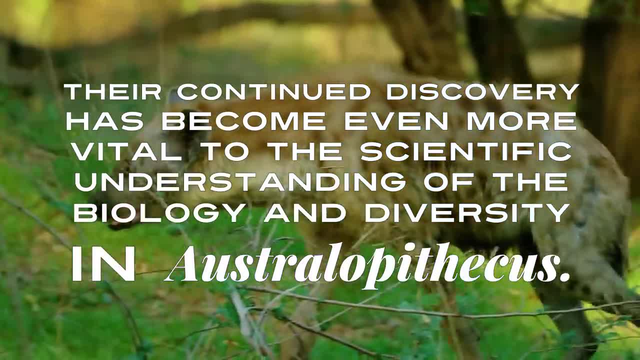 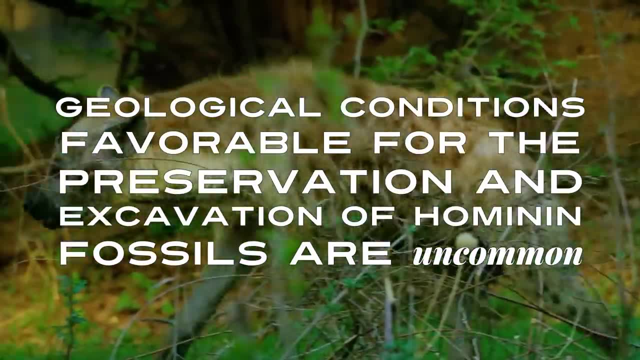 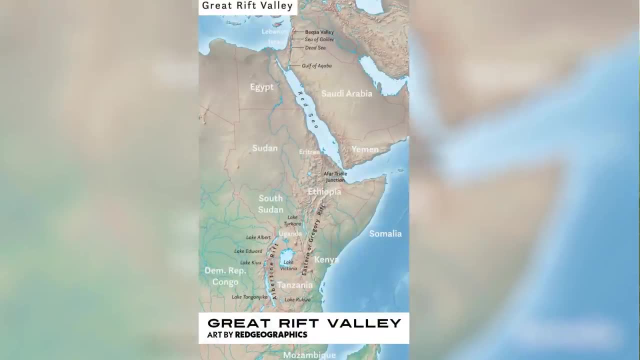 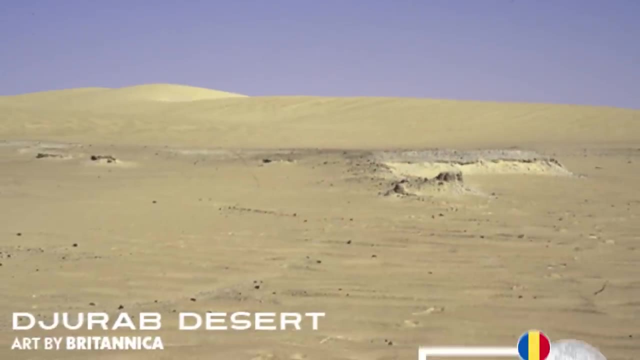 scientific understanding of the biology and diversity in Australopithecus. Geological Conditions Favorable for the preservation and excavation of hominin fossils are uncommon, being largely restricted to the Great Rift Valley in eastern Africa, the limestone caves of South Africa and sedimentary deposits of the Chad Basin and Jerab Desert, an arid region in central. 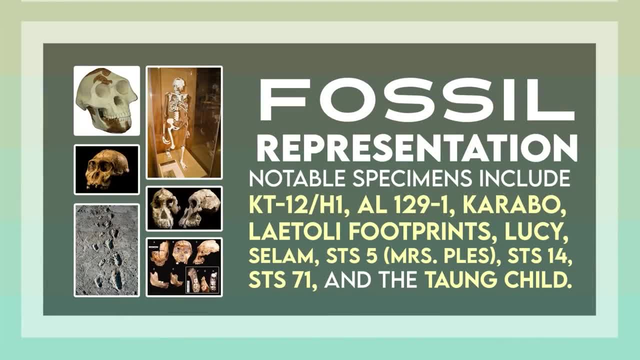 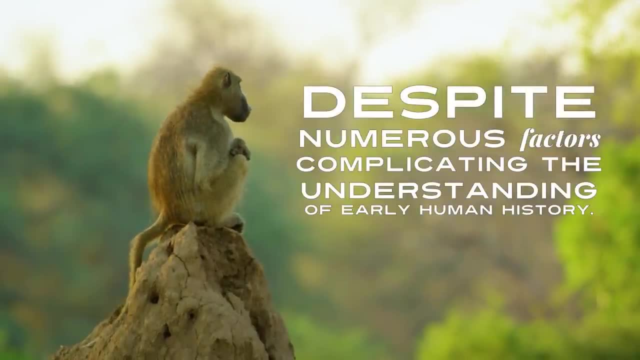 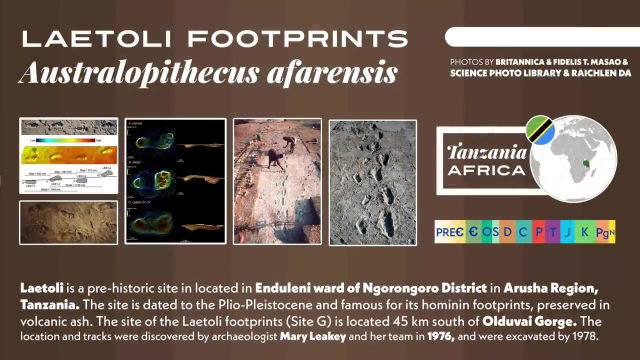 Chai. There are a great deal of fossil finds that are, unfortunately, forever lost in the past. We must therefore reconstruct early hominins with the finds we have, despite numerous factors complicating the understanding of early human history Specimens. Notable specimens include KT12H1, AL129-1, Caraba, the Laetoli footprints, Lucy Solan. 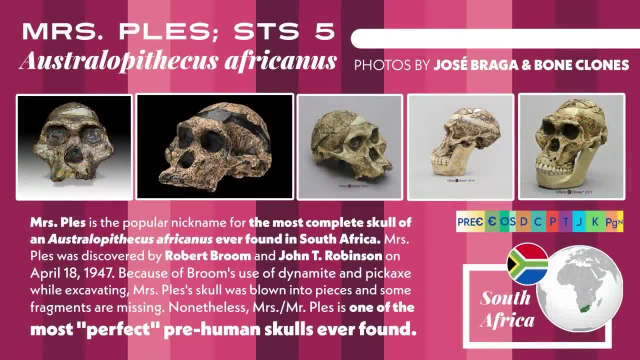 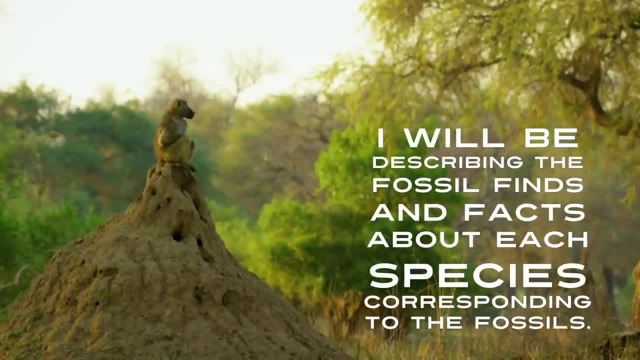 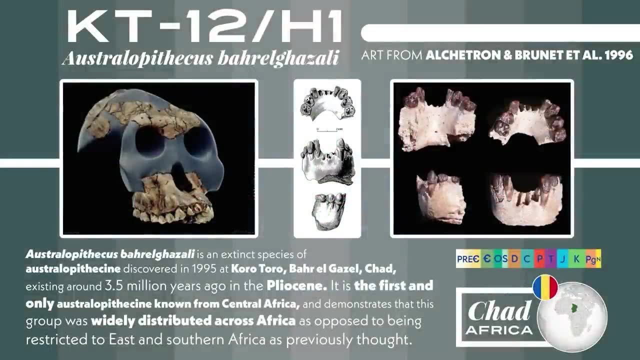 STS5 or, Mrs Ples, STS14,, STS71, and the Tongue Child. In this section I will be describing the fossil finds and facts about each species corresponding to the fossils Facts. KT12H1 is an Australopithecus barragazali mandibular fragment discovered in 1995 in 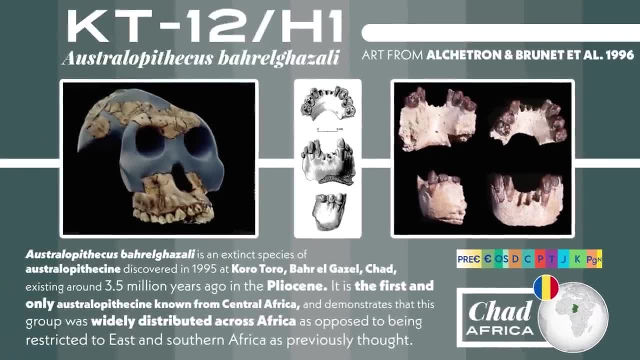 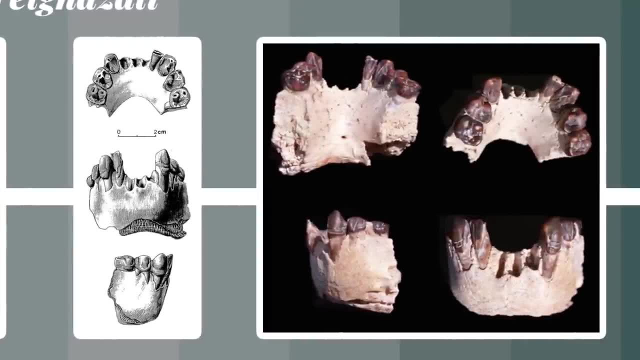 Sahara, Chad. Australopithecus barragazali is an australopithecine discovered in Corotoro Barragazal, Chad, hence the name- existing around 3.5 million years ago in the Pliocene. 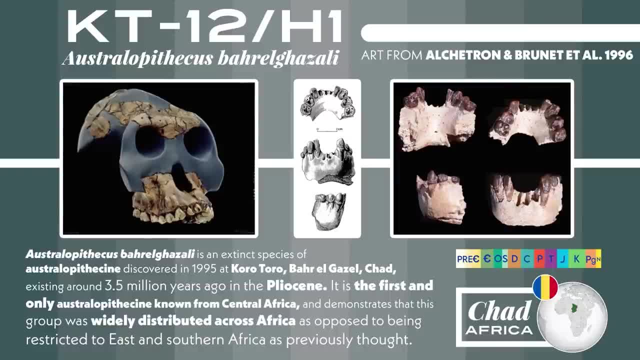 It is the first and only australopithecine known from Central Africa and demonstrates that this group was widely distributed across Africa. The name is also known as the Pliocene. The Pliocene is the first and only australopithecine known from Central Africa and demonstrates that this group was widely distributed across Africa. 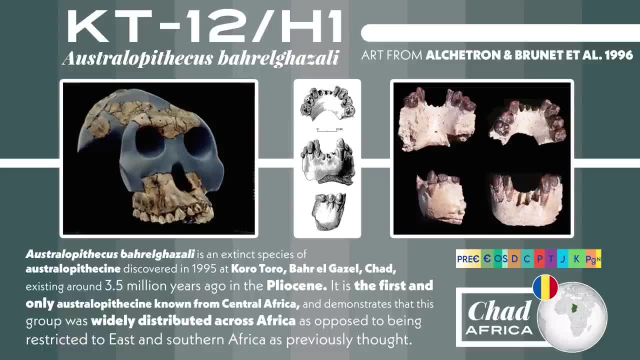 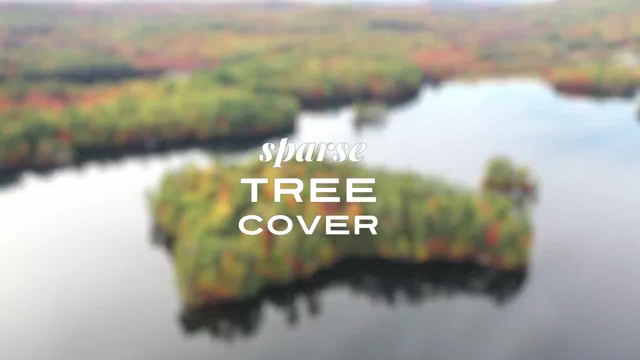 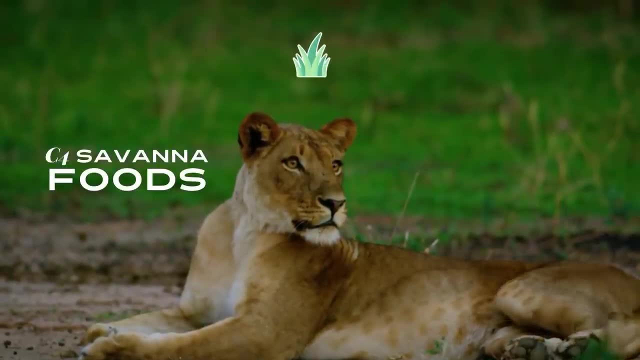 Rather than being restricted to East and Southern Africa. as previously thought, the specimens inhabited a lakeside grassland environment with sparse tree cover, possibly similar to the modern Okobanjo Delta, and similarly predominantly ate C4 savanna foods like grasses sedges. 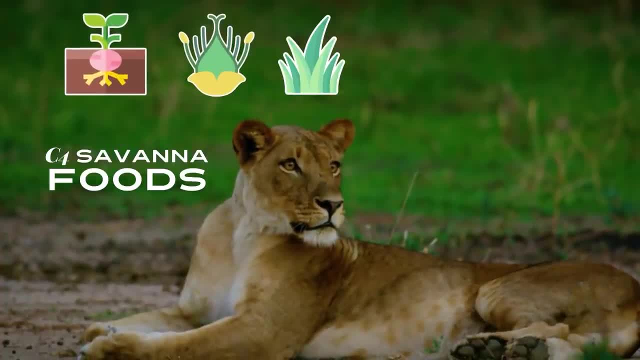 storage organs or rhizomes and, to a lesser extent, also C3. forest foods like fruits, flowers, pods or insects. Facts: KT12H1 is an australopithecine known from Central Africa, hence the name existing. 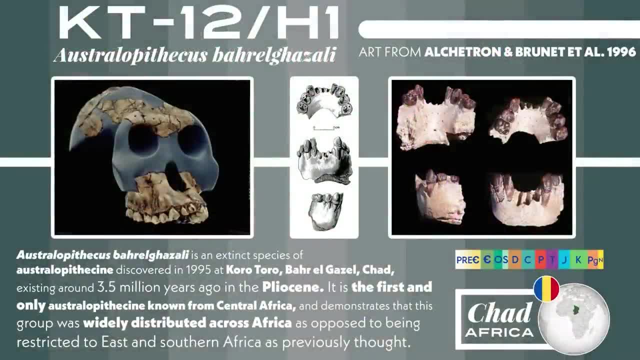 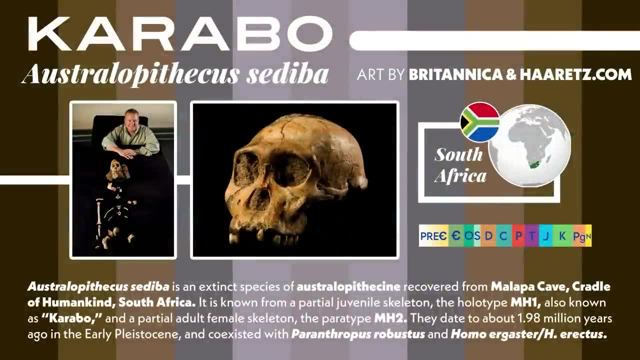 around 3.5 million years ago in the Pliocene. Nonetheless, the teeth seem ill-equipped to process C4 plants, so its true diet is unclear. Caerobo Chiafensis- Caerobo, a juvenile male Australopithecus. 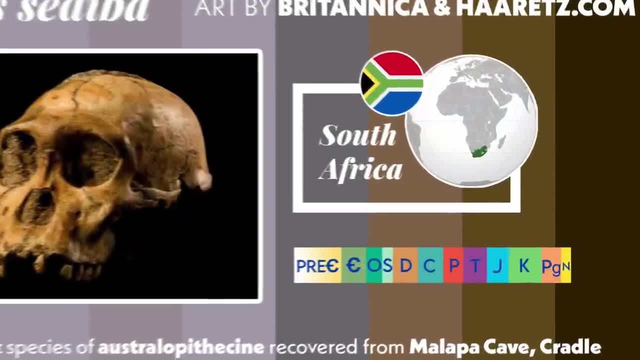 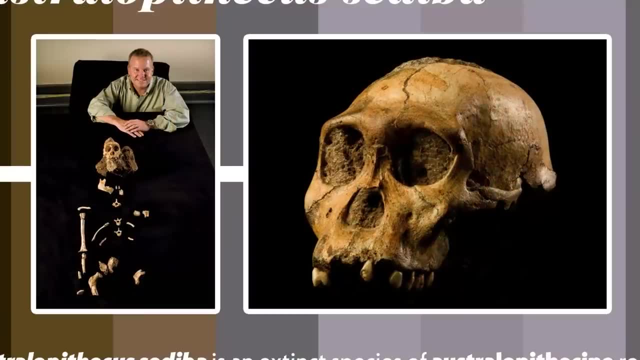 sediba was discovered in South Africa. Australopithecus sediba was an australopithecine recovered from Malapa Cave, Cradle of Humankind, South Africa. Specimens date to about 1.98 billion years ago in the early Pleistocene and coexisted. 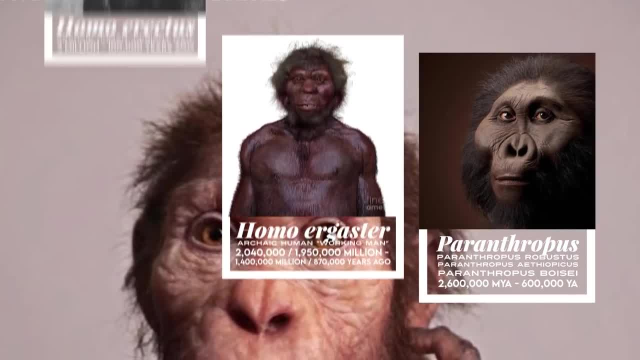 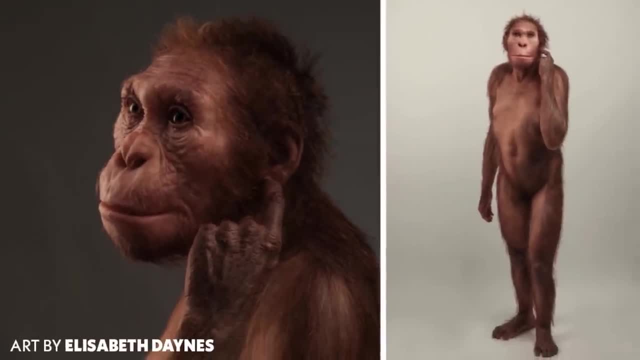 with Paranthropus robustus robustus and Homo ergaster or Homo erectus. The teeth of Australopithecus sediba are quite small for an australopithecine. Like other australopithecine, Australopithecus sediba. 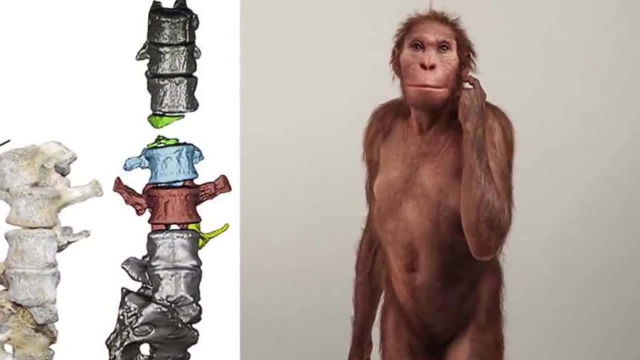 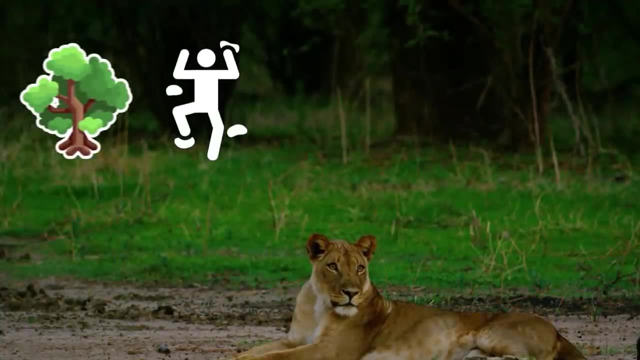 is thought to have had a narrow and ape-like upper chest, but a broad and human-like lower chest, Like other australopithecines. the arm anatomy seems to suggest a degree of climbing and arboreal behavior. The pelvis indicates that Australopithecus sediba was capable of. 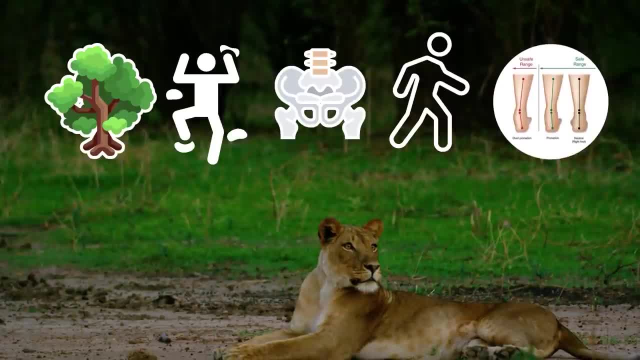 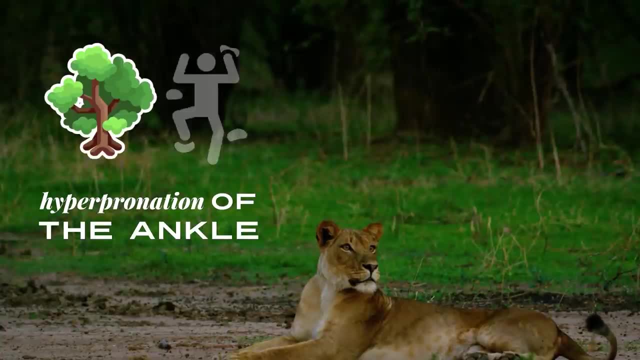 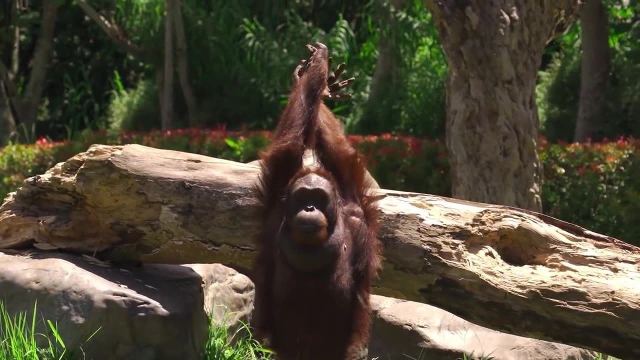 a human-like stride, but the foot points to a peculiar gait not demonstrated in any other hominin, involving hyperpronation of the ankle and, resultantly, rotating the leg inwards while pushing off. This group of adaptations may represent a compromise between habitual 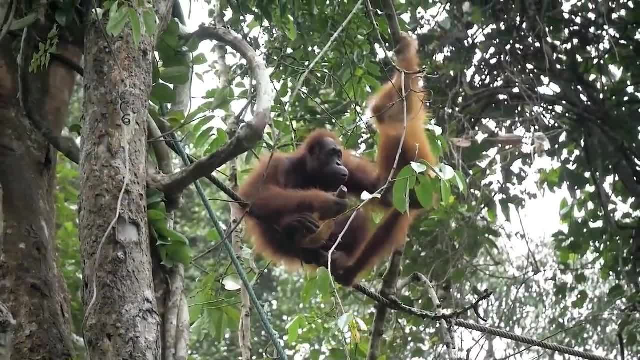 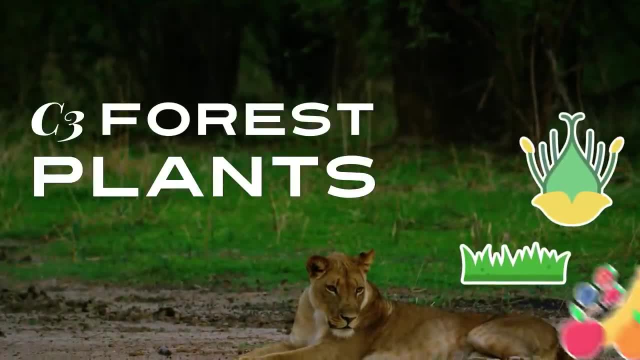 bipedalism and arboreality. Australopithecus sediba seems to have eaten only C3 forest plants, like some grasses and sedges, fruits, leaves and bark. This trauma is often referred to as astralopithecus sediba or astralopithecus sediba or astralopithecus. 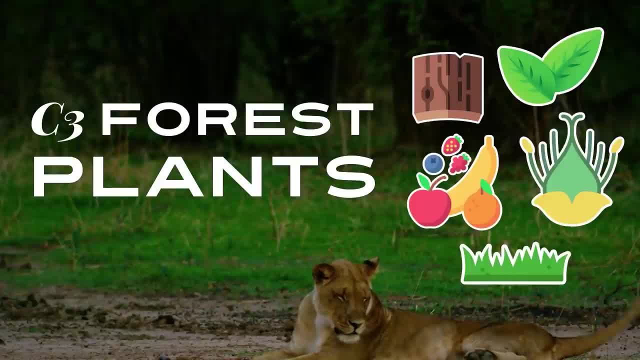 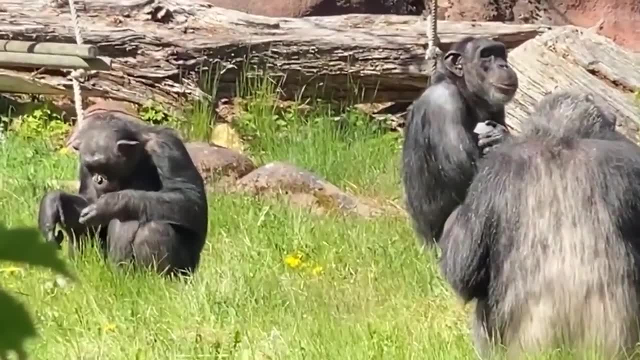 sediba. This trauma is often referred to as astralopithecus sediba or astralopithecus sediba, which strongly contrasts from other early hominins which ate a mix of C3 and abundant C4 savanna plants, but is similar to modern savanna chimpanzees. No other hominin bears. 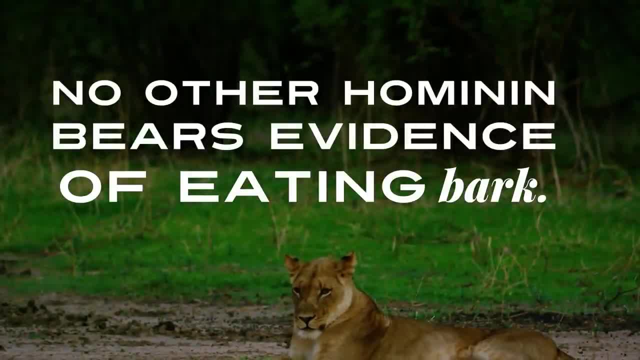 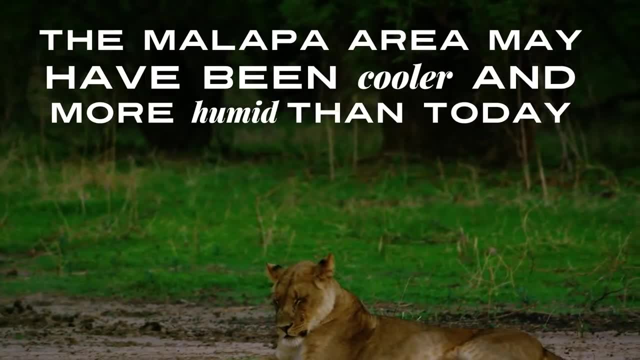 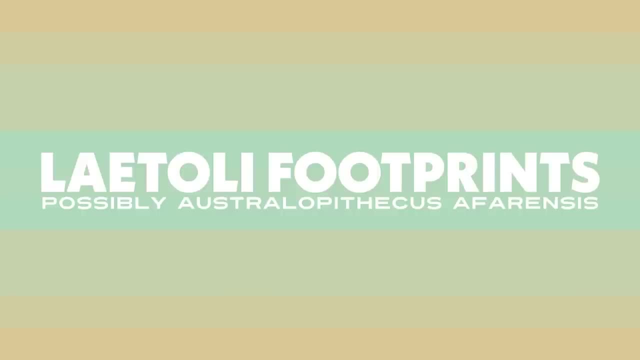 evidence of eating bark. Such a generalist diet may have allowed it to occupy a smaller home range than savanna chimps. The Malapa area may have been cooler and more humid than today, featuring close forests surrounded by more open grasslands. Laetoli Footprints. The Laetoli Footprints represent preserved 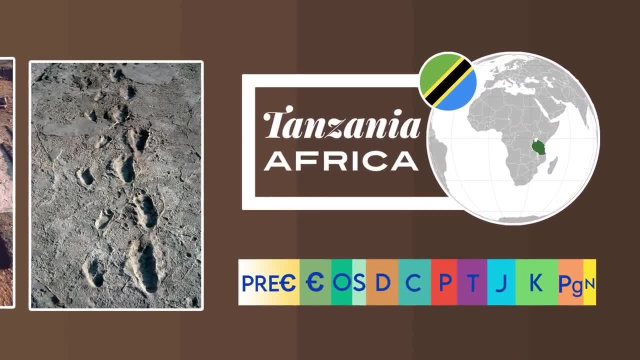 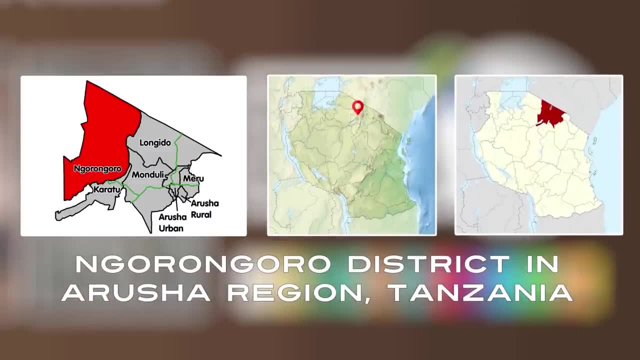 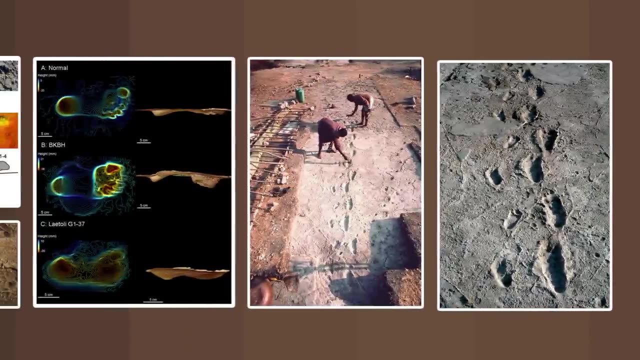 hominin footprints in Tanzania. Laetoli is a prehistoric site located in the Enduleni Ward of Ngorongoro District in Arusha Region, Tanzania. This site is dated to the Playa Pleistocene and is famous for its hominin footprints preserved in volcanic ash. The 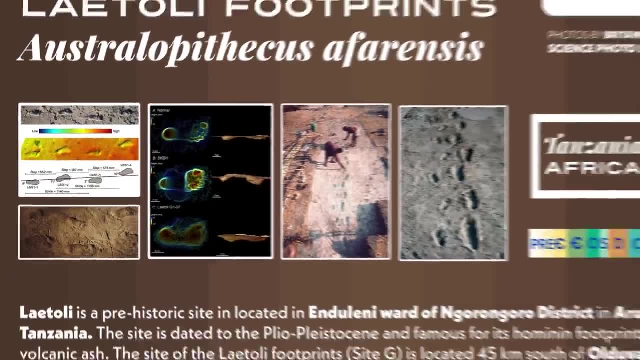 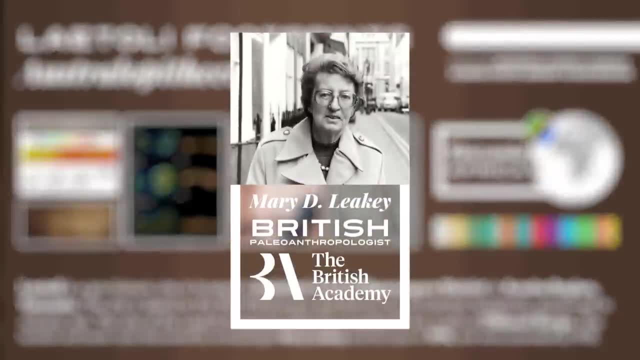 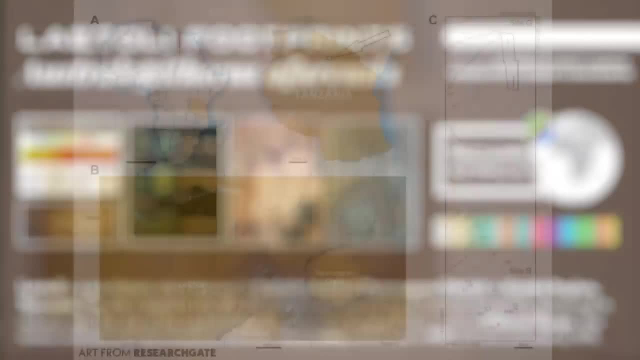 site of the Laetoli Footprints, Site G, is located 45 km south of Oldubai Gorge. The location and tracks were discovered by archaeologists Mary Leakey and her team in 1976, and were excavated by 1978.. Based on analysis of the footfall impressions, these footprints provided. 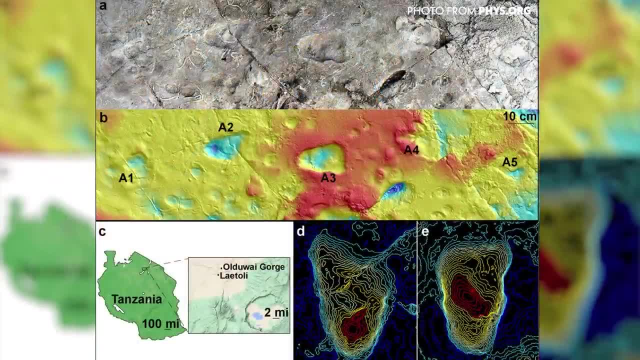 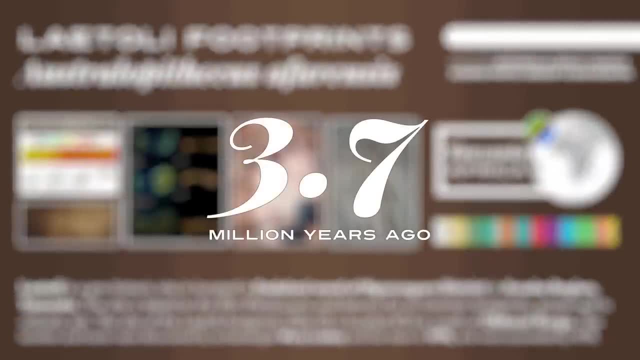 convincing evidence for the theory of bipedalism in Playa-tean hominins and received significant recognition by scientists and the public. Dated to 3.7 million years ago, they were the oldest known evidence of hominin bipedalism at that time. Subsequently, all of the footprints- 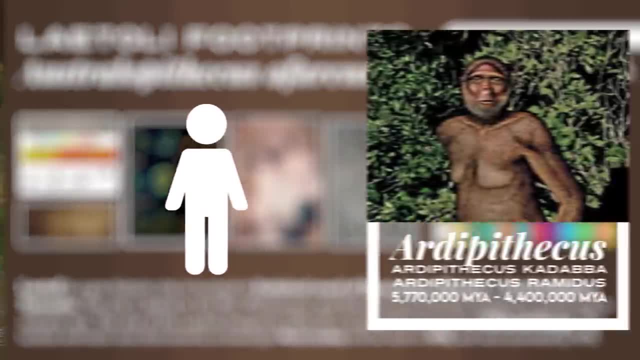 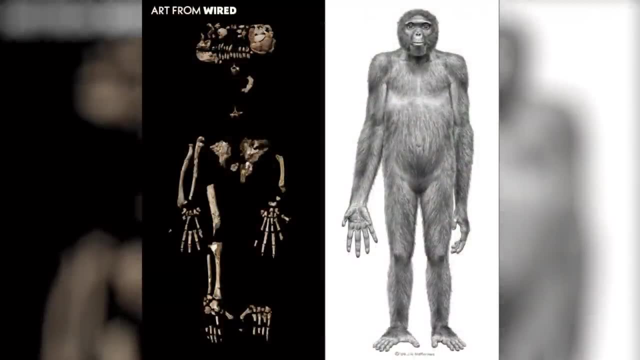 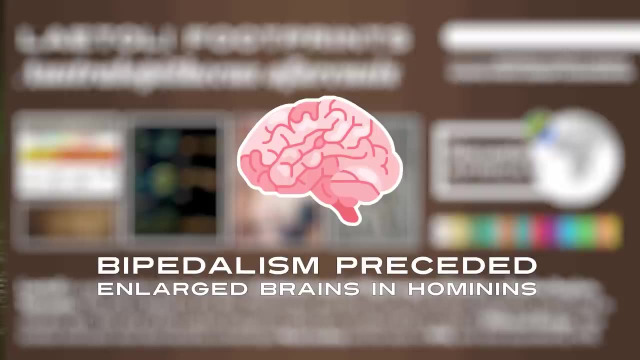 were found with features that suggest bipedalism. Analysis of the footprints and skeletal structure showed clear evidence that bipedalism preceded enlarged brains in hominins, a crucial paleoanthropological find At a species level. the identity of the hominins who made this trace is challenging. 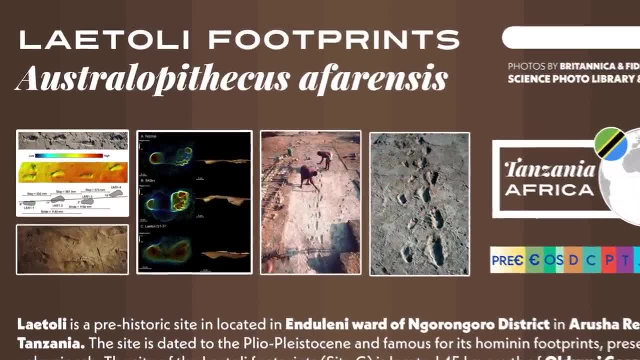 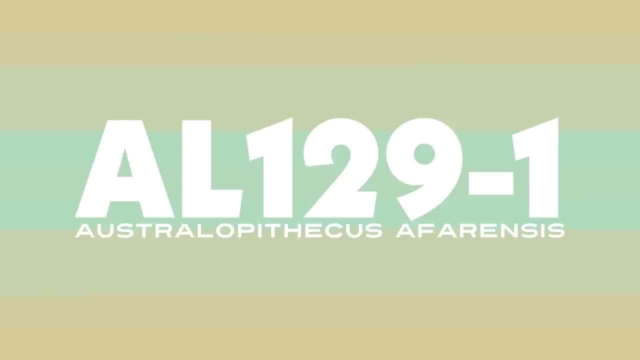 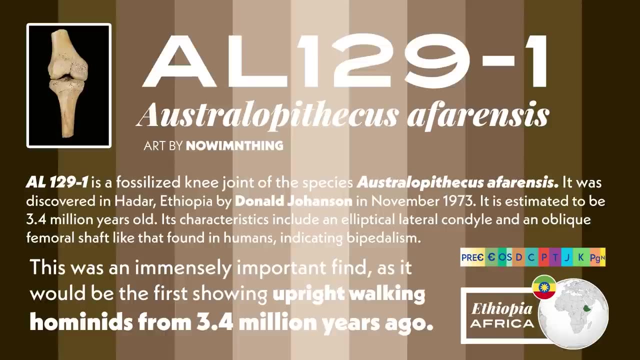 to determine precisely, with Australopithecus afarensis being the most commonly proposed species. AL 1291, an Australopithecus afarensis knee joint, was discovered in 1973 in Hadar Ethiopia. 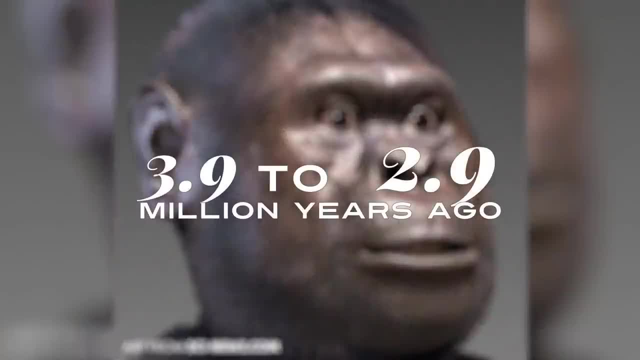 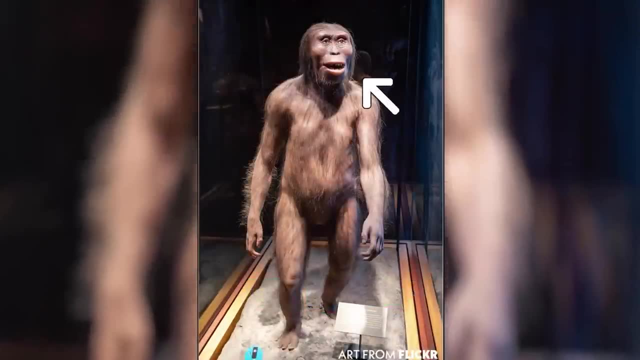 Australopithecus afarensis were australopithecines which lived from about 3.9 to 2.9 million years ago in the Pliocene of East Africa. They had a tall face, a delicate brow, ridge. 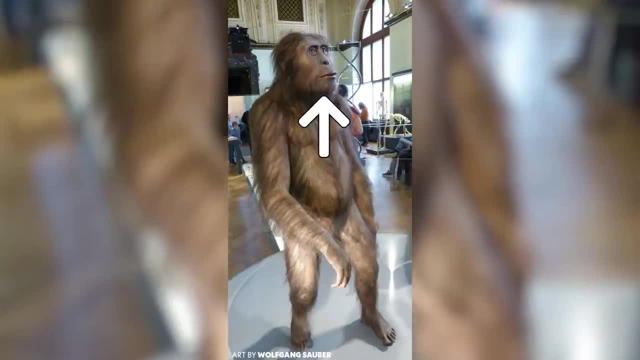 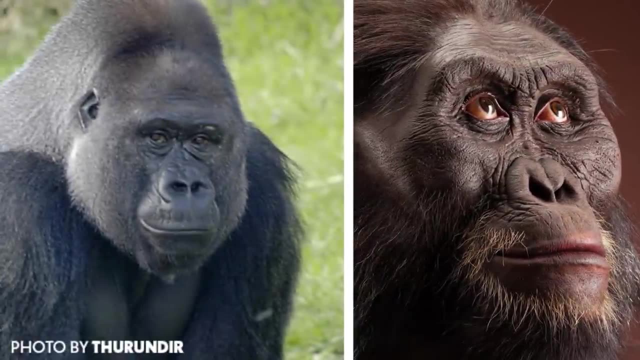 and exhibited prognathism or its jaw jutting outwards. The jawbone was quite robust, similar to that of gorillas. The leg bones, as well as the liatoli fossil trackways suggest Australopithecus afarensis. 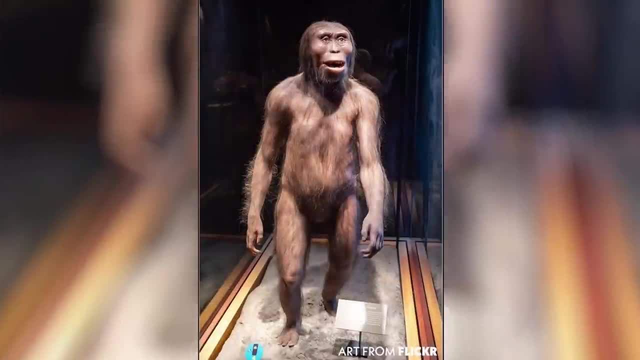 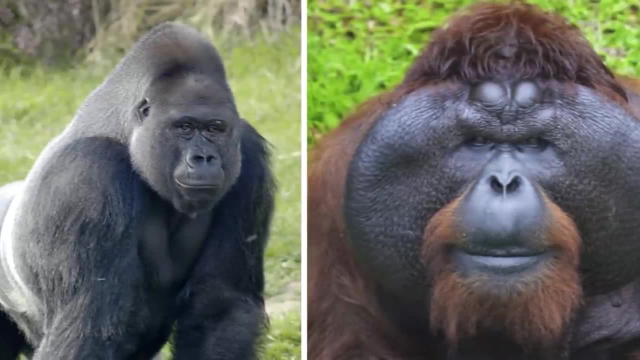 was a competent biped, though somewhat less efficient at walking than humans. The arm and shoulder bones have some similar aspects to those of orangutans and gorillas, which has variously been interpreted as either evidence of partial tree dwelling or arboreality, or 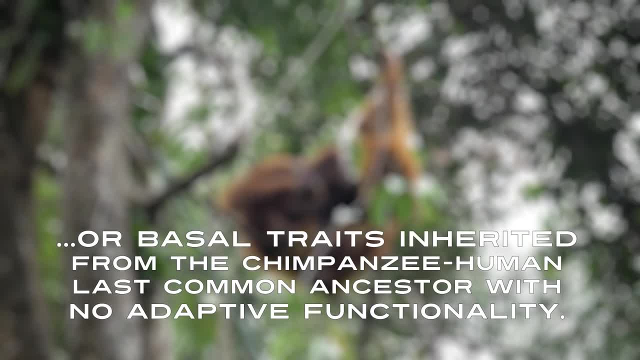 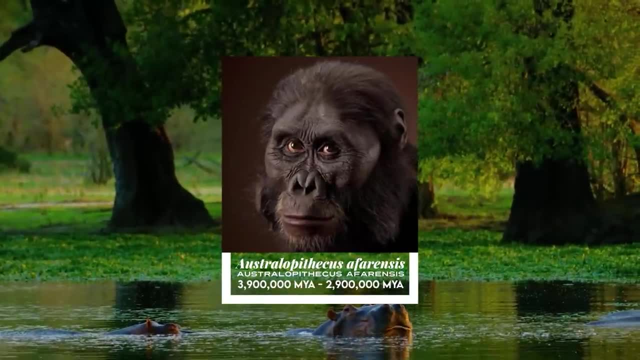 basal traits inherited from the chimpanzee human last common ancestor, with no adaptive use. AL 1291,, an Australopithecus afarensis knee joint, was discovered in 2003 in Hadar, Ethiopia. The Australopithecus afarensis were probably general insomnivores of both C-3 forest plants and 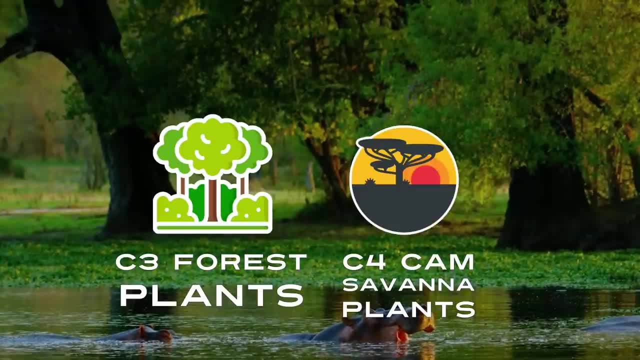 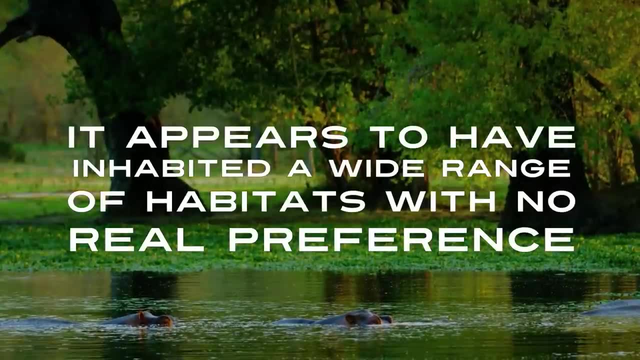 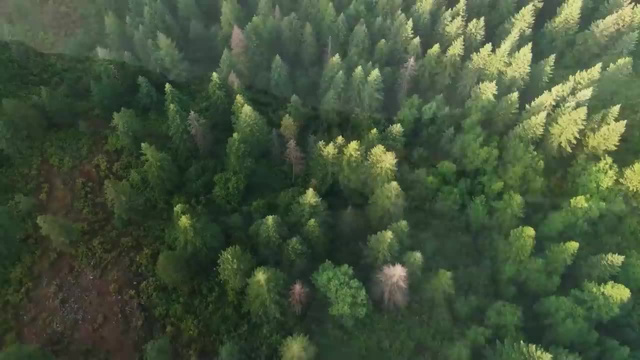 C-4, C a, m sabana plants, and were perhaps creatures which ate such plants and were able to exploit a variety of different food sources. Similarly, it appears to have inhabited a wide range of habitats with no real preference dwelling on open grasslands or woodlands. 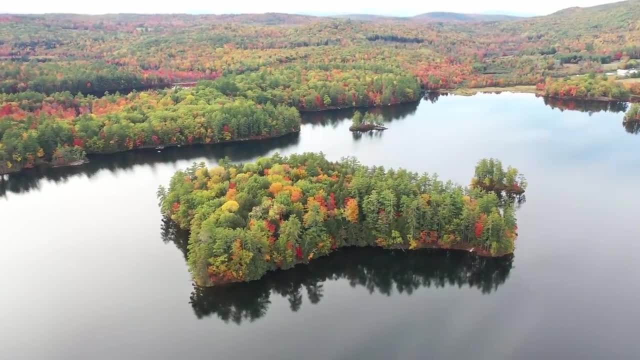 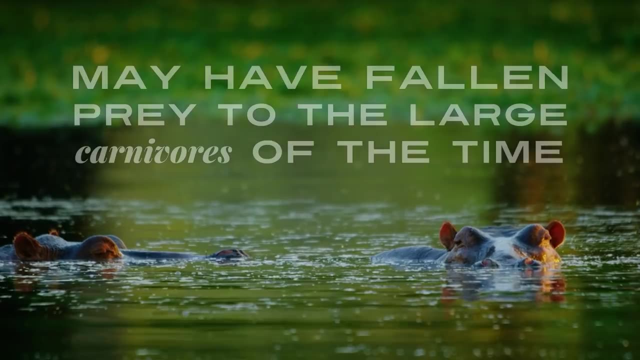 shrublands and lake or riverside forests. Potential evidence of stone tool use would indicate meat was also used to create these shells. This means that the antler of this also a dietary component. This group of early hominins may have fallen prey to the large. 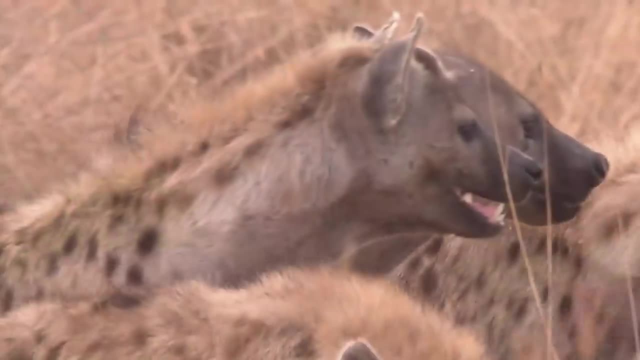 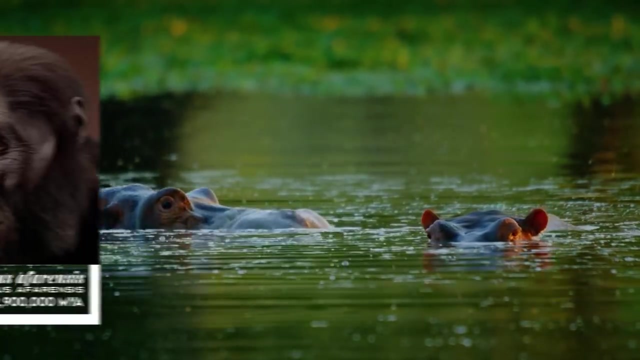 carnivores of the time, like big cats and hyenas. Luckily, over the years, researchers have unearthed more than 400 specimens attributed to the species Australopithecus afarensis from sites in Ethiopia, Kenya and Tanzania. 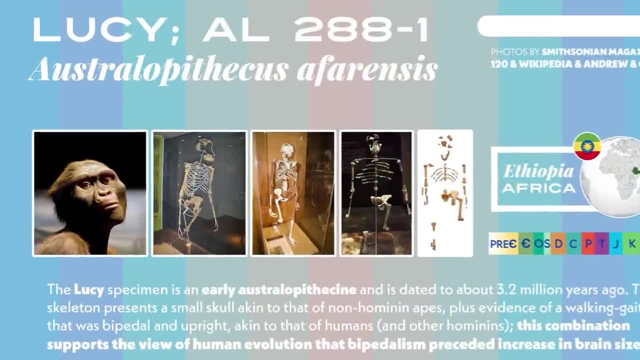 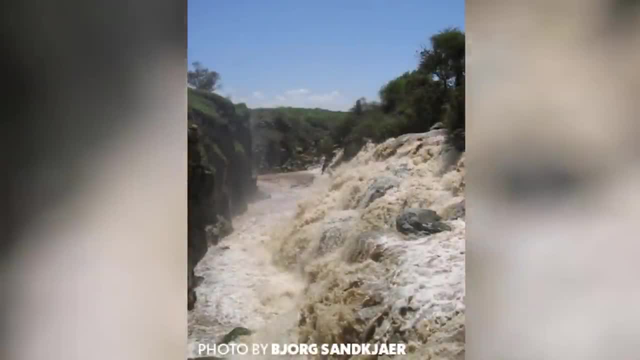 Lucy was a 40% complete skeleton of a female Australopithecus afarensis discovered in 1974 in Hadar, a site in the Awash Valley of the Afar Triangle in Ethiopia, by palaeoanthropologist Donald Johanson of the Cleveland Museum of Natural History. 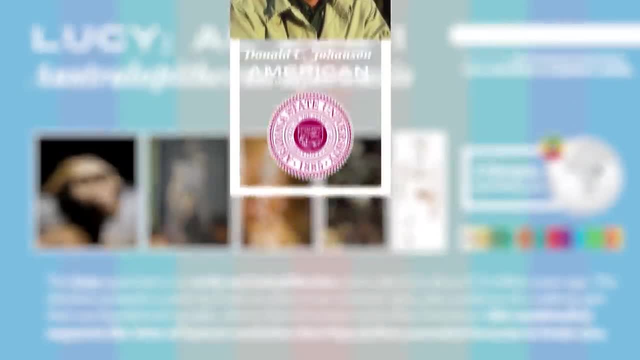 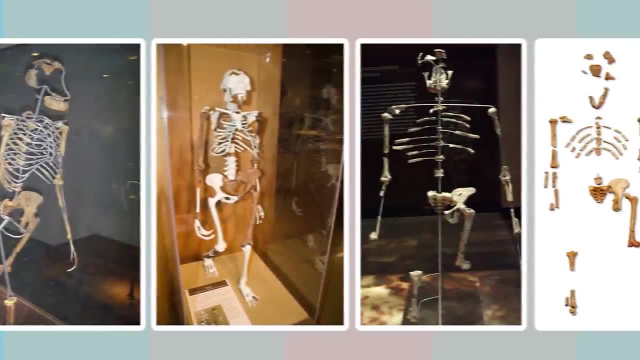 The Lucy specimen is an early Australopithecine dated to about 3.2 million years ago. The skeleton presents a small skull akin to that of non-hominin apes, with evidence of a walking gait that was bipedal and upright, akin to that of humans and other hominins. 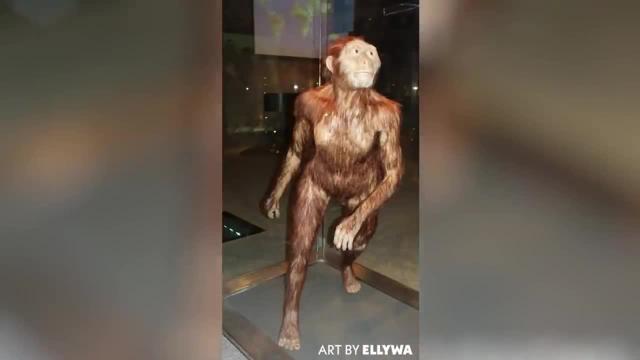 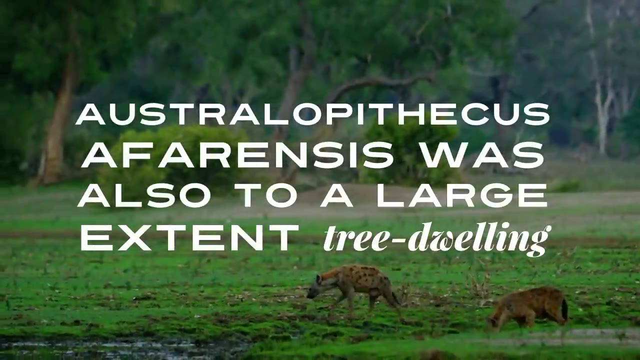 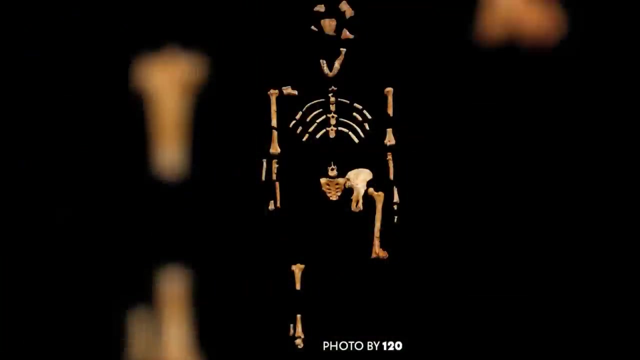 This combination supports the view of human evolution that bipedalism preceded increase in brain size. A 2016 study proposes that Australopithecus afarensis was also, to a large extent, tree dwelling, though the extent of this is debated. Lucy acquired her name from the 1967 song. 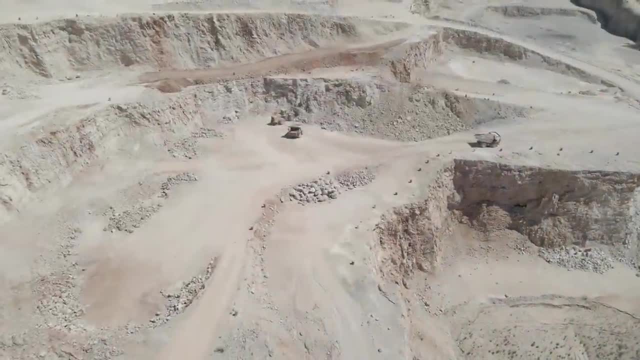 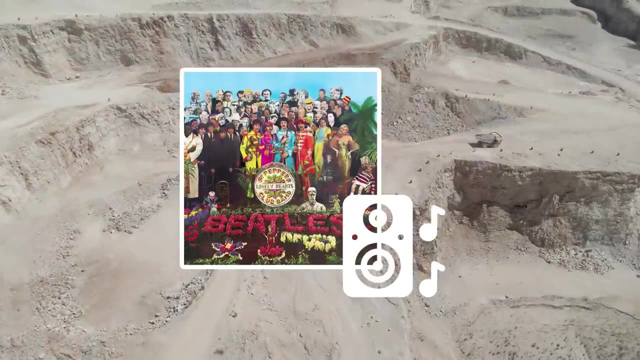 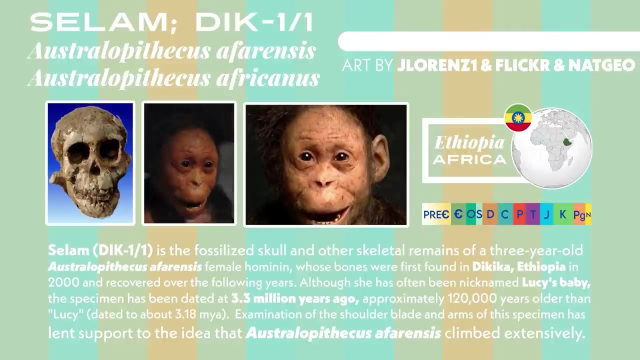 Lucy in the Sky with Diamonds by The Beatles, which was played loudly and repeatedly in the expedition camp all evening after the excavation team's first day of work on the recovery site. A aprove of a slopster Opening slightly further up: sap a feat. 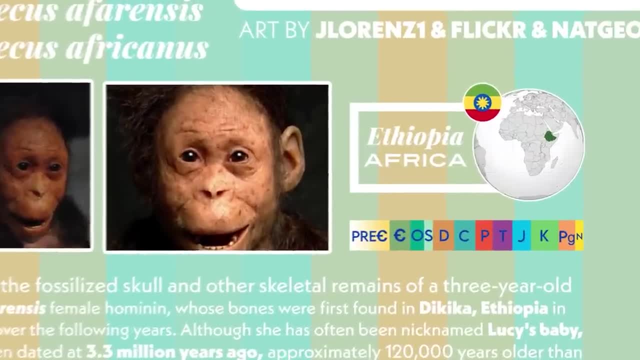 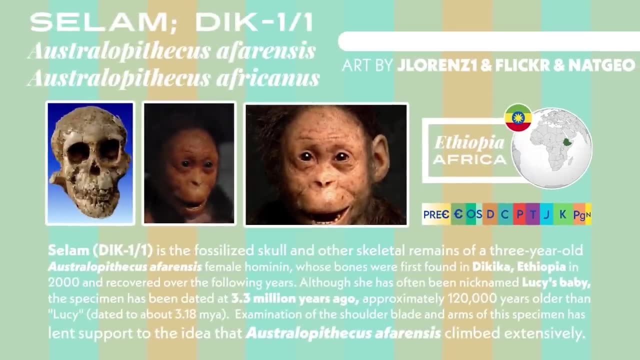 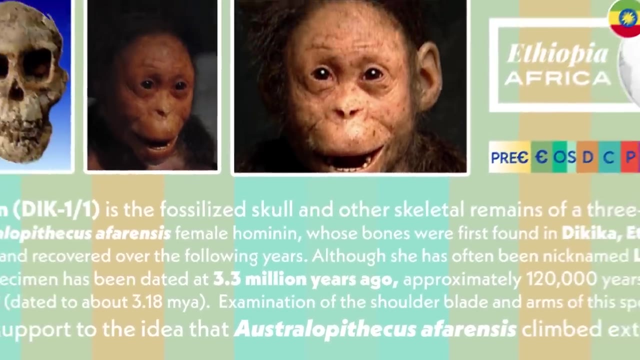 A hypothetical della salam Salaam includes the remains of a three-year-old Australopithecus afarensis female discovered in Dikika, Ethiopia, in the year 2000 and recovered over the following years, Although she has often. been nicknamed Lucy's Baby. the specimen has been dated to 3.3 million years ago — approximately 120,000 years older than Lucy, dated to about 3.18 million years ago. Examination of the short spine is shown clearly, reading thepack equal to the length of Lucy's neck. This includes a snake tonguebed Foreign. as primarily co delightful mirrors. The piece emits the zygomatic eak-erves and red venicle or Eaur jestece pike — the wear of the cornea and spines. The spines are not pulled off due to topателей of growth on their 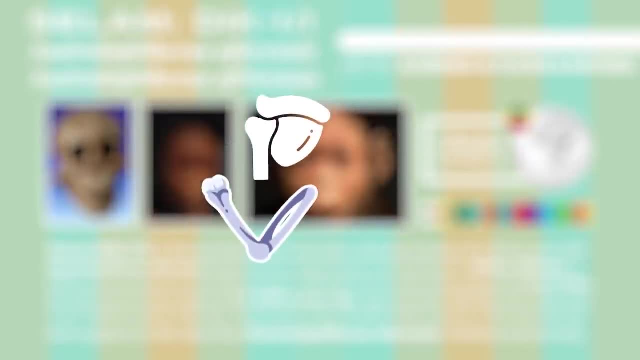 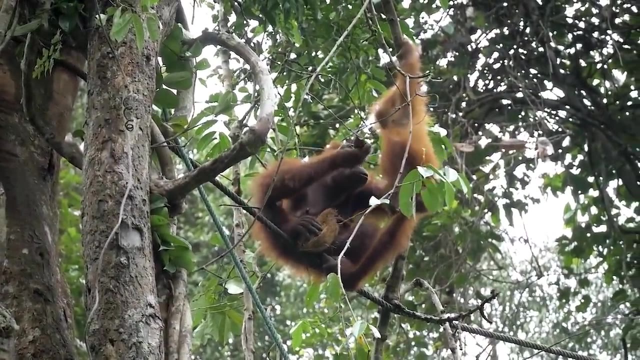 of the shoulder, blade and arms of this specimen has lent support to the idea that Australopithecus afarensis climbed extensively, evidence of arboreal behavior. Many paleoanthropologists propose that the Homo line derives from Australopithecus africanus. 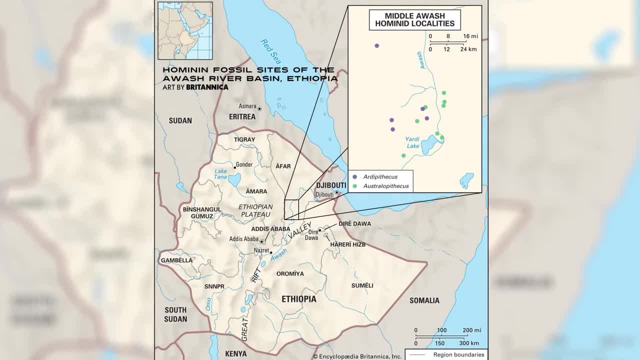 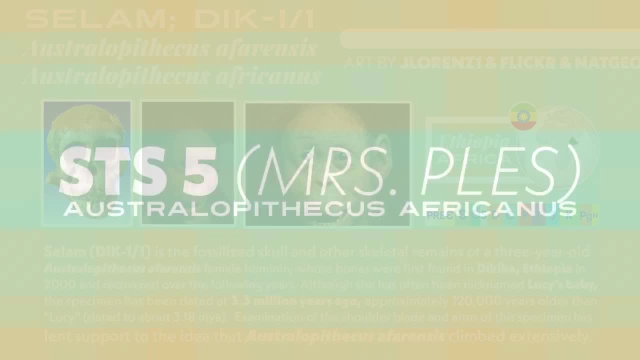 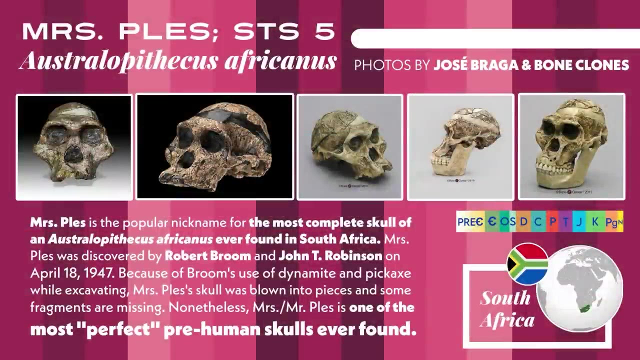 In this view, it might be better to place Salam in the Australopithecus africanus line, since it has more human-like traits than most Australopithecus afarensis. SDS 5,, or Mrs Pless, is the most complete skull of an Australopithecus africanus ever. 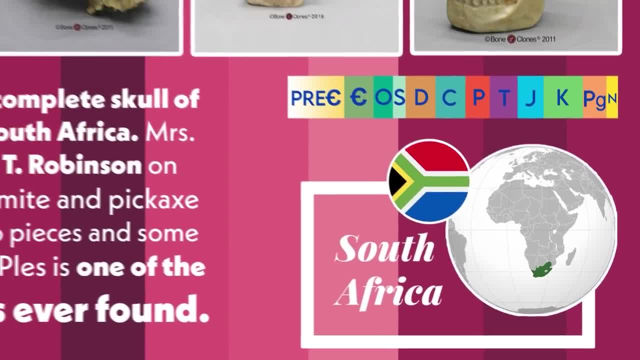 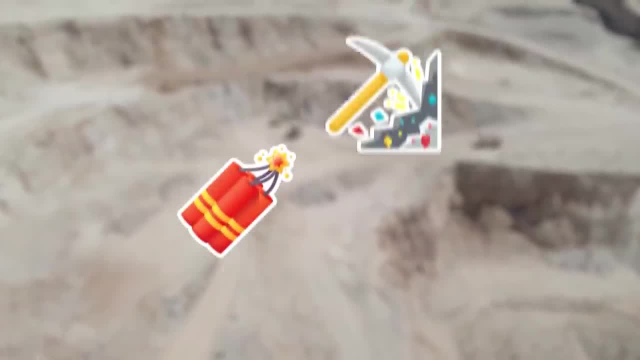 found in South Africa. Mrs Pless was discovered by Robert Broome and John T Robinson on April 18, 1947.. Because of Broome's use of dynamite and pickaxe while excavating, Mrs Pless's skull was. 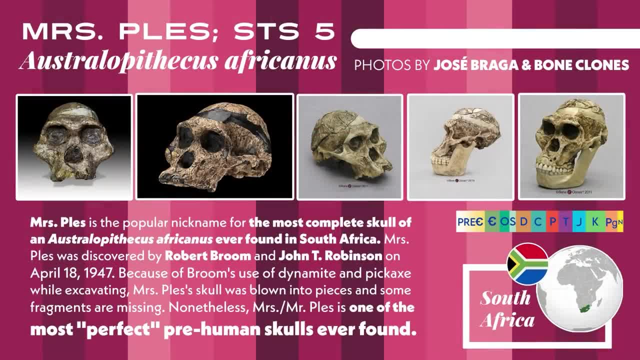 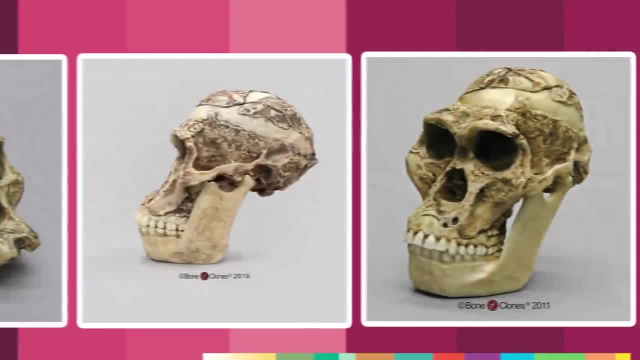 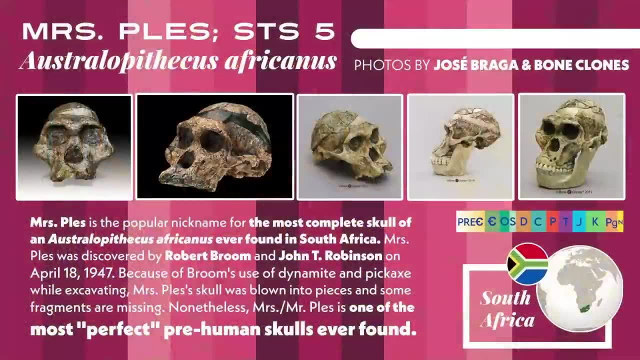 unfortunately blown into pieces and some fragments are missing. Nonetheless, Mrs Pless is one of the most perfect pre-human skulls ever discovered. The genus Australopithecus, of which there are several species, is considered the likely precursor of the genus Homo, to which all humanity belongs. 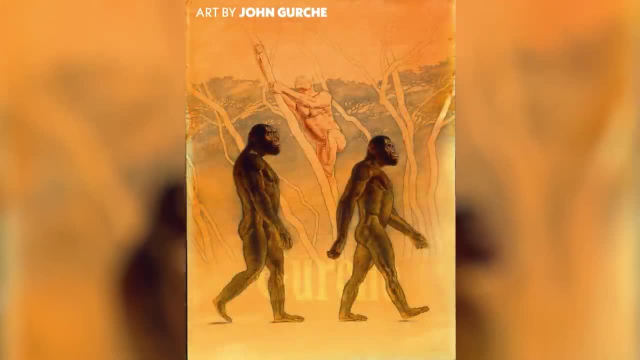 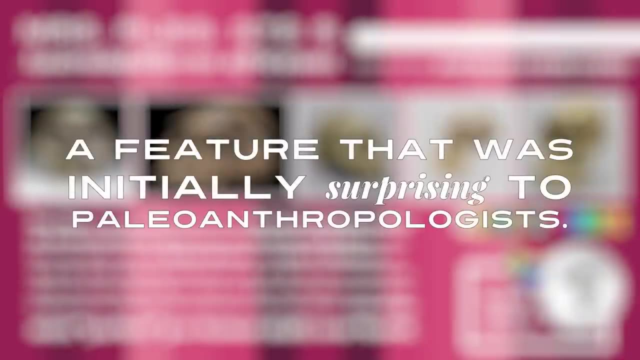 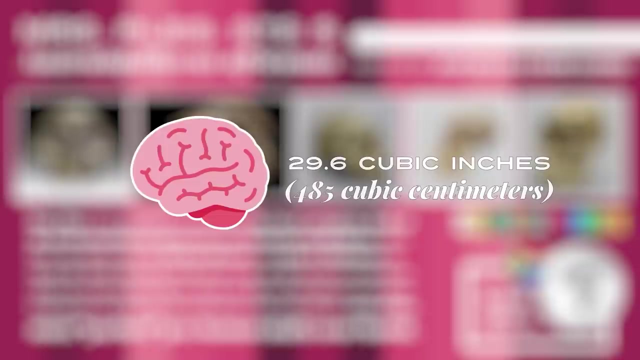 Though its cranium is comparable to a chimpanzee's, Australopithecus walked upright, as humans do, a feature that was initially surprising to paleoanthropologists. The cranial capacity of Mrs Pless is only about 29.6 cubic inches, or 485 cubic centimeters. 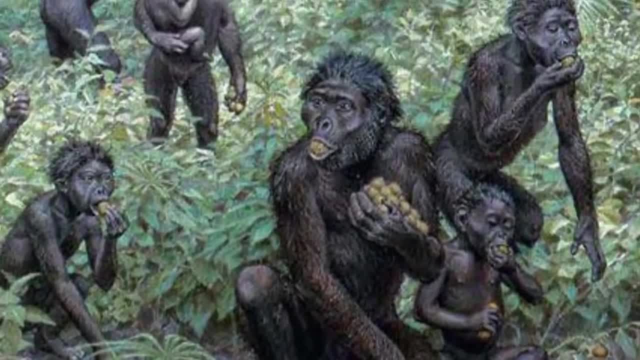 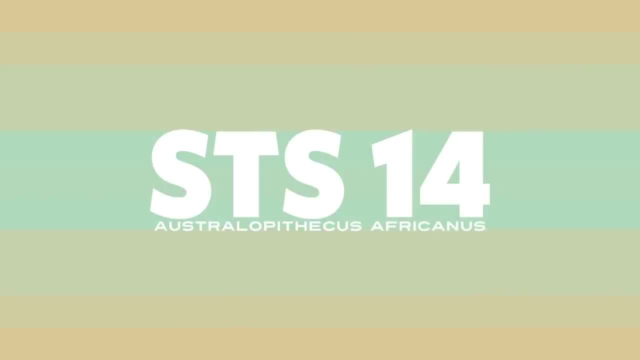 and was one of the first fossils to reveal the size of a human skull. It is believed that upright walking had evolved well before any significant growth in brain size. SDS-14- SDS-14 includes remains of an Australopithecus africanus discovered by Robert Broome and. 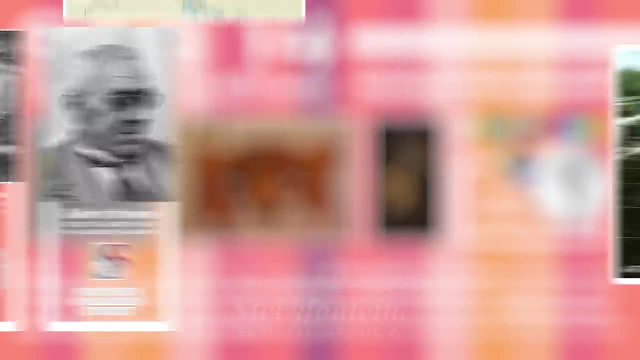 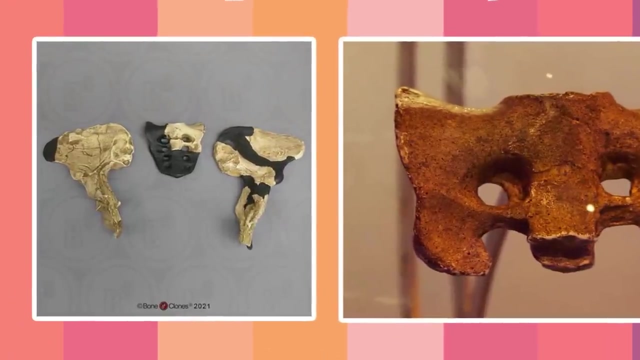 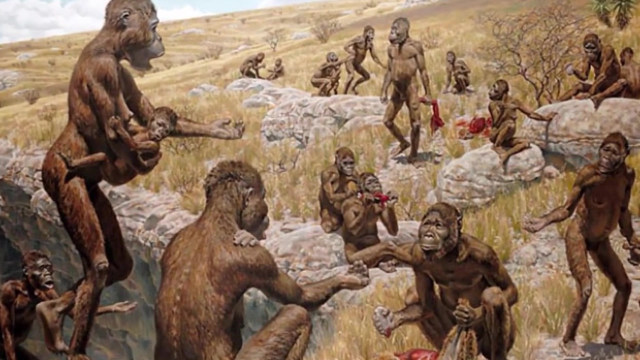 John T Robinson in August 1947 in Sterkfontein, South Africa. Estimated to be about 2.5 million years old, this specimen consists of a pelvis, vertebral column and fragmentary rib and femur. Notable traits include the distinctly human-like shape of its pelvic blades, indicating a type 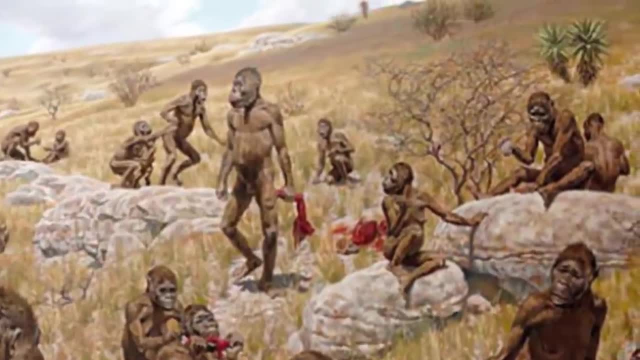 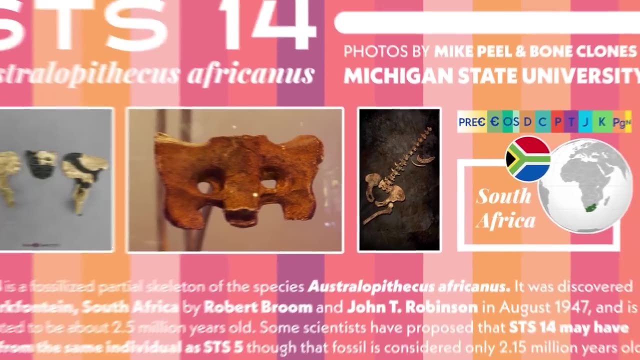 of bipedalism. This find was the first to demonstrate, without a doubt, pre-homo bipedality. Curiously, the specimen has six lumbar vertebrae, more than either most humans, who have five, or modern apes, which may have five or fewer. 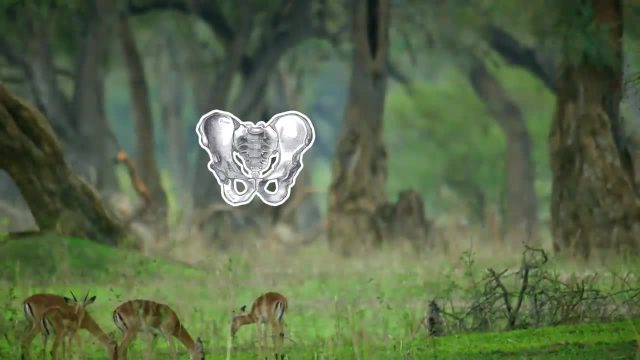 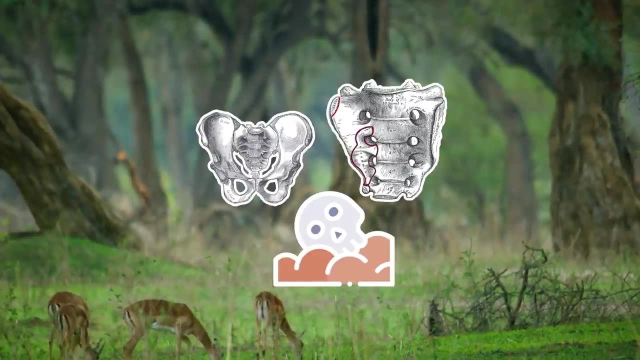 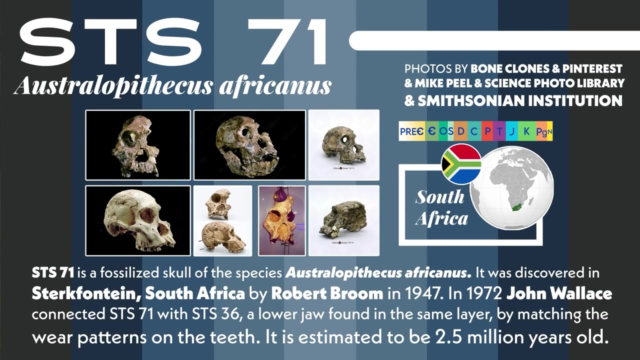 The specimen's sacrum contains an infused invertebral disc between the first and second sacral vertebrae, suggesting that the individual died before reaching maturity. SDS-71. SDS-71 includes the skull of an Australopithecus africanus discovered in 1947 in Sterkfontein. 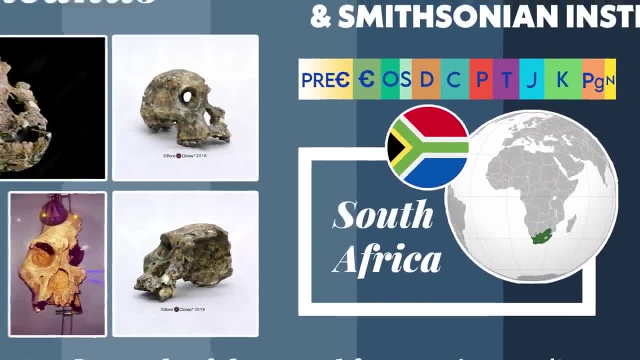 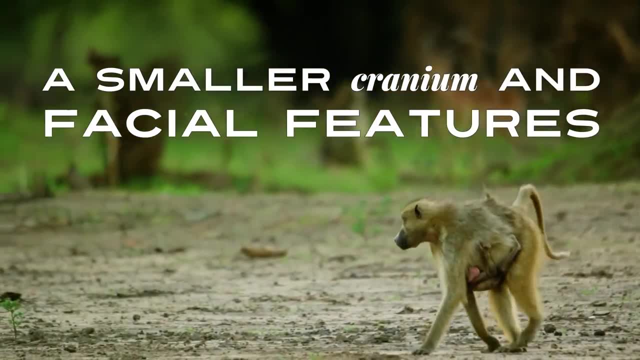 South Africa by Robert Broome. It is estimated to be 2.5 million years old. Its traits include a smaller cranium and facial features than other female Australopithecine finds, yet the size of the teeth indicate this specimen to be male. 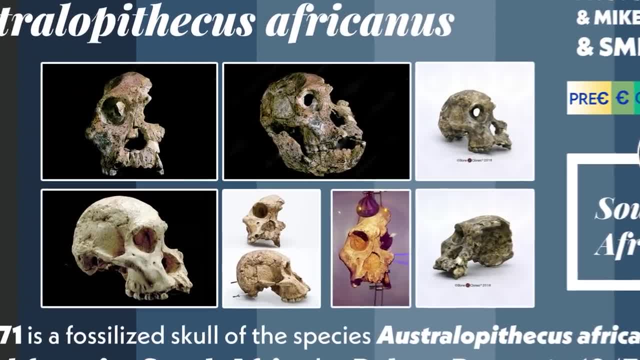 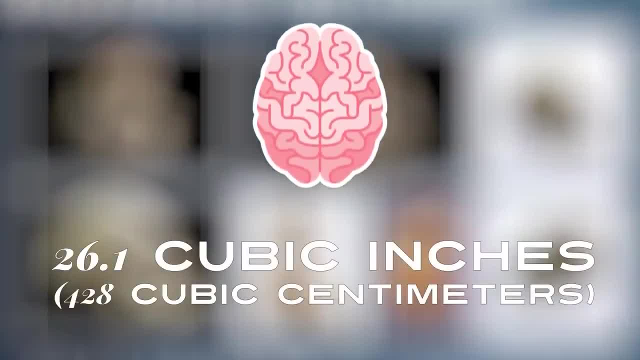 The face shows forward-looking teeth. The face shows forward-looking teeth. The upper projection and the position of the temporal glands high on the cranium indicate large chewing muscles. The brain is 26.1 cubic inches or 428 cubic centimeters. 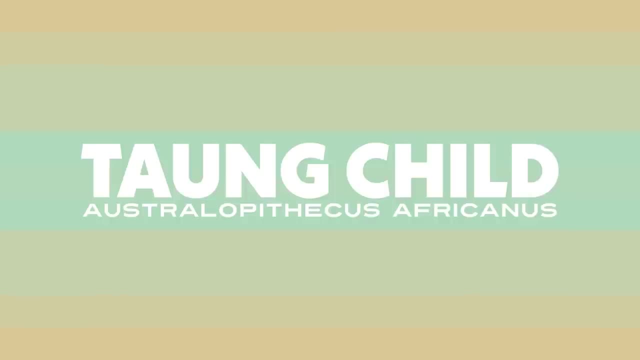 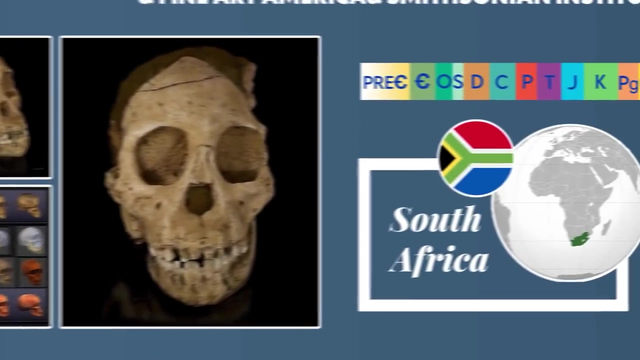 SDS-71. The Tong child includes the skull of a young Australopithecus africanus discovered in 1924 by quarrymen working for the Northern Lime Company in Tong, South Africa. Raymond Dart described it as a new species in the world. 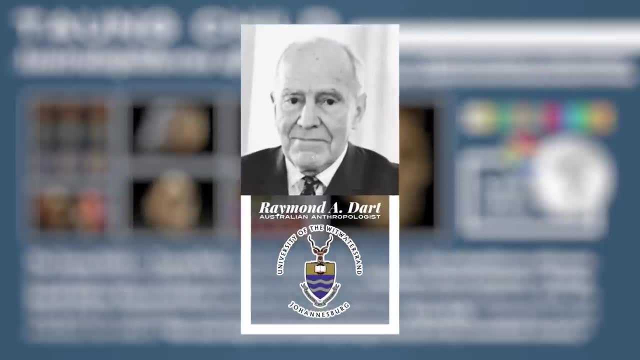 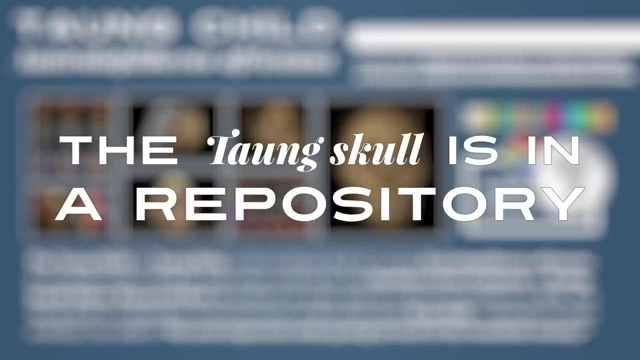 It was a new species in the journal Nature in 1925. It was from 2.8 million years ago and it was 3.3 years when it died. The Tong skull is in a repository at the University of Woodwater's rent. 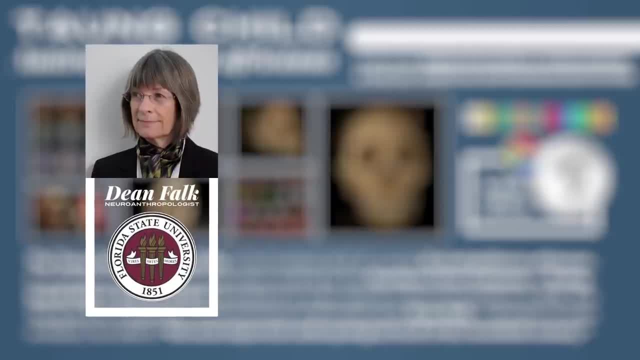 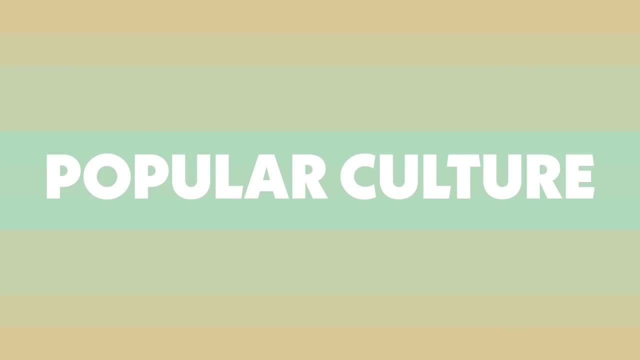 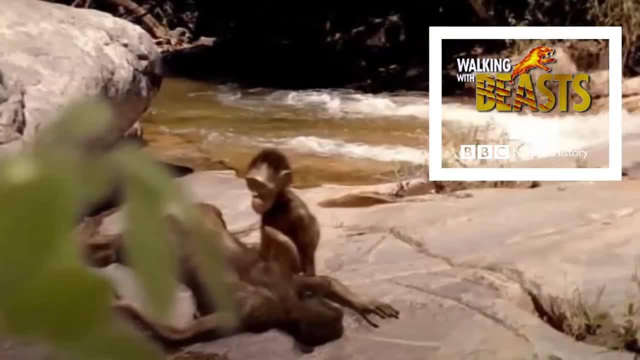 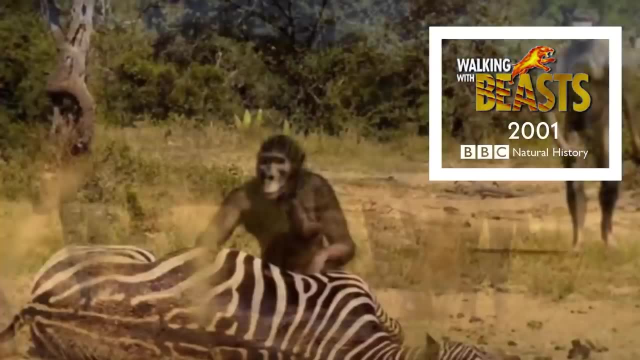 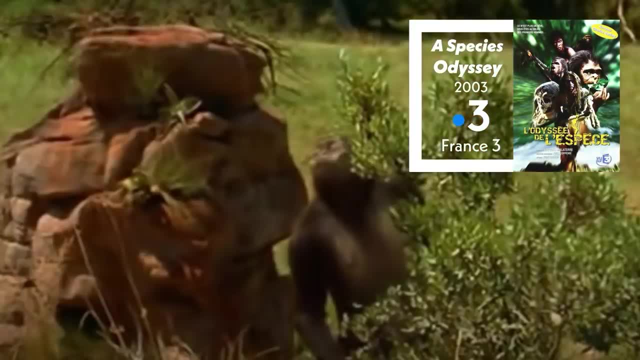 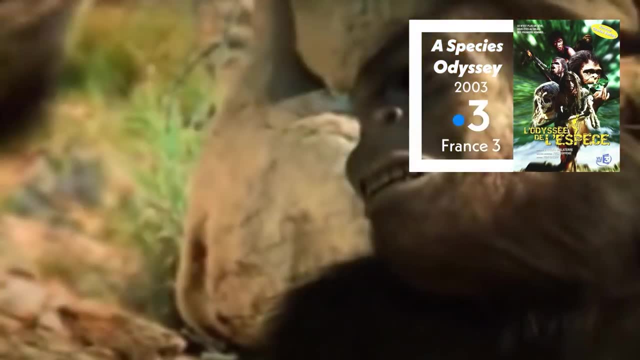 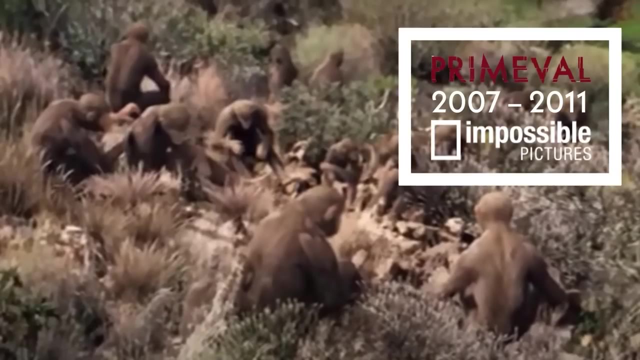 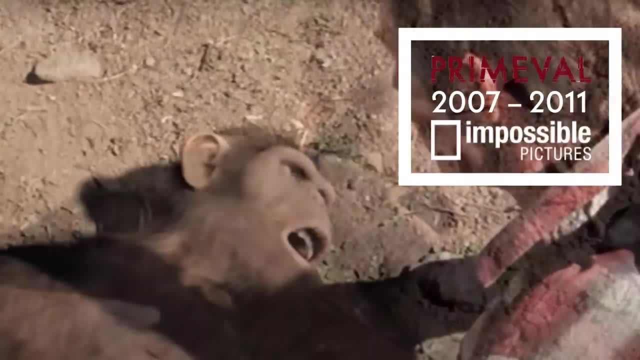 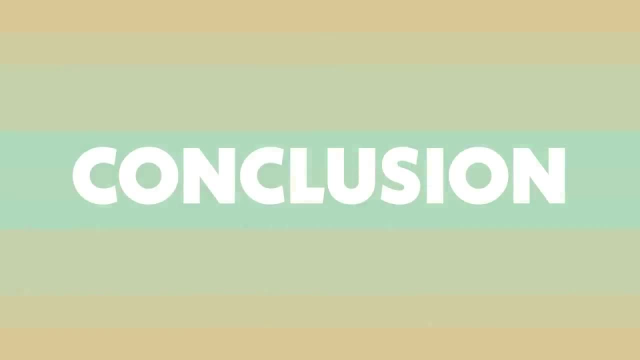 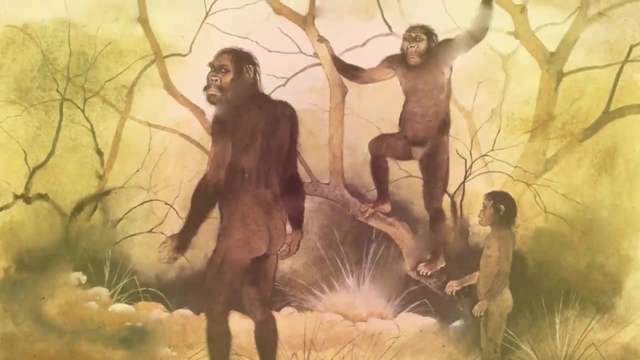 than they are in actuality, and killed by poisoning by a human. yet a large group is then found to be alive and thriving. Early hominins that dwell in numerous areas throughout Africa existed during the early Pliocene and early Pleistocene. 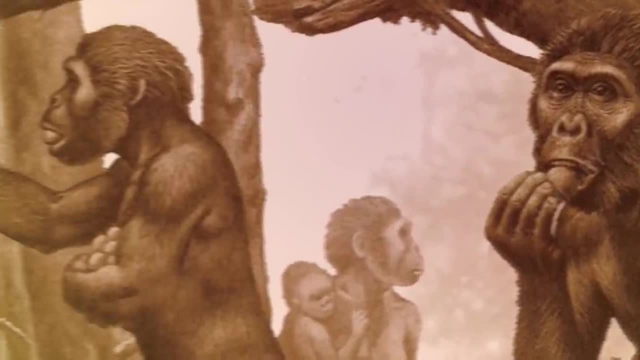 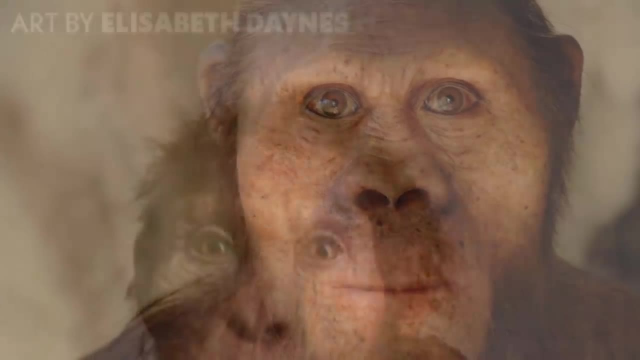 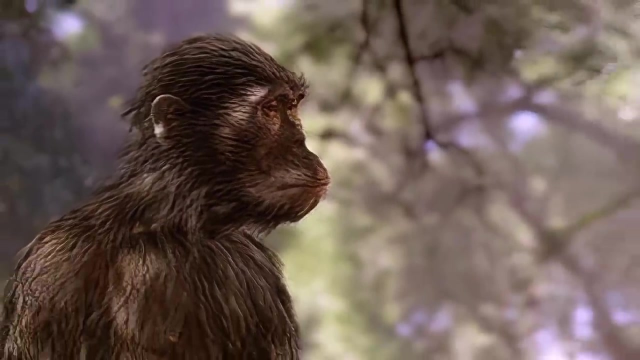 This group is thought to have been the ancestor to Homo, a group including other hominins. in modern humans, There is a diverse plethora of species in the genus and controversy surrounding the synonymy of certain taxa. The earliest member of Australopithecus dwelt around 4.2 million years ago and eventually 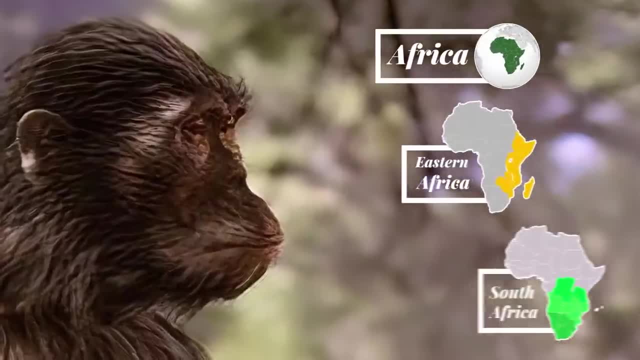 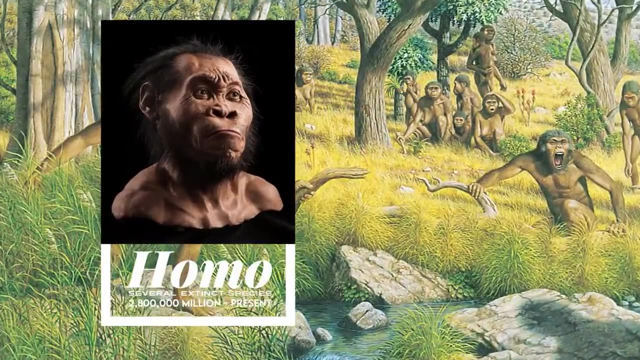 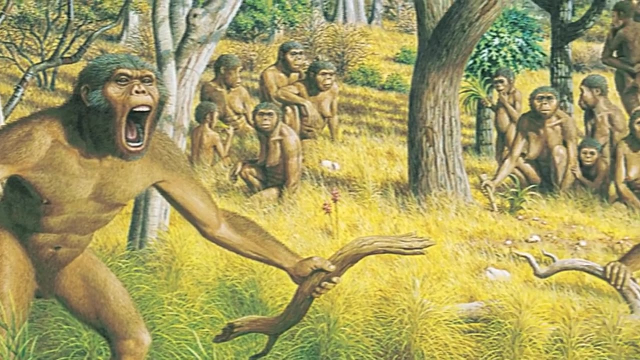 became widespread throughout eastern and southern Africa, becoming extinct 1.9 or 1.9 million years ago. The genus Homo arose from an Australopithecus species between 3 and 2 million years ago, Bipedal packing small brains and smaller canine teeth than apes their cheek teeth. 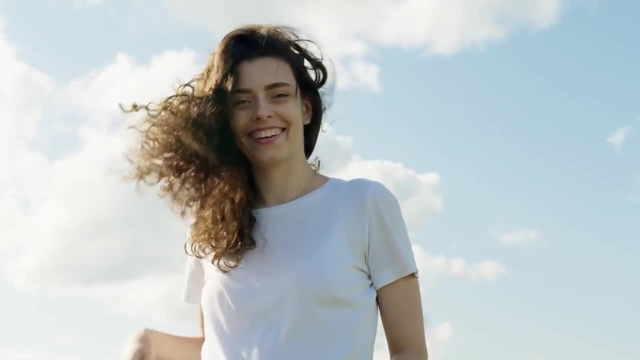 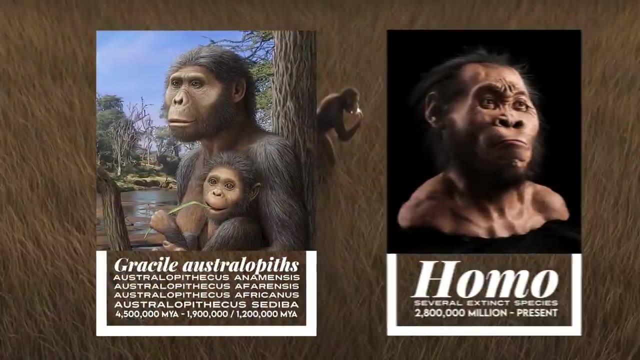 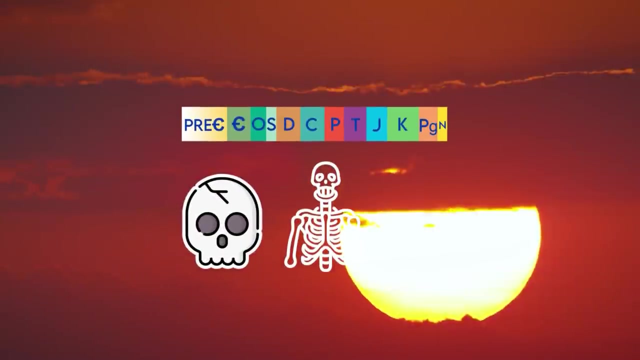 were surprisingly larger than those of modern humans. Researchers agree that one of the grasshopper species, or a yet undiscovered variety, was the direct ancestor of the genus Homo and, ultimately, living humans. However. 2. The period in which the fossils were discovered is too ancient for African fossil DNA to survive. 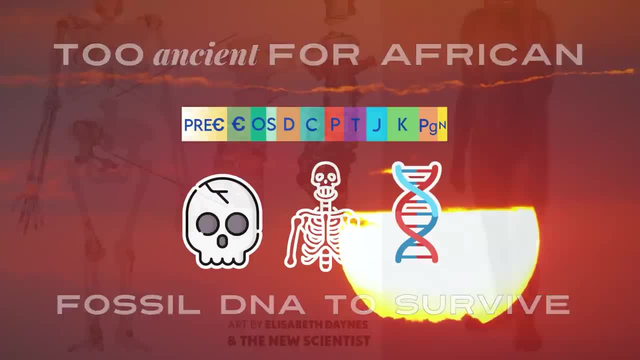 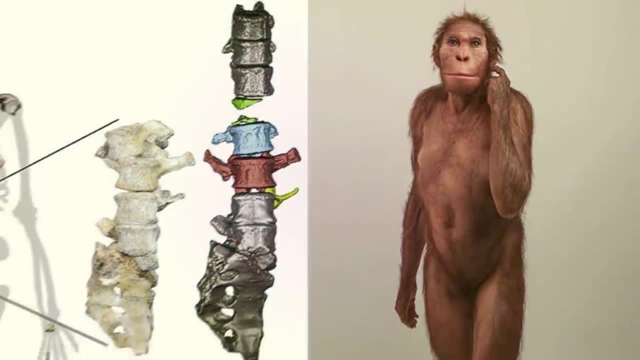 Anthropologists must reconstruct the Australopithe family tree based on visible skeletal traits, leaving more room for ambiguity and interpretation. Looking back millions of years to the age of Australopithes, no one would have expected for this hominin lineage to thrive. 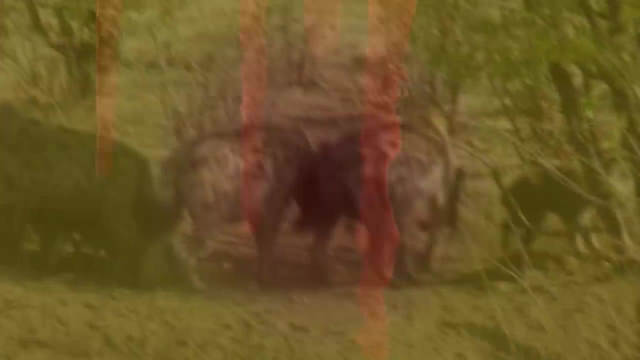 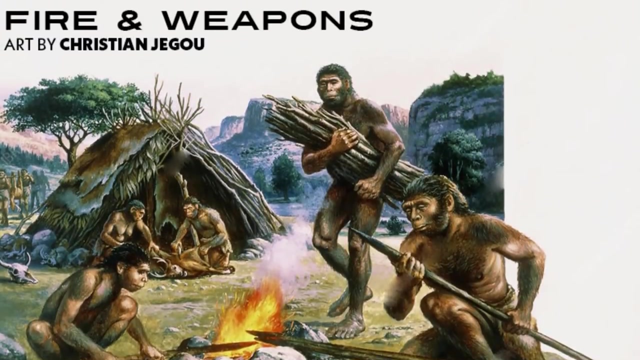 They were short and slow and probably made prime targets for predators. They lacked advantages of later hominins, Big brains, advanced weapons and fire, as well as defenses of earlier, more ape-like ancestors, including large canine teeth and tree-climbing abilities. 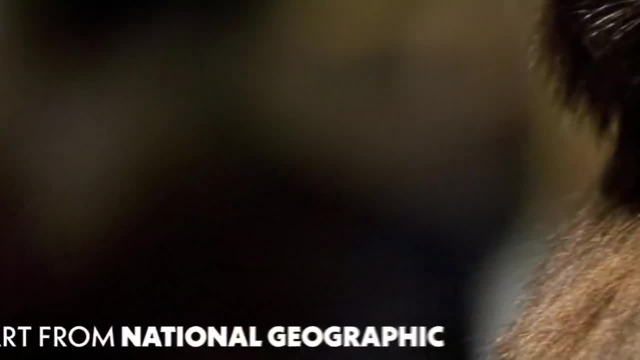 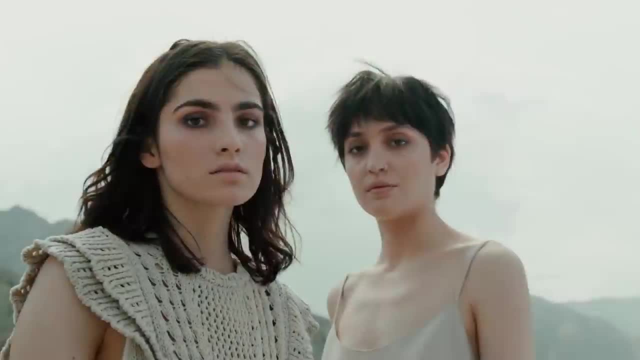 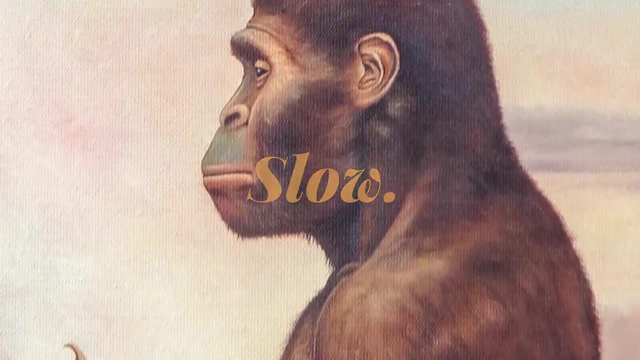 Nonetheless, during this period, hominins diversified into a multitude of species, and we Homo sapiens are here today due to the survival of one of those lineages: Australopithecus: Small, Slow, Diverse, Sexually dimorphic. 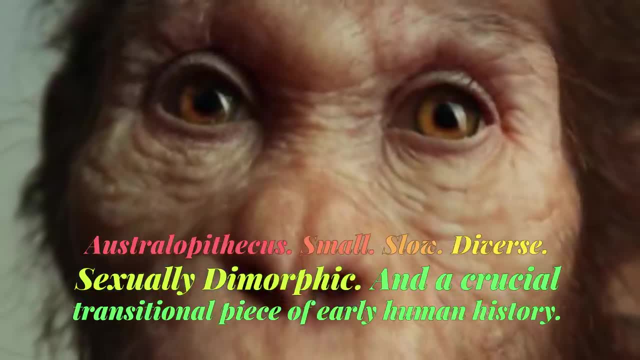 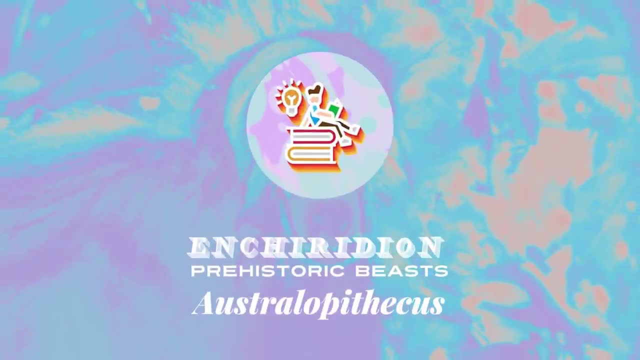 And a crucial transitional piece of early human history. Thank you so much for joining me in this program episode of Prehistoric Beasts. I listened to the feedback you guys included in the comments and removed the leaves covering the hominins in this redux version, which I hope was much less distracting.